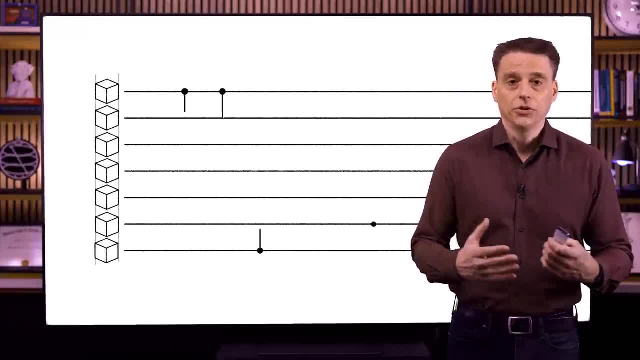 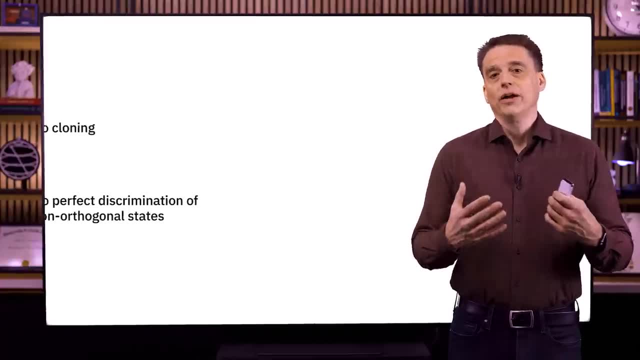 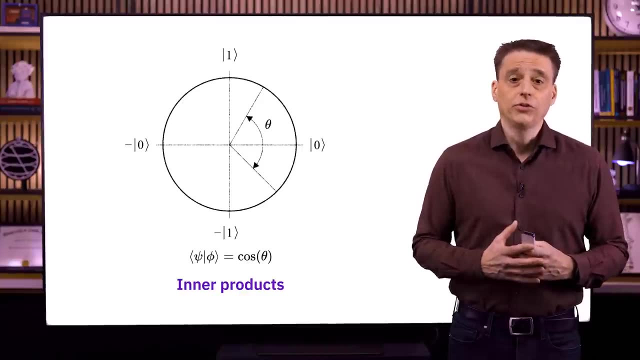 for both single and multiple systems. we've taken a look at the quantum circuit model and we've observed some fundamental limitations on quantum information. Along the way, we encountered some important mathematical concepts, including tensor products and inner products, and we'll continue to make use of those concepts and we'll introduce some. 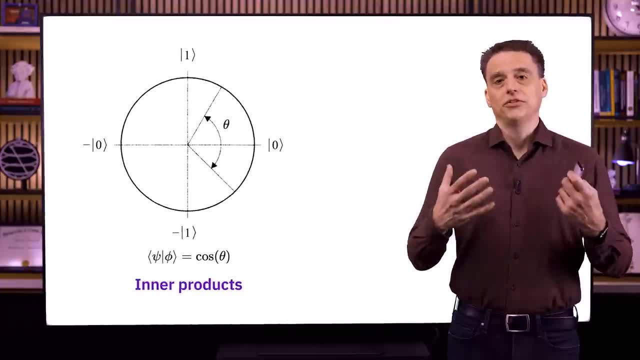 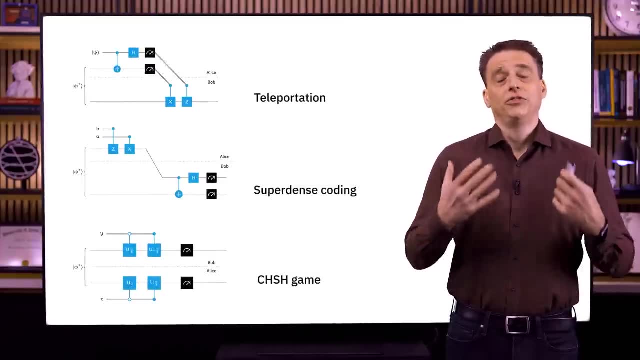 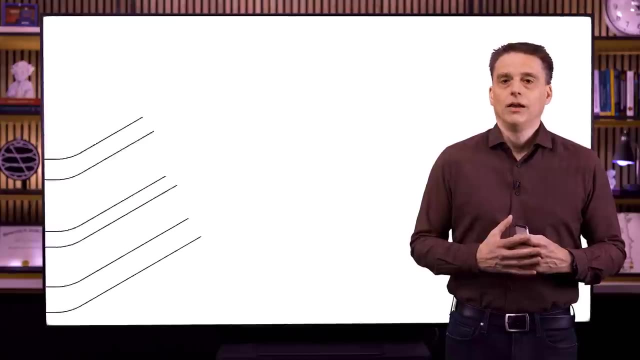 new ones as well as we need them. In this lesson, we'll be focusing on three fundamentally important examples: Quantum teleportation, super dense coding and the CHSH game, which is also called the CHSH inequality and not always described as a game. These are not just random examples meant. 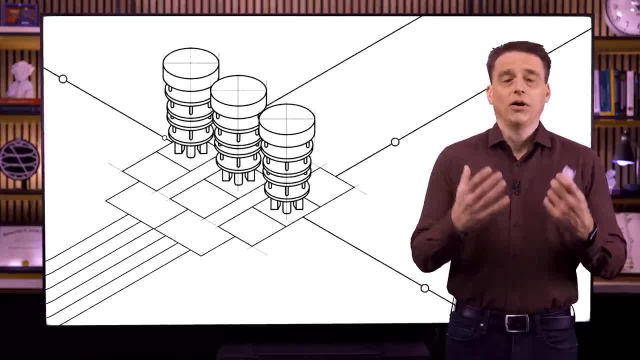 to illustrate how quantum information works. They're not just random examples meant to illustrate how quantum information works. They're not just random examples meant to illustrate how quantum information works. They're not just random examples meant to illustrate how quantum information works. They really are key parts of the foundation of 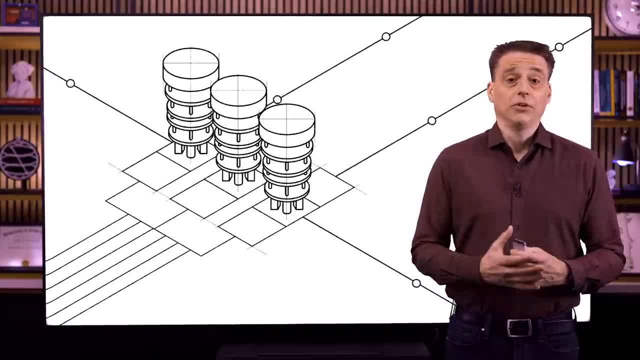 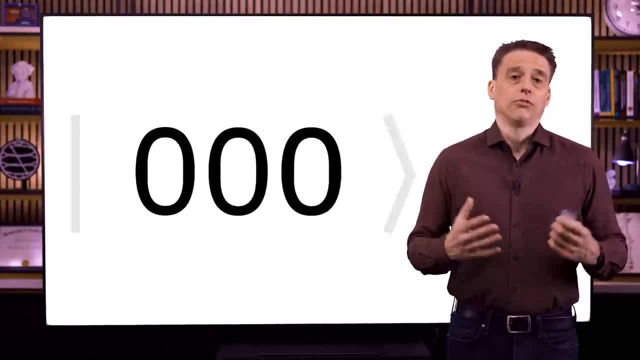 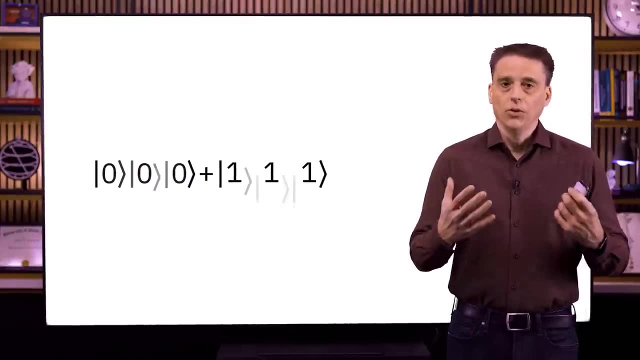 quantum information, and they arise in different and sometimes unexpected settings within quantum information and computation. Entanglement plays a key role in all three of these examples and in fact it's entanglement that makes them work and makes them interesting. So this lesson will in some sense be our first opportunity to see 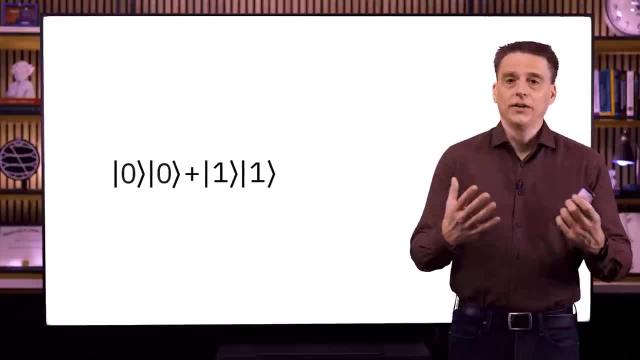 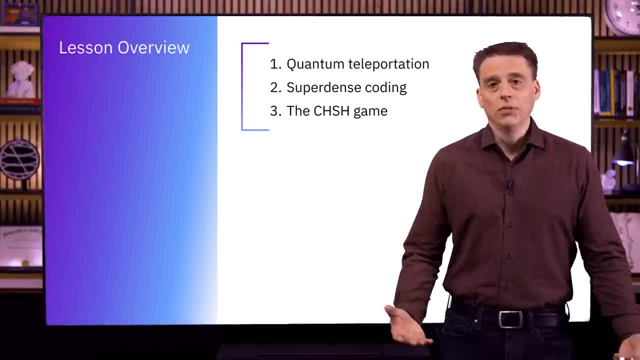 entanglement in action and to begin to explore what it is that makes entanglement so interesting. The overview for the lesson is very simple. We'll go one by one through the three examples that I just mentioned: Quantum teleportation, super dense coding and the CHSH. 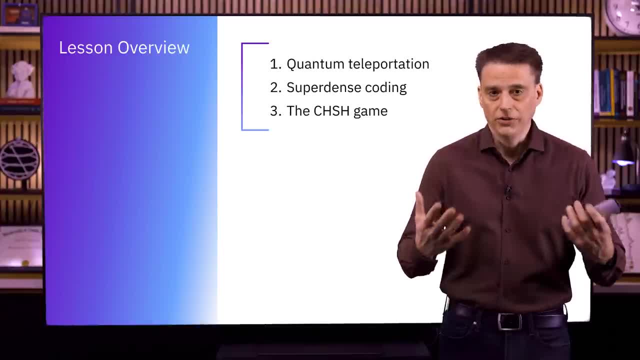 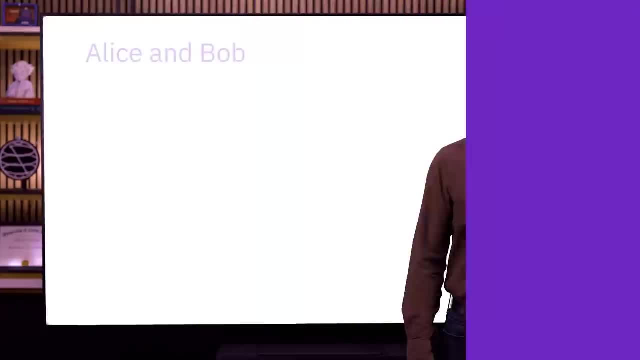 game. We'll discuss what these things are and what makes them interesting, and we'll go through analyses that explain exactly how they work at a mathematical level. Before we get to the first of the three examples, which is quantum teleportation, it's appropriate to first introduce the characters. 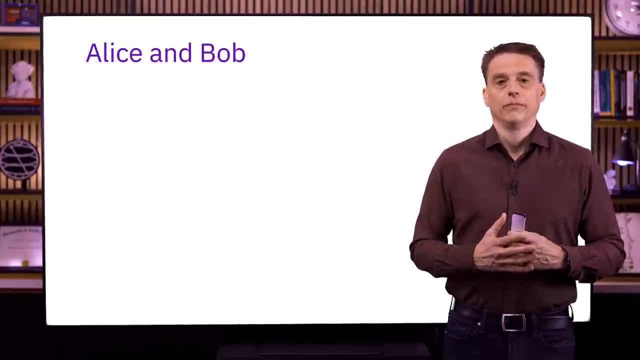 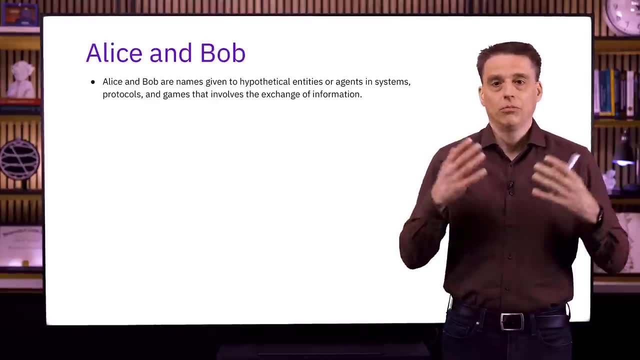 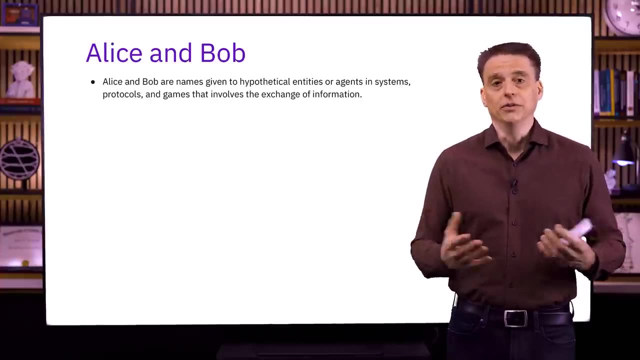 Alice and Bob. in case you're not familiar with them, Alice and Bob are names given to hypothetical entities or agents in systems, protocols, games and really any other type of interaction you might wish to consider that involves the exchange of information. They first arose in the context of cryptography in the 1970s, but the convention to use these 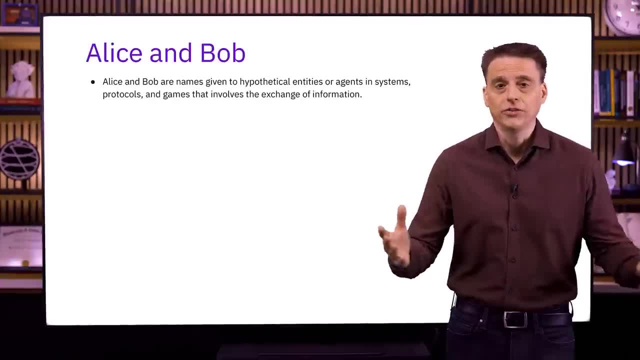 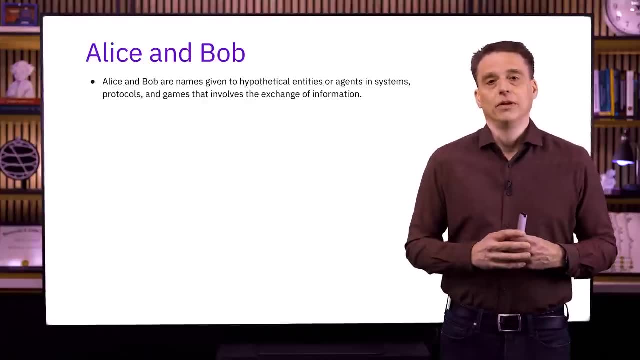 names in this way has become very common in a much broader context since then. The idea is that these are very common names, at least in some parts of the world, and they start with the letters A and B. It's also convenient to refer to Alice and Bob using the pronouns her and him. 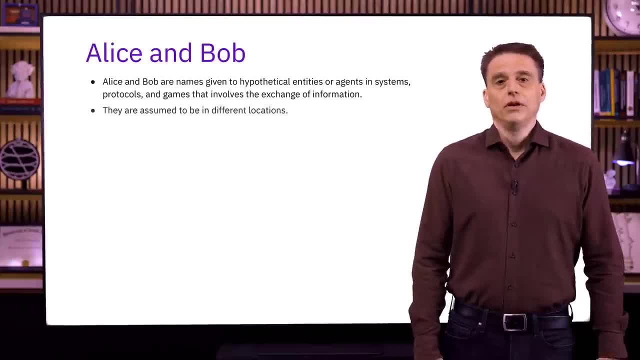 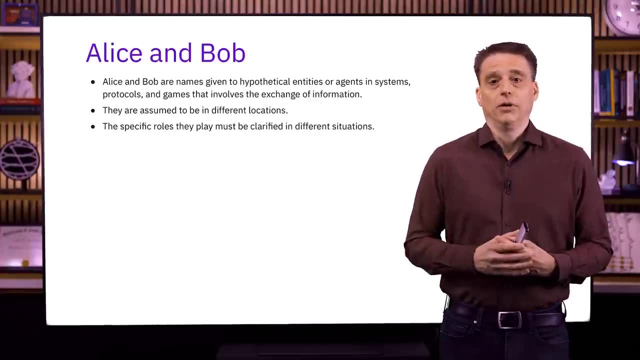 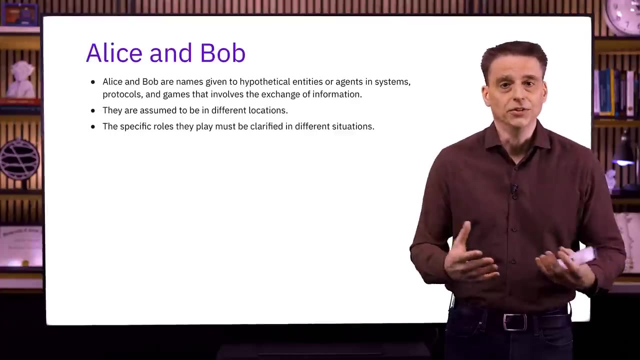 just for the sake of brevity, We typically imagine that Alice and Bob are in different locations and that they have different goals and different behaviors, depending upon whatever it is that we're talking about. For example, if we're talking about communication, meaning the transmission of information, then we might decide that Alice is the sender. 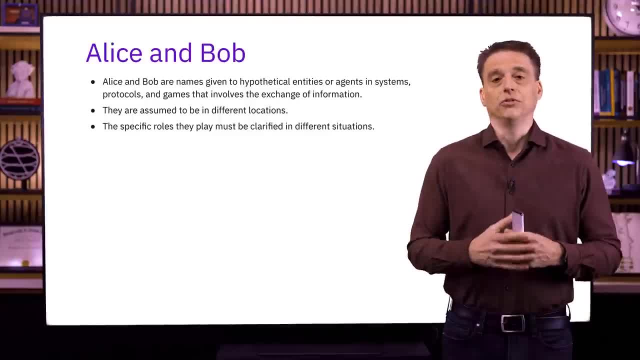 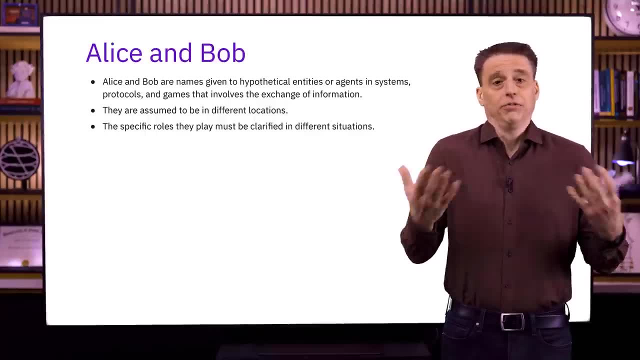 and Bob is the receiver of whatever information is being transmitted. Sometimes Alice and Bob cooperate- that's very typical- but sometimes they compete or they might have different goals. that may or may not be consistent with one another, But this all has to be made clear in the situation at hand. 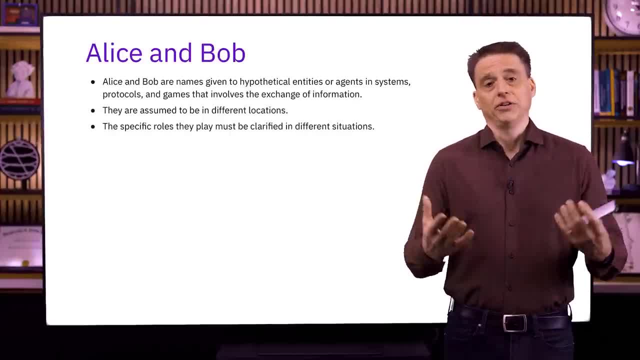 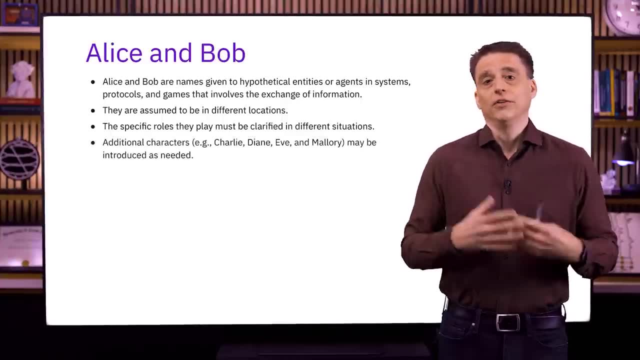 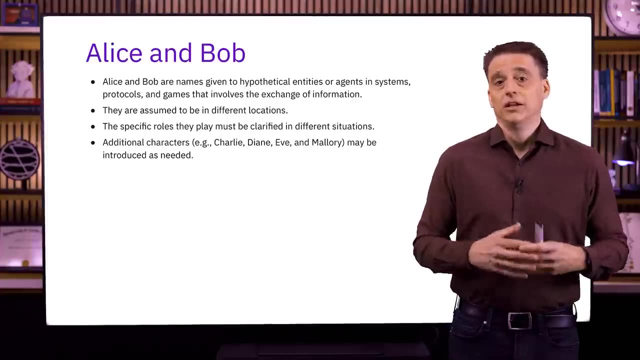 Of course, they represent abstractions and not necessarily actual human beings. We can also introduce additional characters, such as Charlie and Diane, or different names that represent different personas, such as Eve for an eavesdropper, or Mallory for someone behaving maliciously. 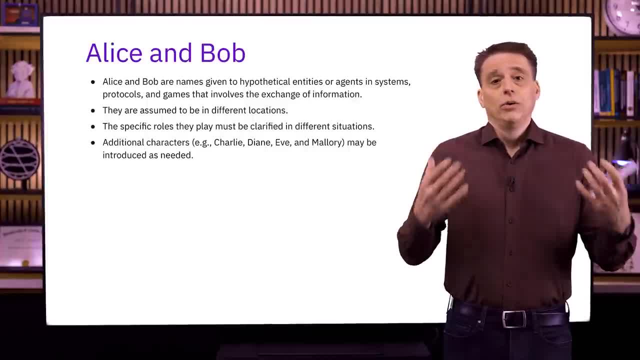 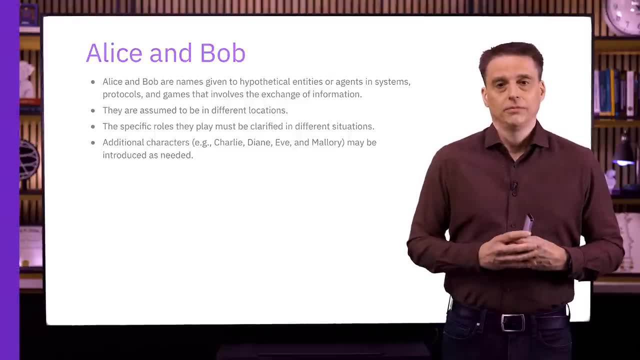 depending upon the setting. In any case, we will see Alice and Bob in all three of the examples that we'll discuss in this lesson and, from time to time, throughout the remainder of the series. I'll also make a few comments about entanglement before moving on to the three examples. 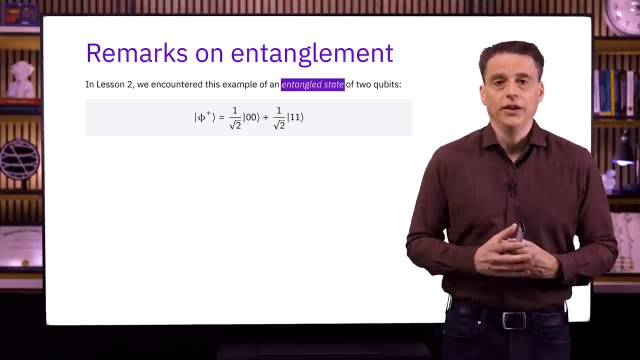 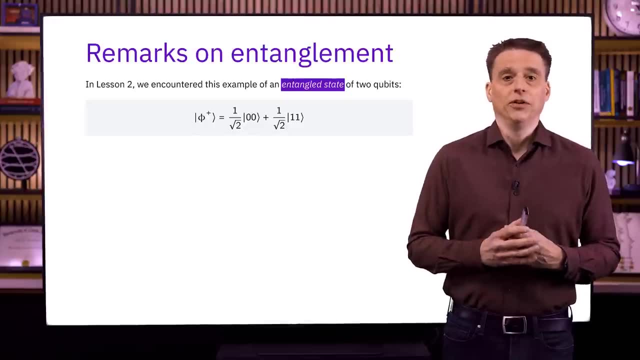 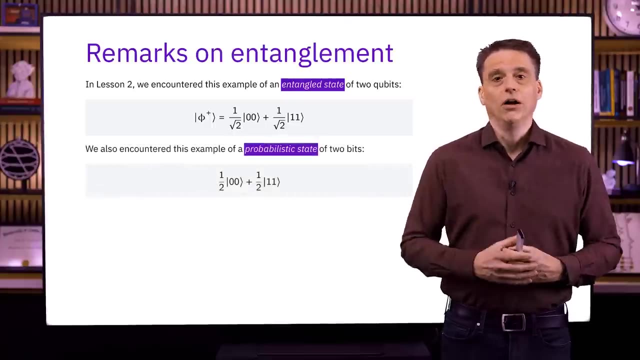 In lesson two, we encountered this example of an entangled state of two qubits. It's a one of the four Bell states and you could say that this particular state represents the archetypal example of an entangled quantum state. We also encountered this example of a probabilistic state of two bits. 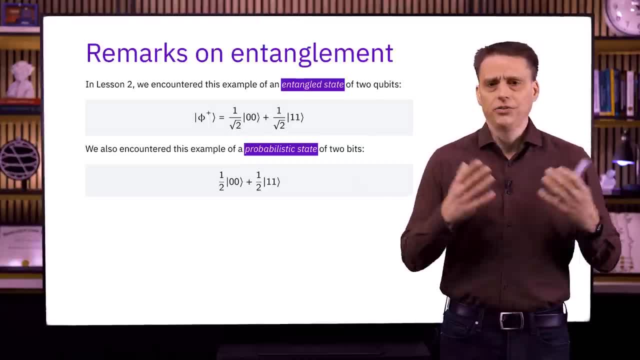 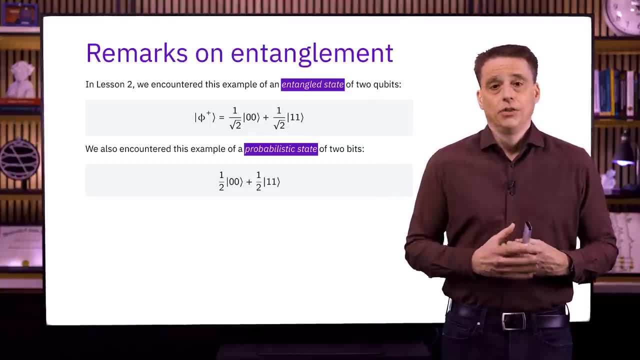 It's analogous to the entangled state in some sense, but it's not entangled. Entanglement is a uniquely quantum phenomenon, essentially by definition. There is a precise mathematical definition of what entanglement is and basically what entanglement is is that it's an entanglement of two qubits. It's an entanglement. 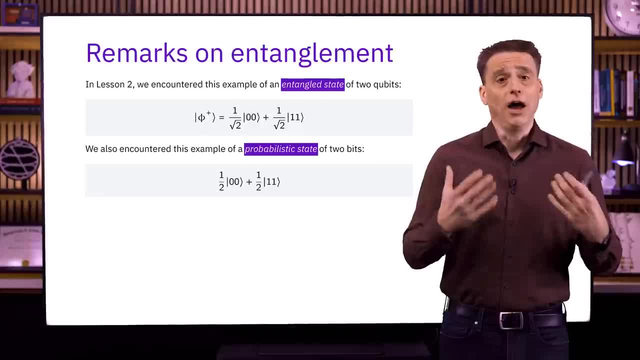 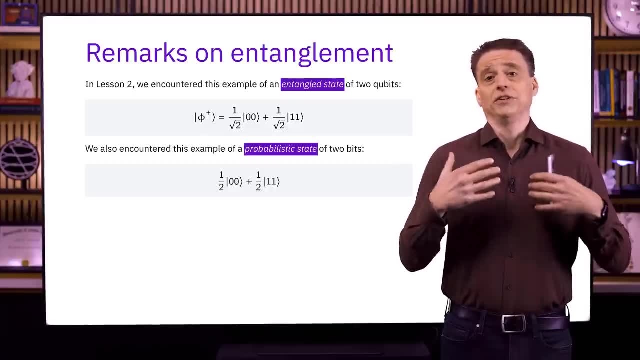 of two qubits. Basically, what that definition says is that entanglement is a non-classical quantum correlation, But that's not all that helpful at an intuitive level. It's a definition of entanglement in terms of what entanglement isn't, And it's probably for that reason that 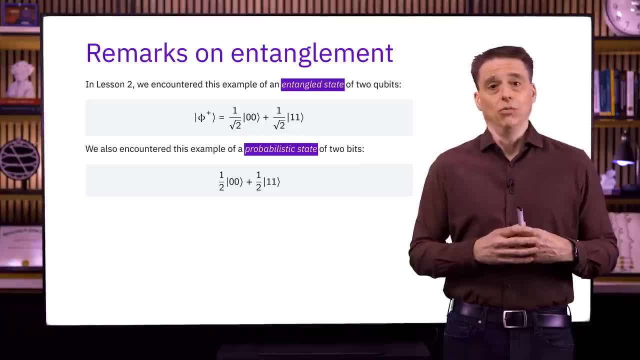 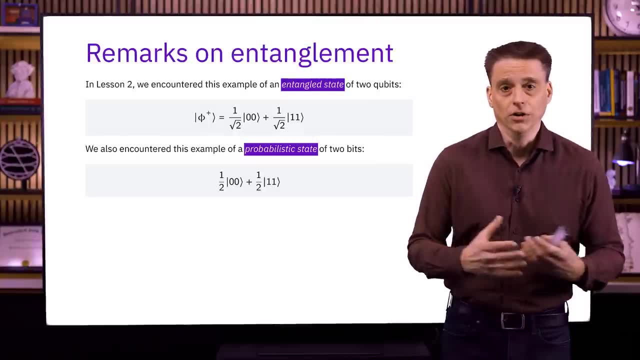 it's actually pretty difficult to explain what entanglement is and what makes it special in intuitive terms. When people do try to explain what entanglement is in intuitive terms, you often hear explanations that really don't distinguish these two states in a meaningful way. 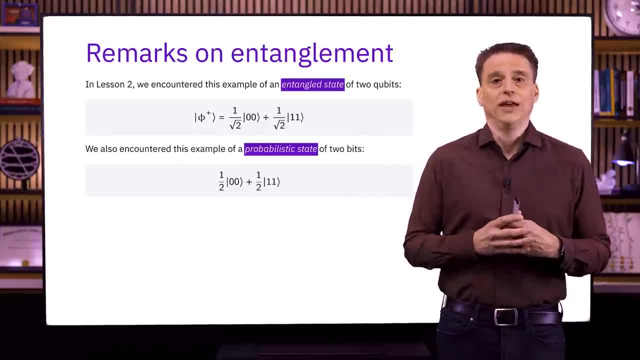 You may hear the idea that if you measure one of the two entangled qubits, then the state of the other one is somehow instantaneously affected, or that the state of the two qubits can't be described separately, or that the two qubits somehow maintain a memory of one another. 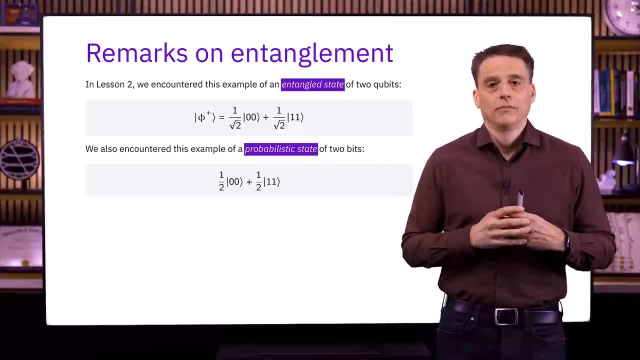 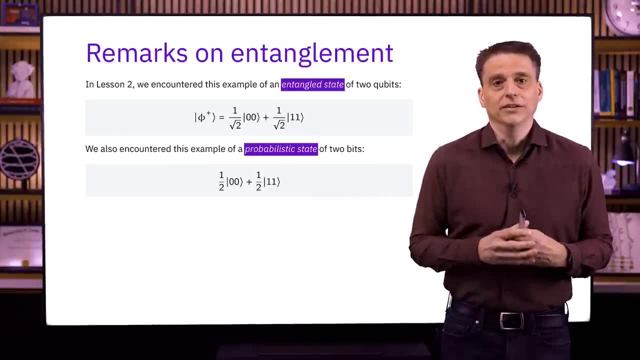 or even that they're emotionally attached in some way. But why are those properties not true for this state? These two bits are intimately connected and each one has a perfect memory of the other one, in a literal sense, But it's not an entangled. 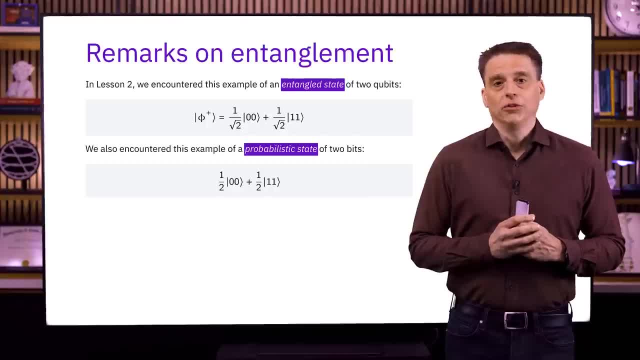 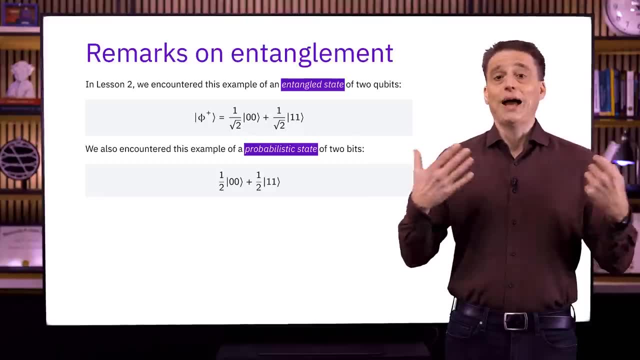 state. Well, one way to explain what makes entanglement special and what makes this state very different from this state is to explain what we can do with entanglement or what we can see happening because of entanglement that goes beyond the decisions we make about. 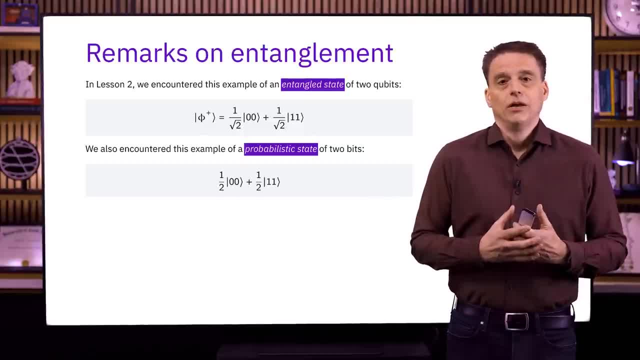 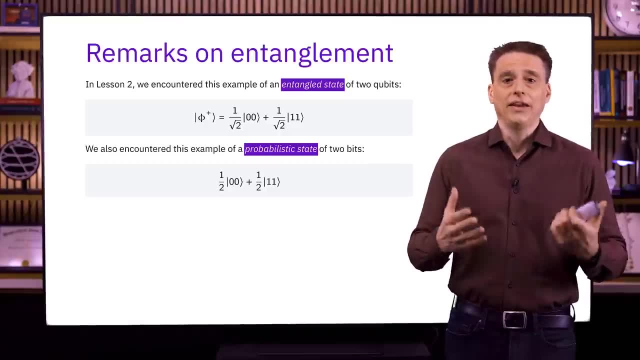 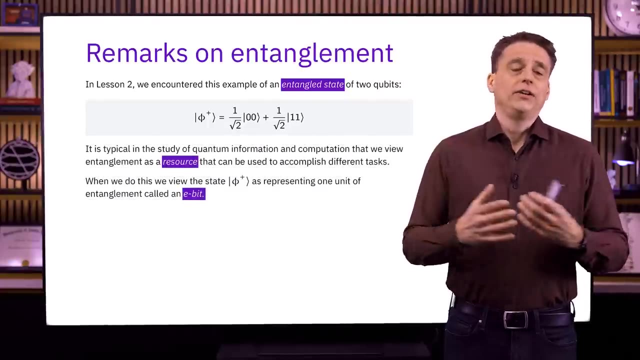 how we represent our knowledge using vectors. All three of the examples that we'll discuss in this lesson have this nature, in that they represent the state of entanglement that we cannot do with this state or with any classically correlated state. Indeed, it's very typical in the study of quantum information and computation. 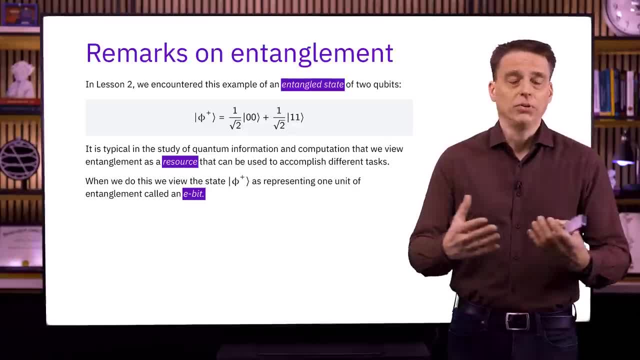 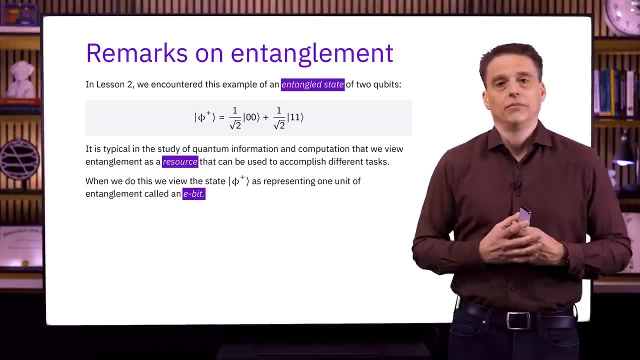 that we view entanglement as a resource through which different tasks can be accomplished, And when we do that, we view this state as representing one unit of entanglement. We refer to this unit of entanglement as an E-bit. The E stands for entangled or entanglement. 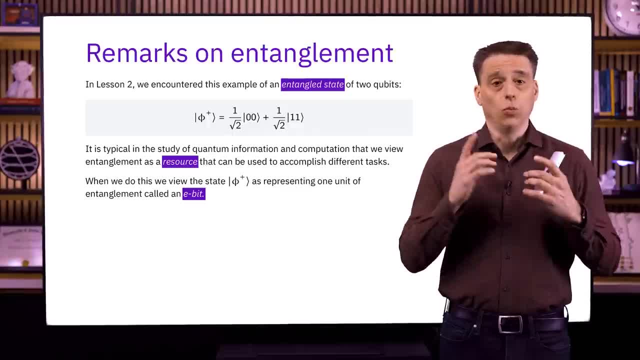 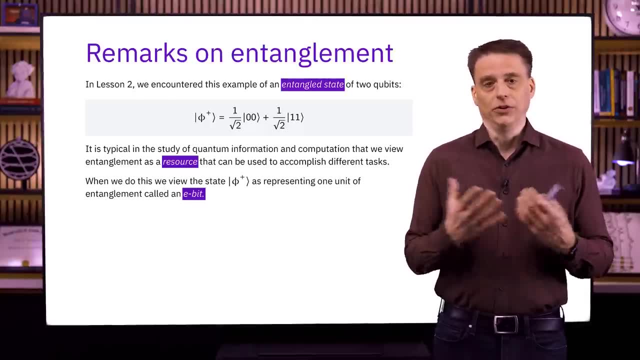 It's true that it's two qubits, but as a quantity of entanglement it's one E-bit. You can also view a pair of ordinary classical bits in the correlated probabilistic state from before as being a resource which is one bit of shared randomness. 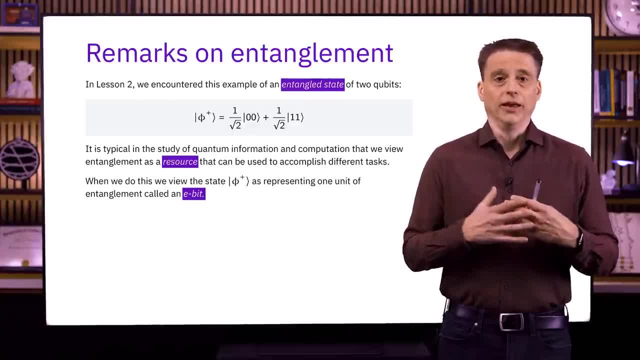 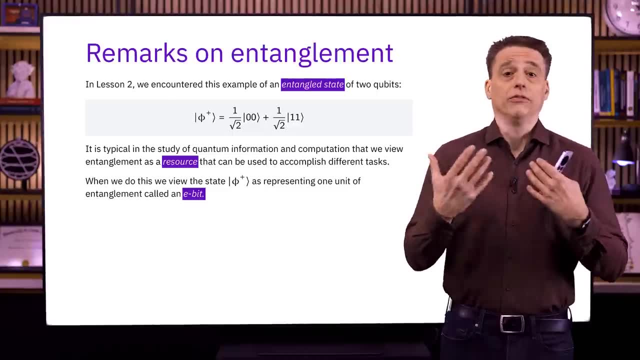 It can be very useful in cryptography to share a random bit with somebody, presuming that nobody else knows what that bit is, so that it can be used as a private key or as part of a private key, for example, for the sake of encryption. 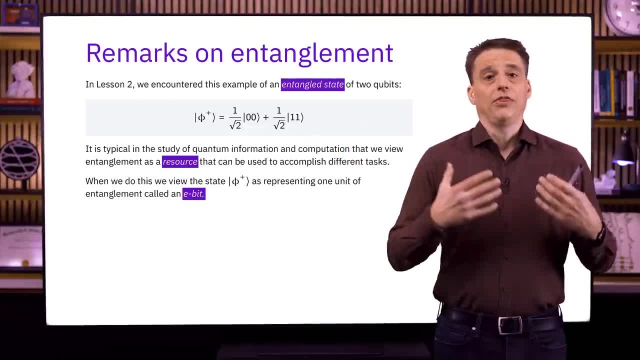 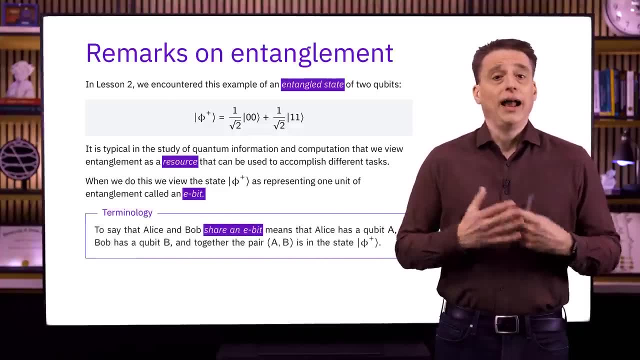 But in this lesson our focus will be on this entangled state And things that we can do with it. And just to clarify the terminology: when we say that Alice and Bob share an E-bit, what we mean is that Alice has a qubit named A, Bob has a qubit named B. 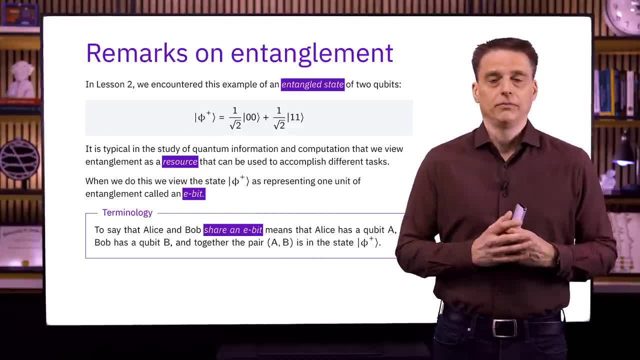 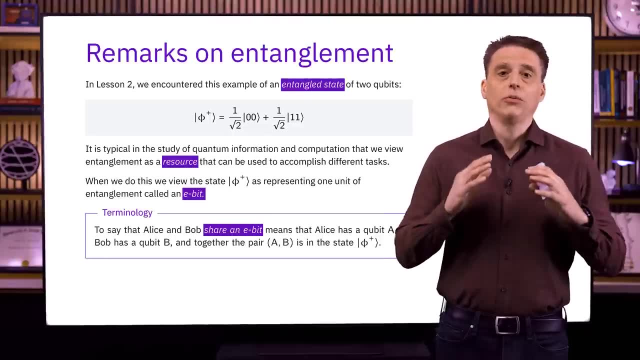 and together the pair AB is in the phi-plus state. It's not important what names we choose for the two qubits. of course We could choose different names, But throughout this lesson we'll stick with these names in the interest of clarity. 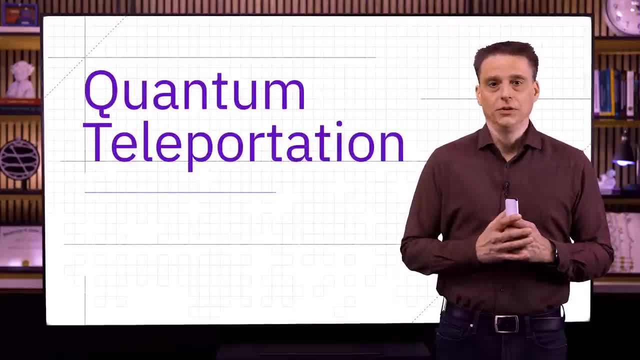 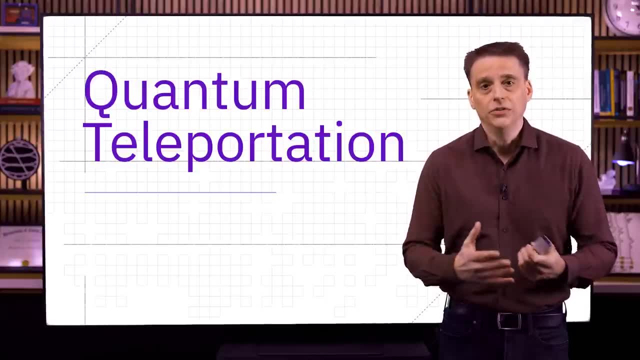 The first example of the lesson is this: This is quantum teleportation, which hereafter we'll just refer to as teleportation for the sake of brevity. What teleportation is is a protocol that allows a sender to transmit quantum information. 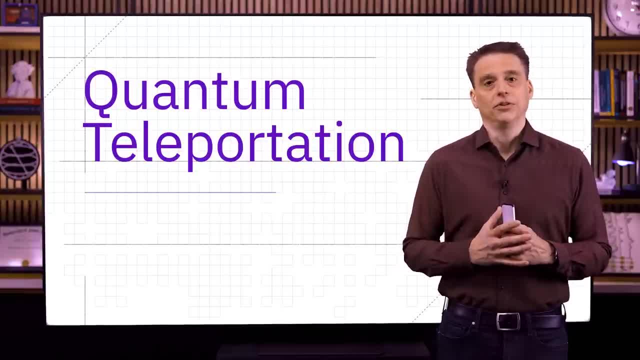 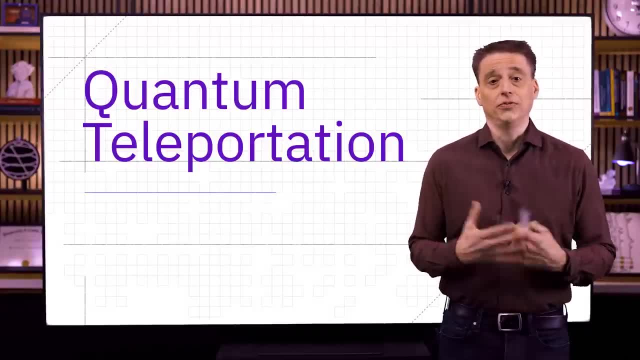 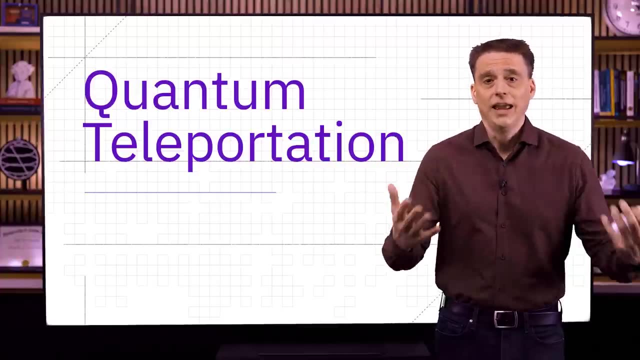 to a receiver using only entanglement and classical communication to accomplish that transmission. It has absolutely nothing to do with the typical interpretation of the word teleportation in science fiction, which is that matter disappears at one location and appears in another. It's not just a name that's meant to conjure that as an image or as a metaphor, so to speak. 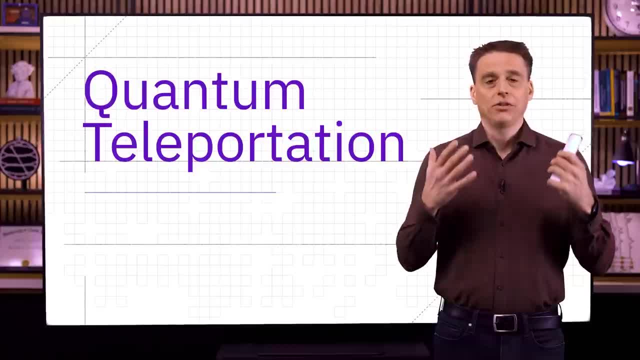 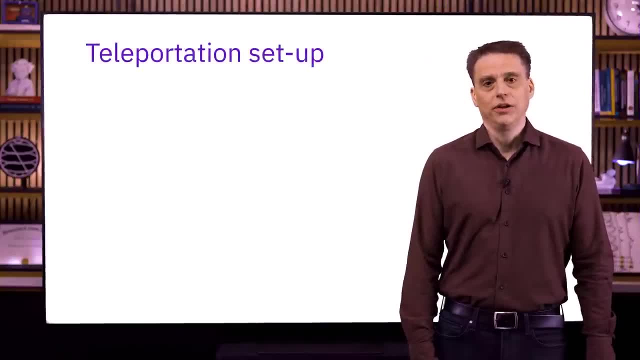 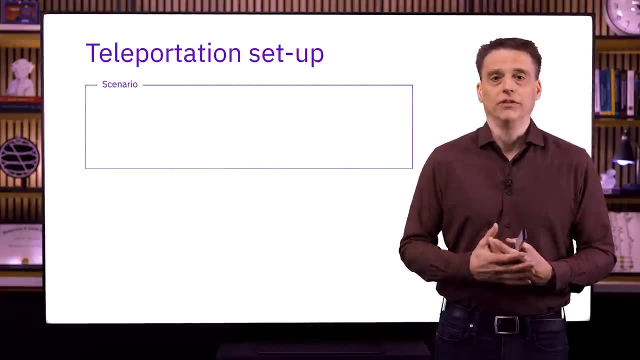 What's getting teleported is quantum information, not matter, and that's happening through a transmission of classical information, together with entanglement. To understand exactly how teleportation works, it's helpful to begin by setting the stage, so to speak. What we'll do is to imagine a scenario involving Alice and Bob, and that scenario is as follows. 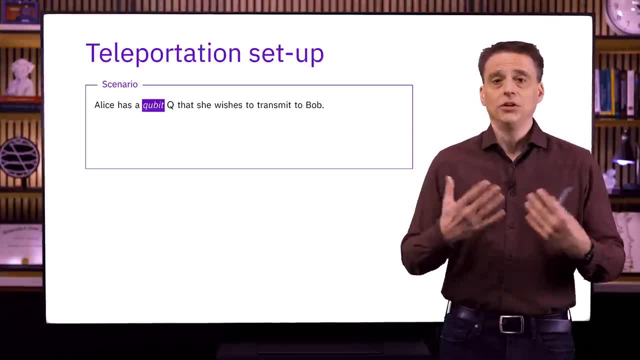 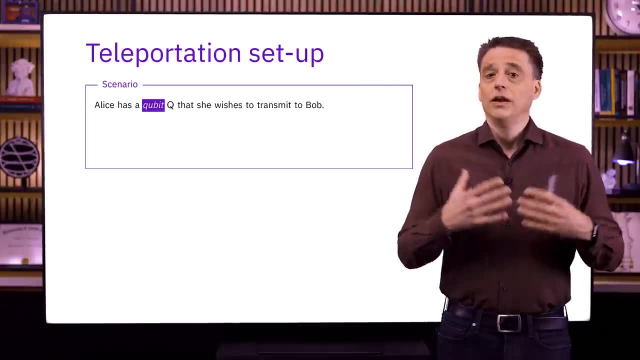 Alice wants to send a cube that she would like to transmit to Bob, meaning that she wants Bob to hold in his hands a qubit that's in exactly the same state that Q is in as they begin the protocol. In other words, we're talking about the fundamental problem of information transmission or communication. 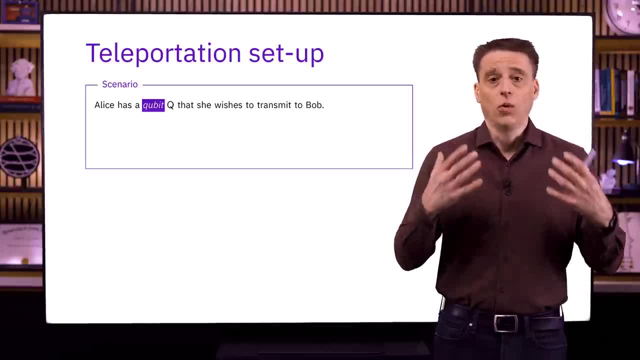 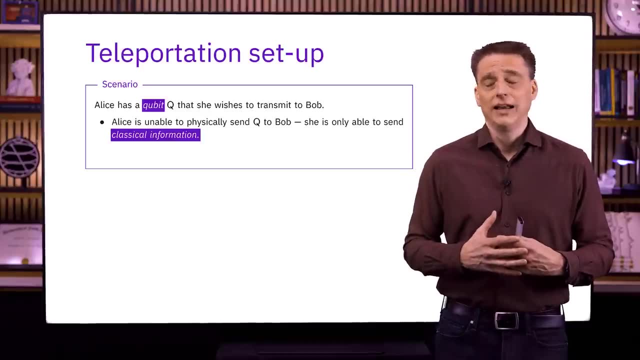 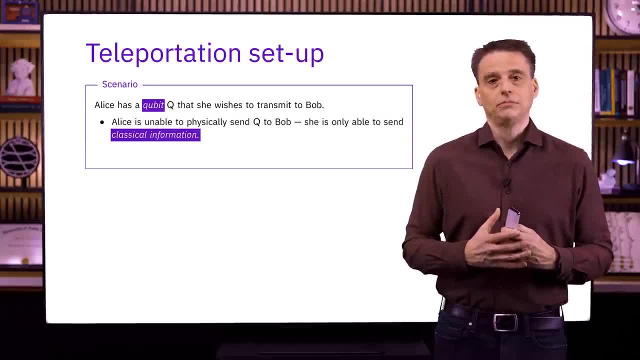 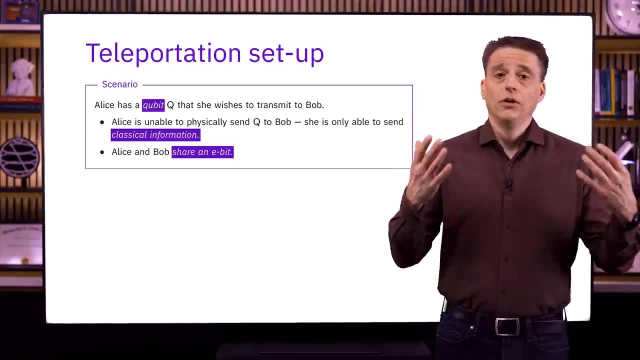 all that she can do is to send classical information to Bob. Alice and Bob also have an additional resource, which is that they share an ebit. So that's the scenario. It's easy to imagine situations where the constraint that Alice can't physically 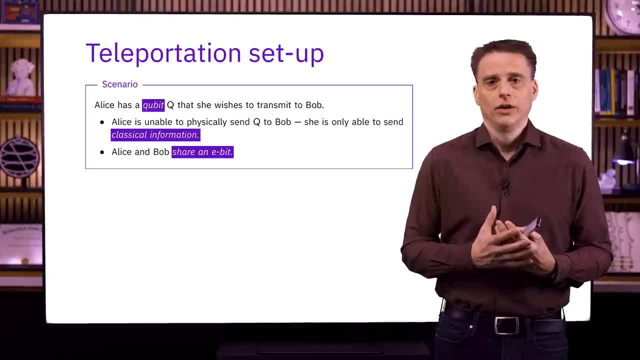 send Q to Bob is a reasonable abstraction. If Alice and Bob were on different continents, for instance, or if Alice didn't know Bob's exact location, then physically sending a qubit would probably be pretty challenging. But classical communication is of course not only possible. 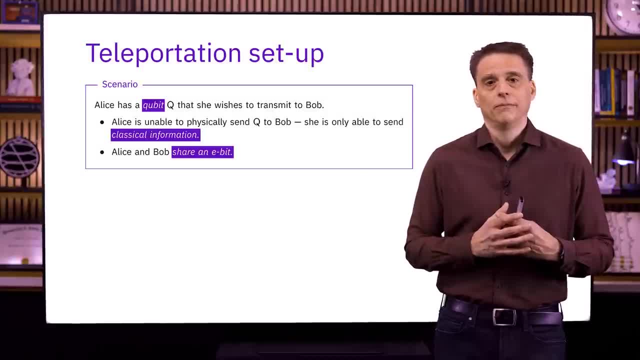 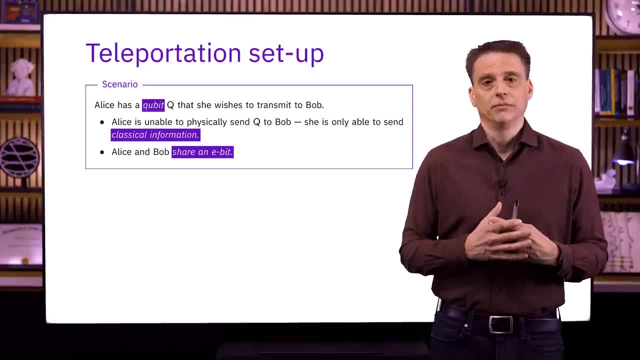 but quite inexpensive under those circumstances. Now one might ask whether it's possible for Alice and Bob to accomplish this task without even needing the shared ebit. In other words, is there any way to transmit a qubit using classical communication alone? The answer is no. it's not possible to transmit quantum information using 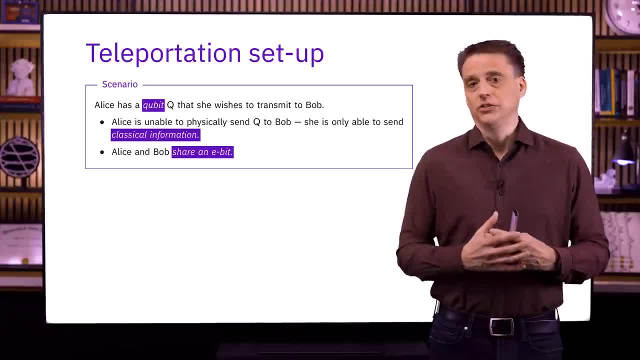 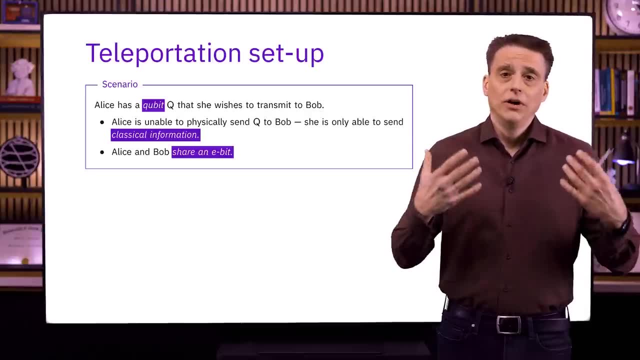 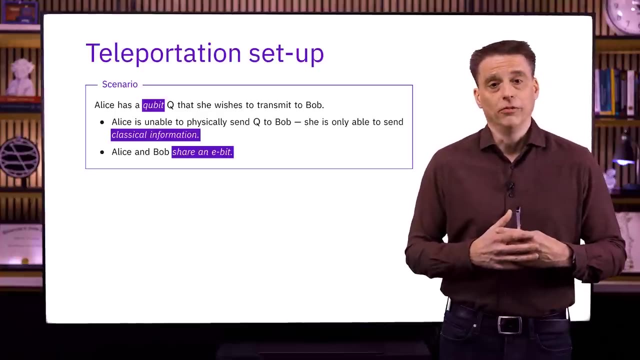 classical communication alone, And that's not too difficult to prove using some basic quantum information, which we'll see in the third unit of the series. For now, an intuitive way to think about it is to think about the no-cloning theorem. Imagine that there was a way to send quantum information using classical communication alone. 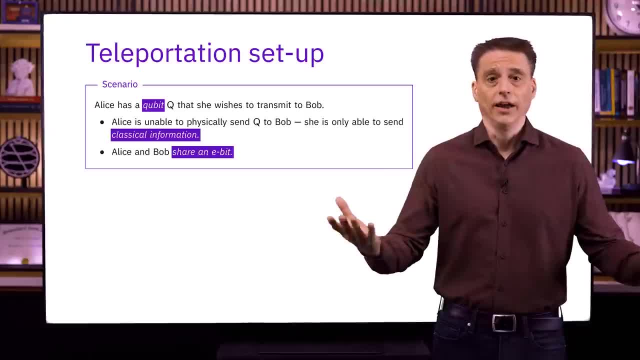 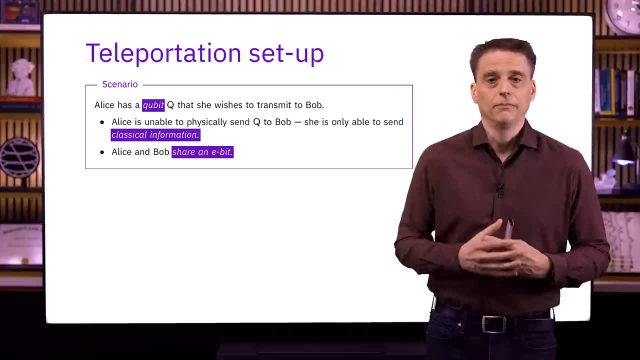 But classical communication can easily be copied and broadcast. So that means the classical communication could be broadcast to two receivers, Bob and Charlie. let's say, If they both received the same classical information from Alice, then would they both end up with Q. 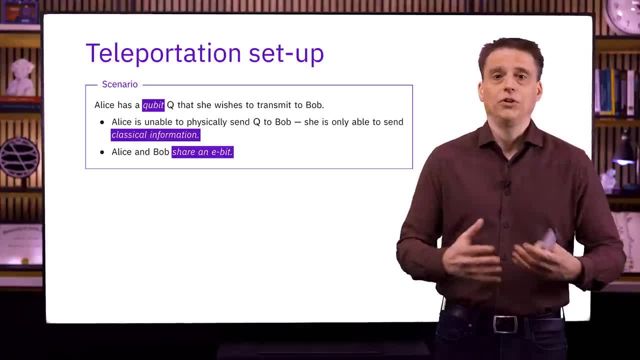 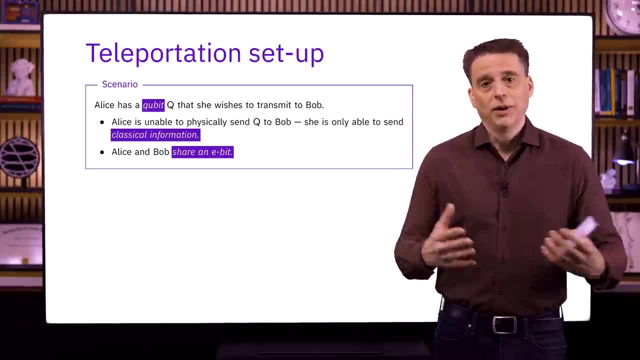 That would suggest that we cloned Q, but we know that that's impossible. Just as an aside, let's observe that it certainly is possible to describe quantum state vectors using classical information. Every quantum state vector you'll see in this series is being described to you. 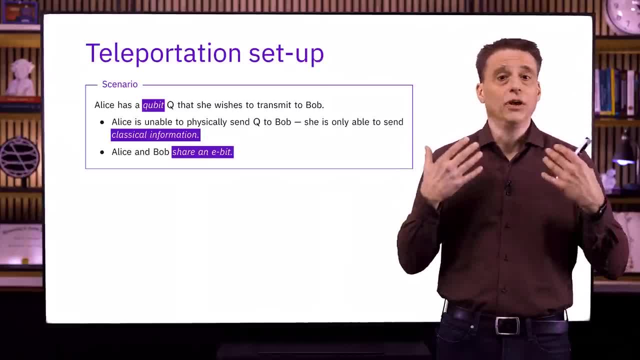 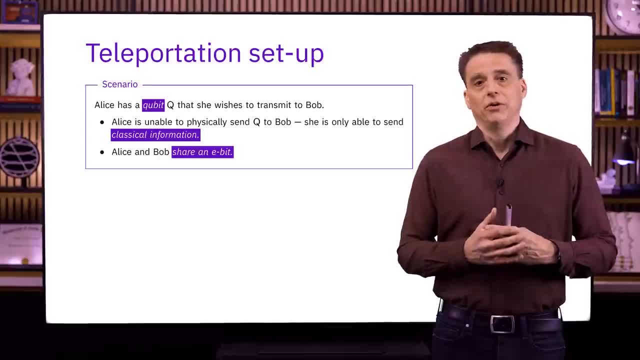 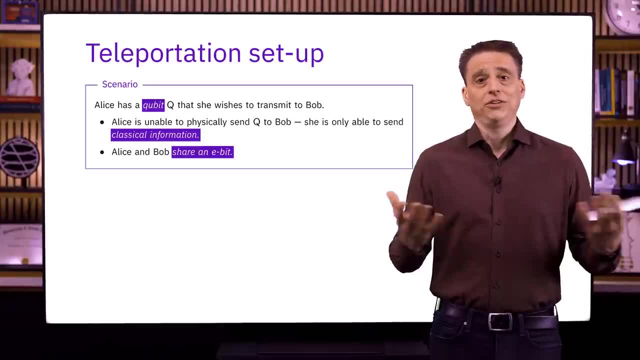 Let's look at this. Let's look at this In general. we could imagine describing whatever state Q is in using classical bits, perhaps to some precision, But that's not quantum communication. That's just describing quantum states as vectors, And we'll come back to the distinction between them in just a moment. 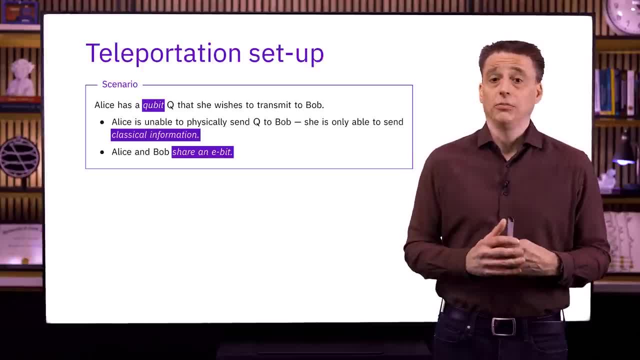 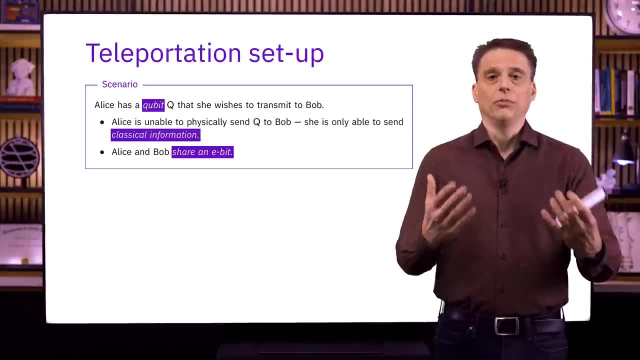 Getting back to the scenario, however, and working under the assumption that Alice and Bob do share an E-bit, we will see that Alice and Bob have everything they need to accomplish the task, And that's what the quantum teleportation protocol does does specifically using two bits of classical communication. 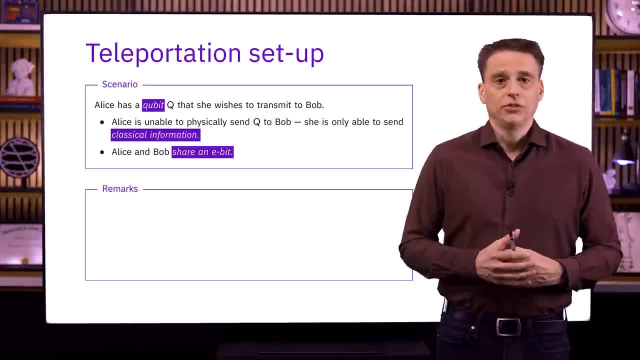 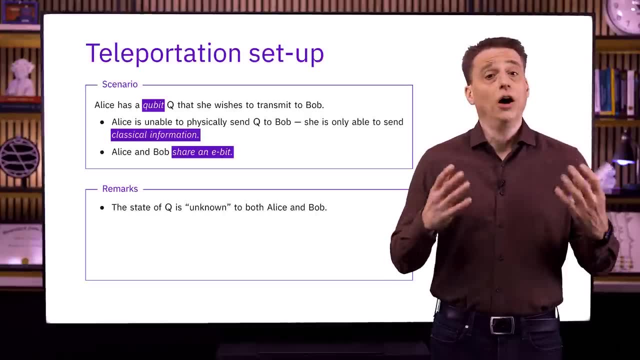 Before getting into these details, however, let me make a few quick remarks just to make sure that the assumptions are clear. First, we're assuming here that the state of Q is unknown to Alice and Bob, So, in particular, Alice can't send Bob. 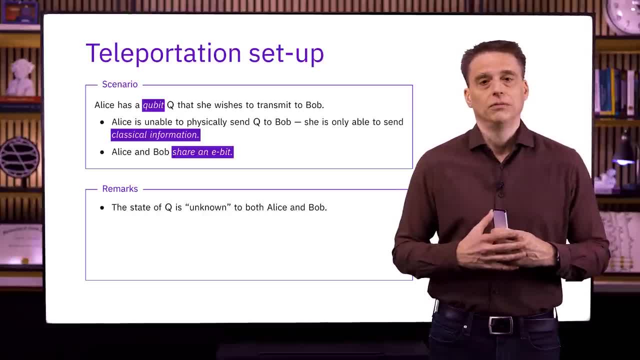 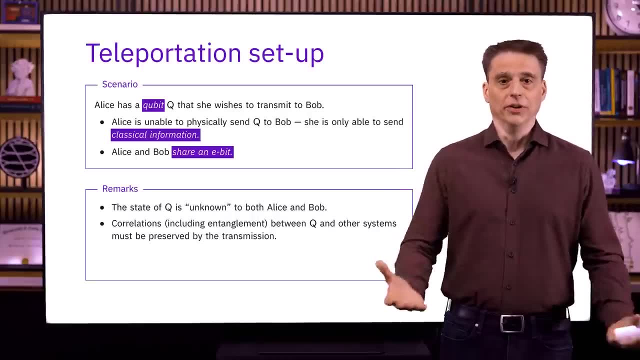 a description of the state Q, because she doesn't know it in general. We also have to consider the possibility that Q is correlated with other systems, including the possibility that it's entangled with other systems And the transmission of this qubit to Bob. 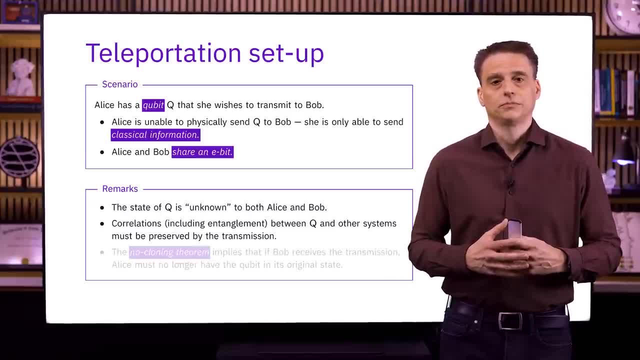 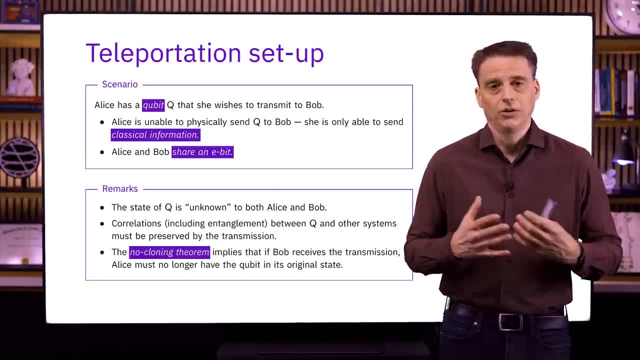 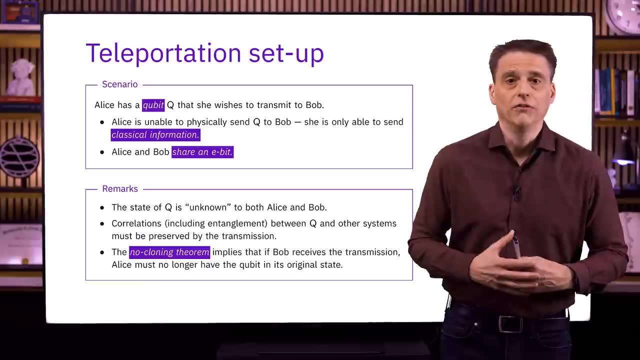 must preserve those correlations. Finally, I mentioned the no-cloning theorem when I was talking about trying to communicate qubits classically. But there's another connection here with the no-cloning theorem, which is that if Bob receives the transmission of this qubit Q 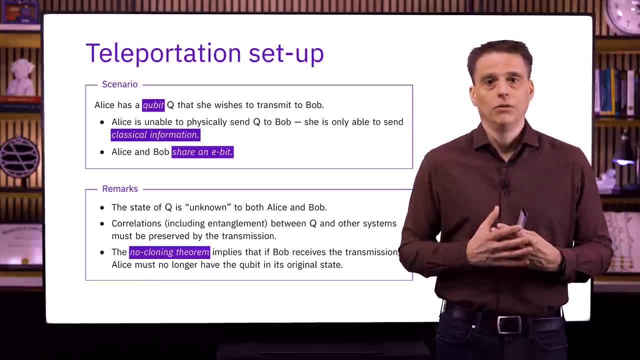 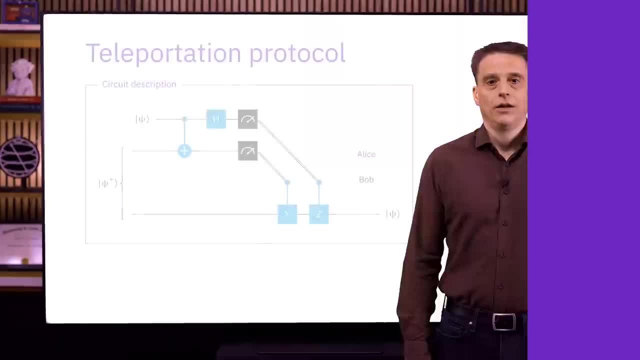 from Alice, then she must not have it anymore because Q can't be cloned, And that's just something to keep in mind as we consider the teleportation protocol. The teleportation protocol can be described in a pretty simple and direct way with the quantum circuit. 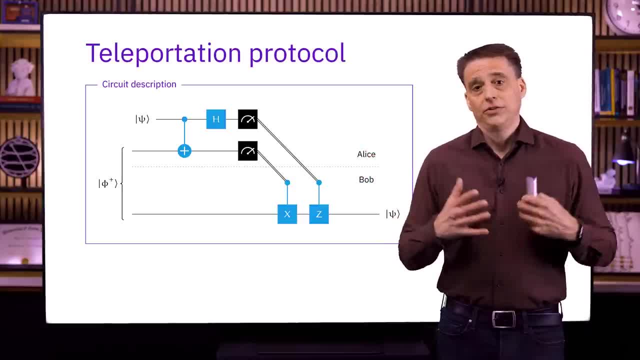 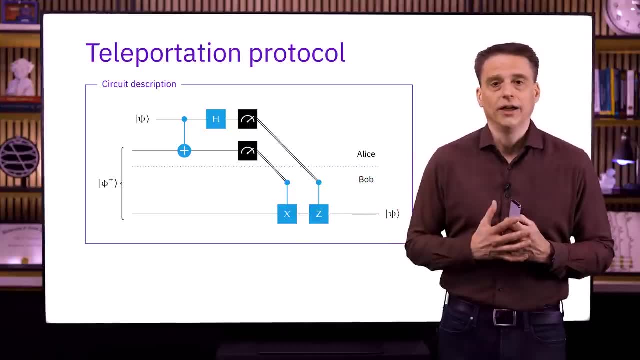 diagram. as you can see right here, It's slightly stylized in that it depicts the separation between Alice's part and Bob's part, but otherwise it's just a quantum circuit diagram. Everything above the dotted line represents Alice's actions and everything below represents Bob's actions. 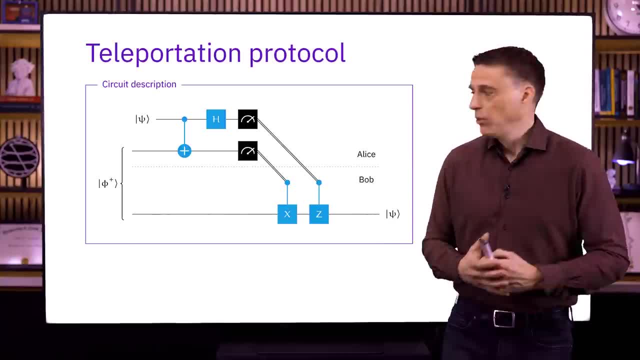 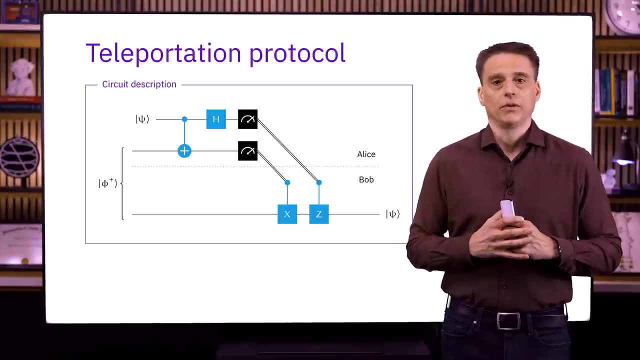 Time goes from left to right, as always, and we see that we start with these two qubits here being in a phi plus state. So this is the E bit that Alice and Bob start with. We can put labels on the qubits to make clear which one is which. 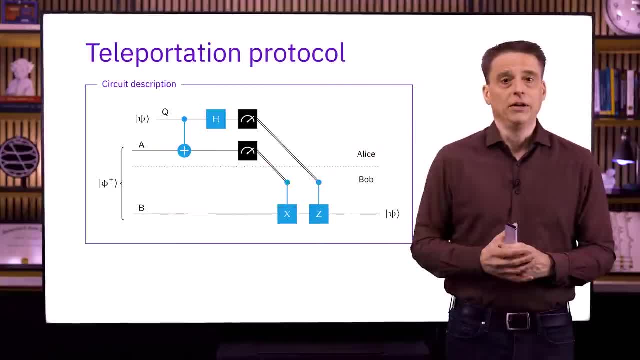 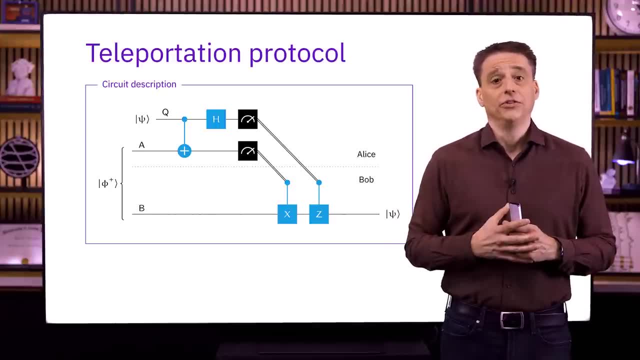 So this is the qubit A and this is the qubit B. that form the E bit and this is the qubit Q that Alice wishes to transmit to Bob. Here we're hypothesizing that the state of this qubit Q is psi, but a little bit later. 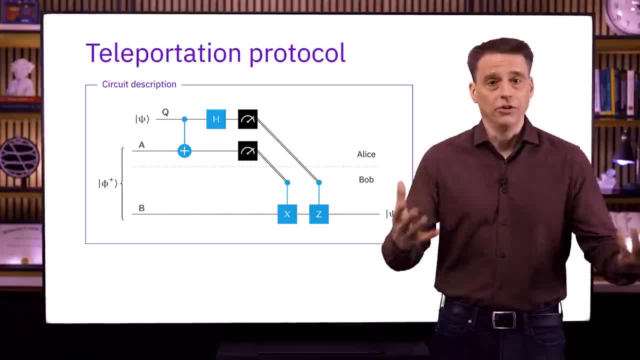 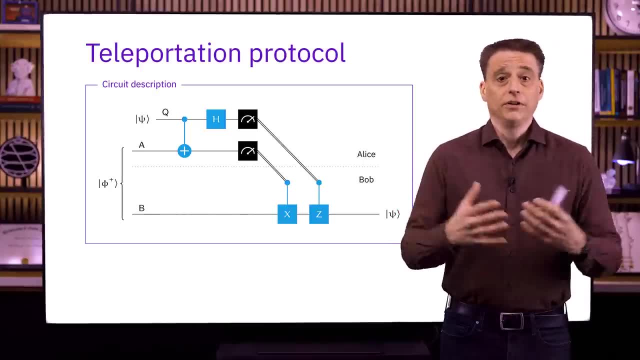 on. we'll consider the possibility that Q is entangled with some other system And what the diagram is claiming- because we've written psi down here, is that this circuit effectively does transmit whatever state psi we had up here on Alice's part, down here to Bob's part. 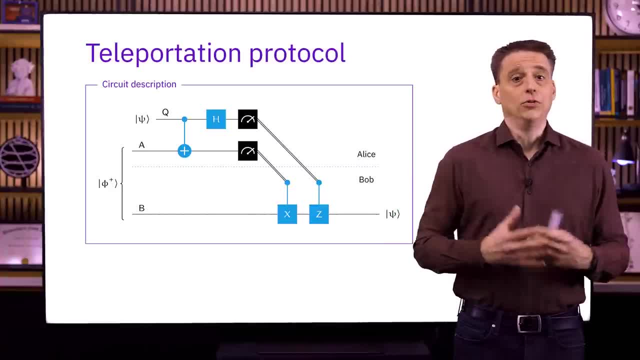 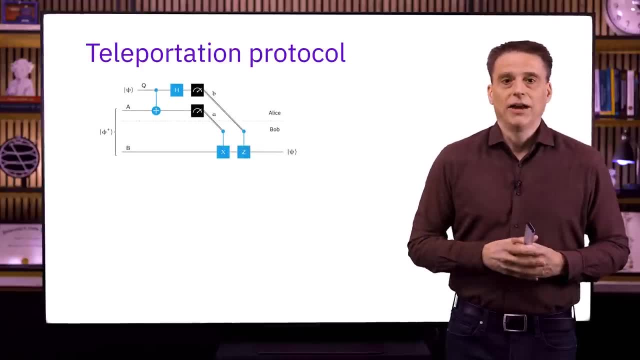 The only communication that we have crossing the line between Alice and Bob is the two classical bits that are represented by these double lines right here. Let's shrink this diagram down a little bit so that we have a little bit more room, and let's see what happens. 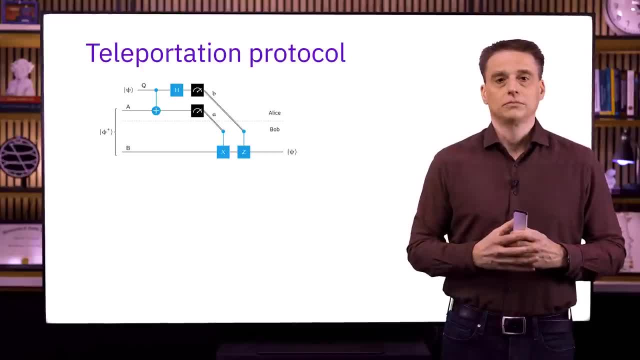 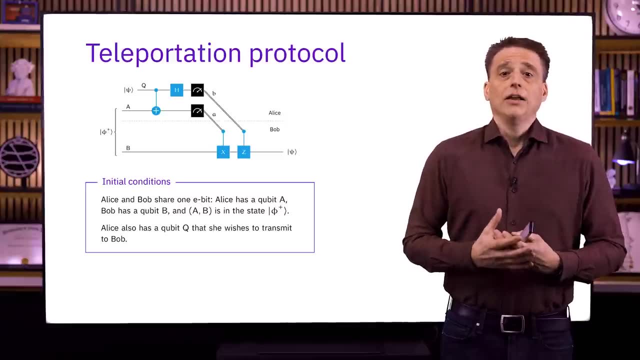 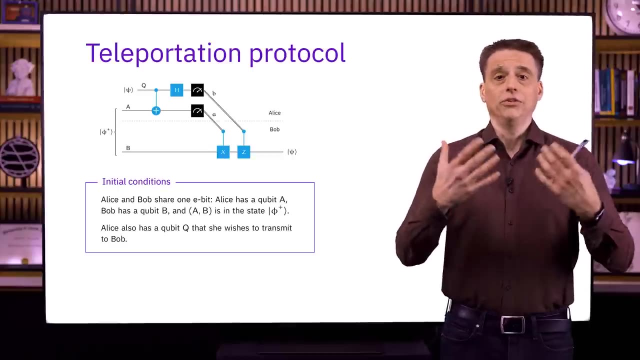 Let's examine the circuit more closely. I've already described the initial conditions, but just to recapitulate, Alice holds a qubit A and Bob holds a qubit B, where A and B together are in a phi-plus state. So that's what it means to share an E bit. 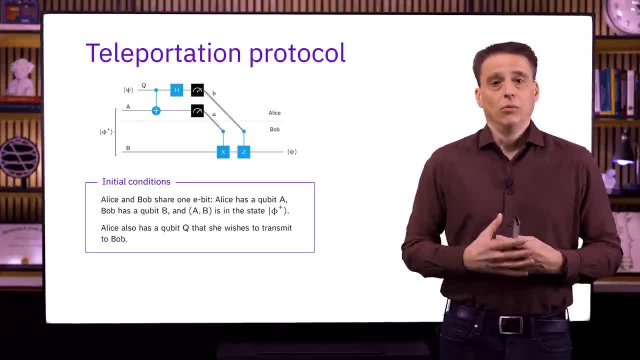 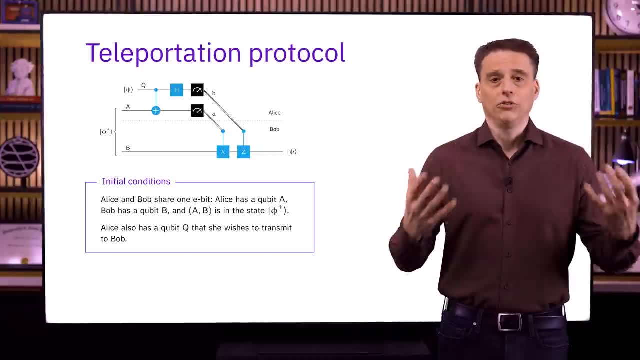 Alice also has this qubit Q that she wishes to transmit to Bob, and we're considering the case that Q is in some arbitrary quantum state, psi. Now we don't know anything about how Alice and Bob came into possession of this E bit. 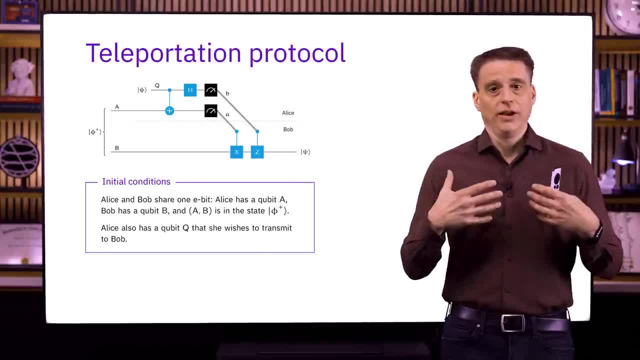 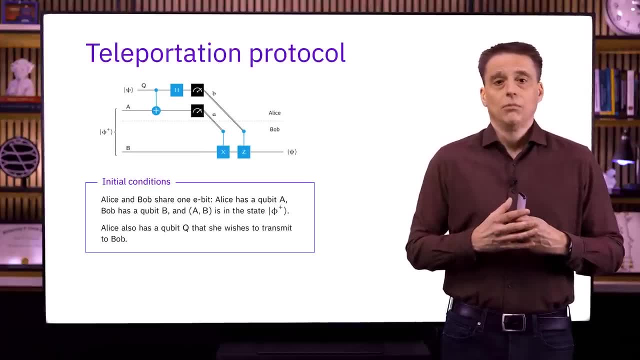 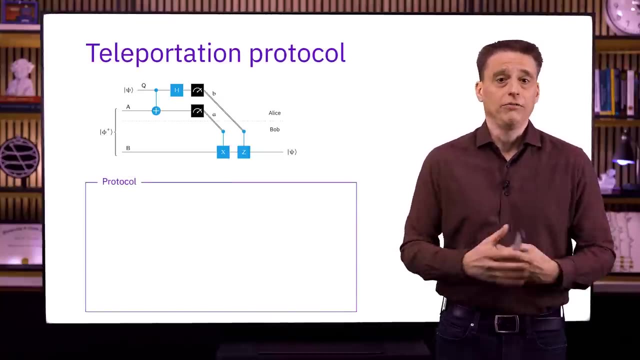 It could be that they've had it for a long time. Maybe they created it some time ago when they were in the same location and they've been saving it for this occasion, But those details aren't relevant here. The steps that happen next, which represent the teleportation protocol itself, are as: 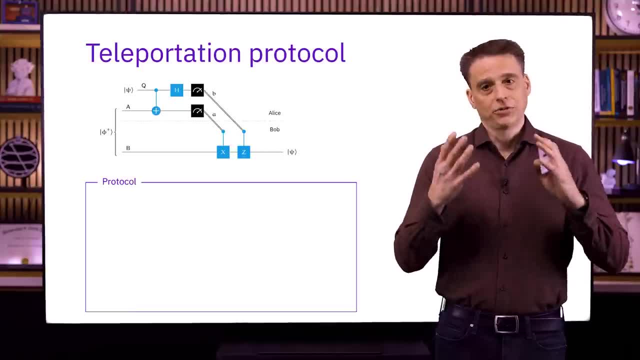 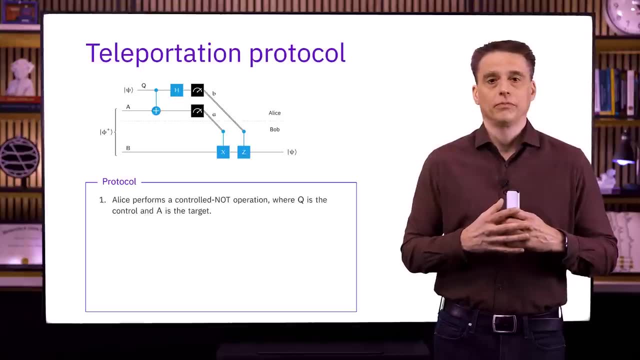 follows And, just to be clear, these are the steps that the diagram describes and we're just going to write them down and see what happens. Alice first performs a controlled- NOT- operation, where the qubit Q that she wants to send to Bob is the control and the qubit A is the target. 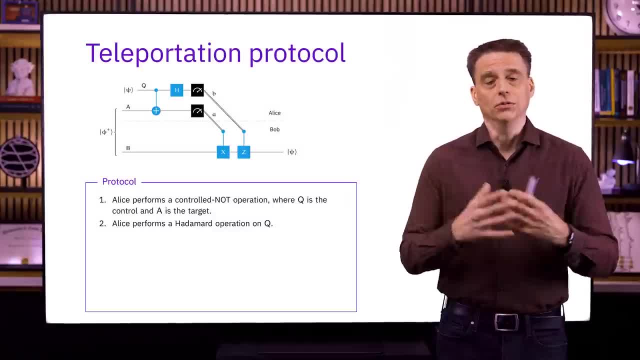 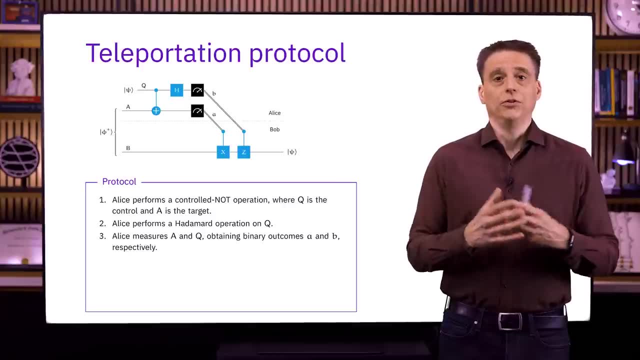 The next step is that she performs a Hadamard operation on Q And then she measures the two qubits that she holds, A and Q, with respect to standard basis measurements, And we let lowercase a be the outcome of the measurement of the QBIT A and we let 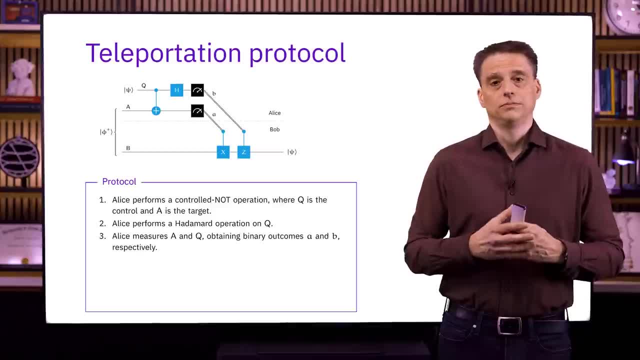 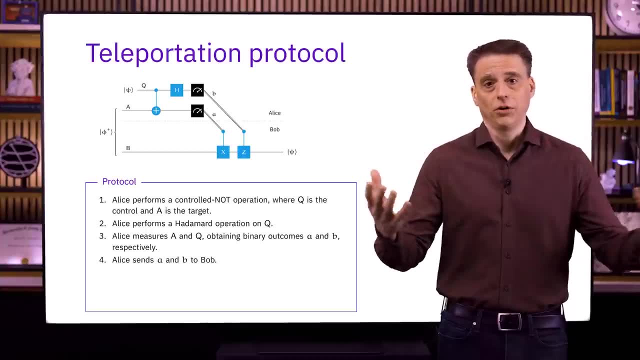 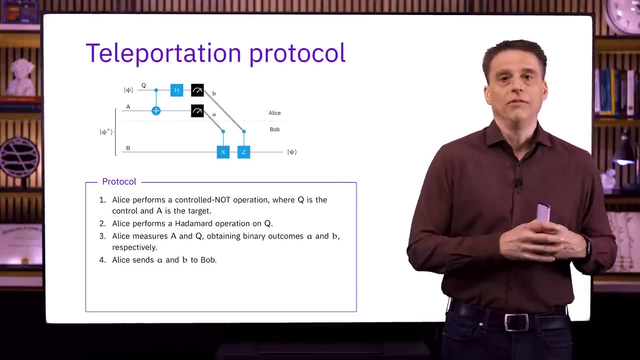 it then be the outcome of the measurement of the qubit Q. Alice then sends those two classical bits to Bob, and this is the only communication that is involved in this protocol and that is indicated in the diagram by the fact that these two про cross the dotted line between Alice and Bob, which you can think of as representing. 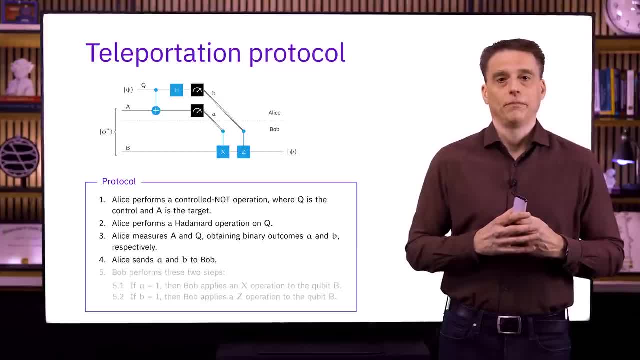 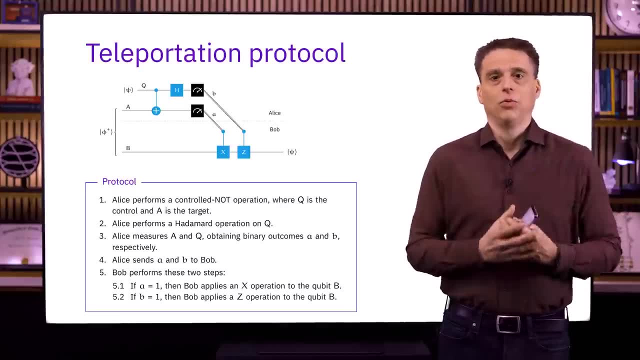 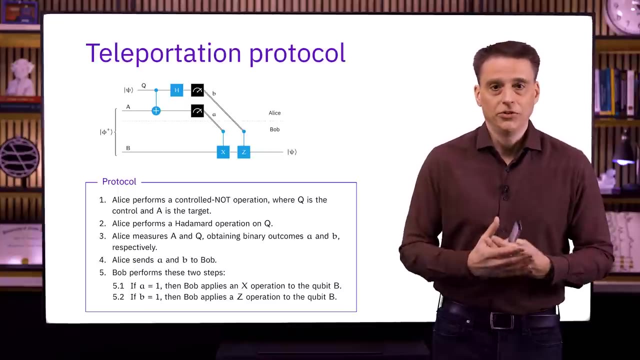 whatever distance separates them. About distance introduced bits A and B, he does two things. First, if A is equal to one, then he performs an X operation, or in other words a, NOT gate, on his qubit B, and otherwise, if A is equal to zero, 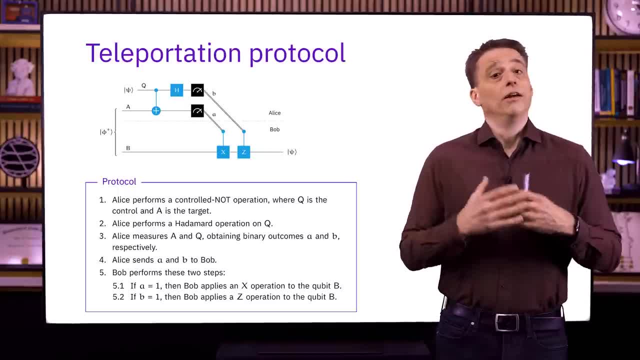 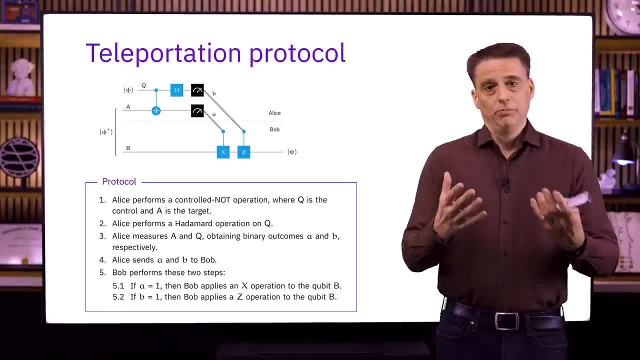 then he doesn't do that. And along similar lines, if B is equal to one, then Bob performs a Z operation or a Z gate or a phase flip, also on the qubit B, and like before, if B is equal to zero. 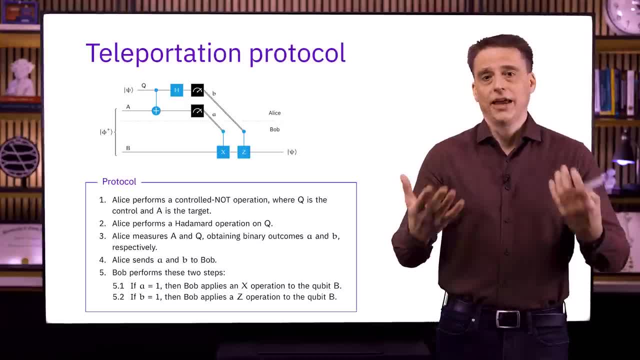 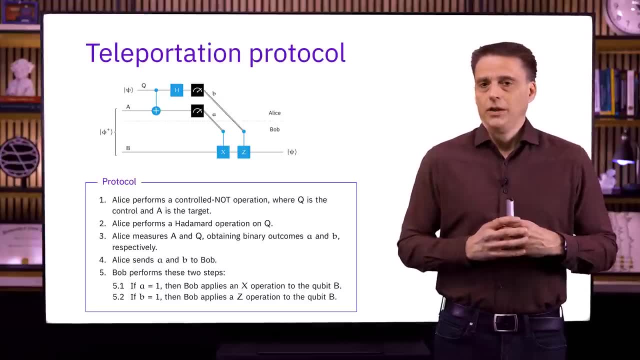 then he doesn't do that. This is all indicated in the figure where we have these controlled X and controlled Z gates, where the controls are the two classical bits. You don't have to think of these gates as being control gates if you don't want to. 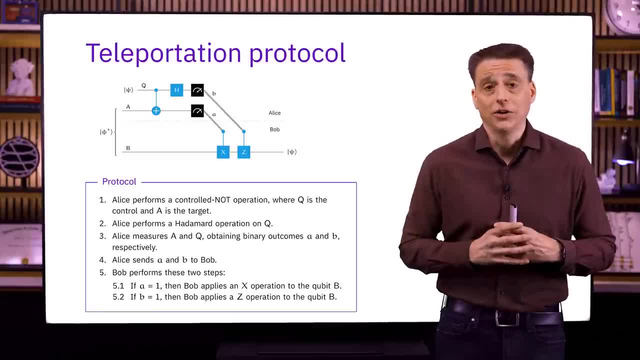 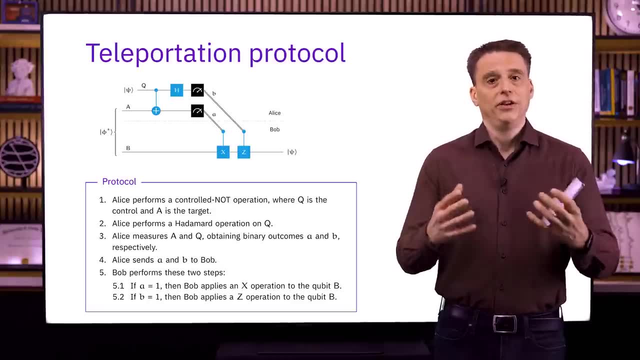 This is just a handy way to express what we want in the form of a circuit diagram. The point is that Bob applies an X gate to the qubit B if A is equal to one, and then he applies a Z gate to the qubit B if B equals one. 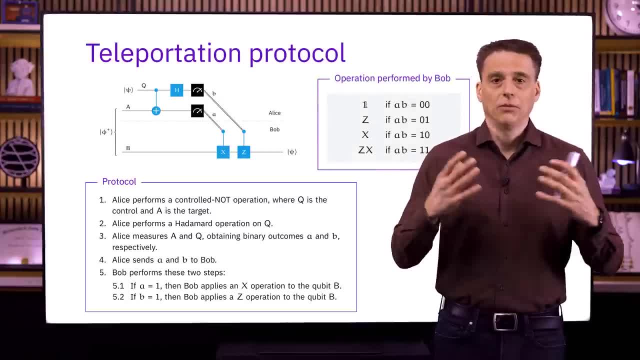 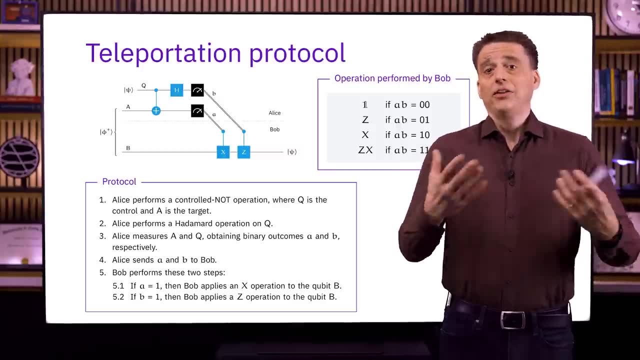 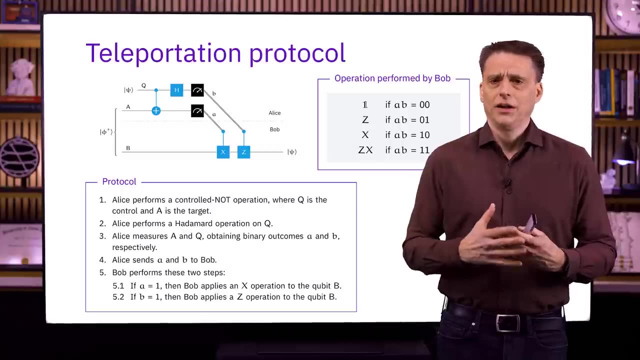 And for the sake of convenience, later we can write down explicitly the combined operation that Bob performs on his qubit B, depending upon the classical bits that Alice sends. So that is the teleportation protocol. It's pretty simple really. The fact that it actually works is a different matter. 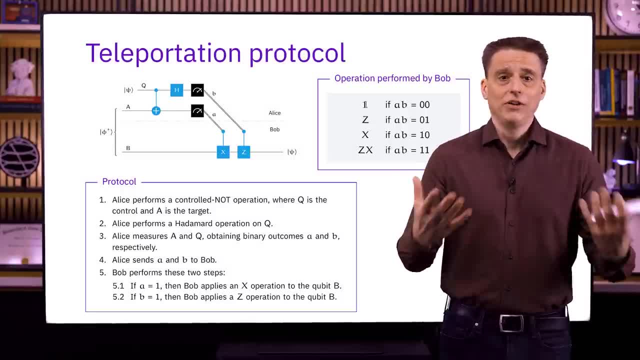 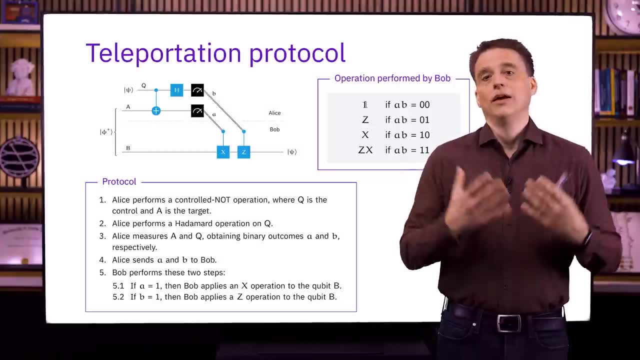 And although the analysis isn't that complicated, you should not feel that you're missing something if you don't immediately see why it works. That's why we need to go through an analysis And that's what we will do next, To analyze the teleportation protocol. 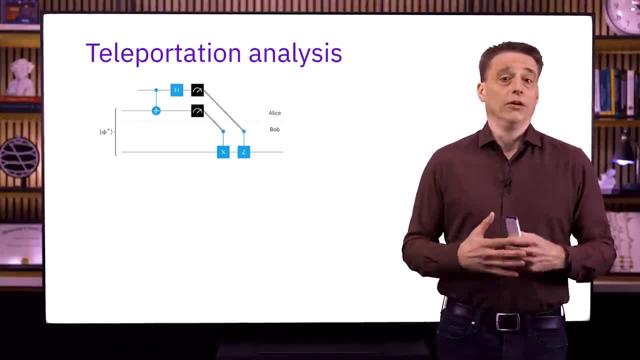 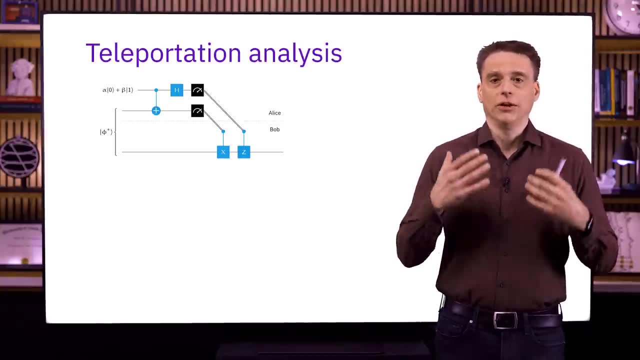 we'll work through it one step at a time to see what the states of the three qubits are at different points in time. We're gonna first consider the case that the top qubit is in the state alpha zero plus beta, one where alpha and beta are any complex numbers. 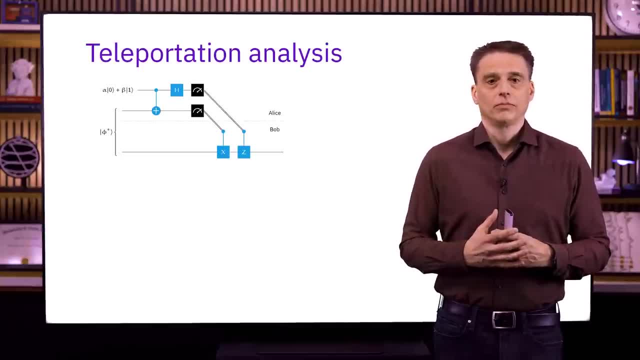 that cause this vector to be a unit vector. This is the qubit Q that Alice is trying to transmit, but we don't really care what it's called at this moment. A little bit later we'll take a look at the situation in which this qubit is entangled with another system. 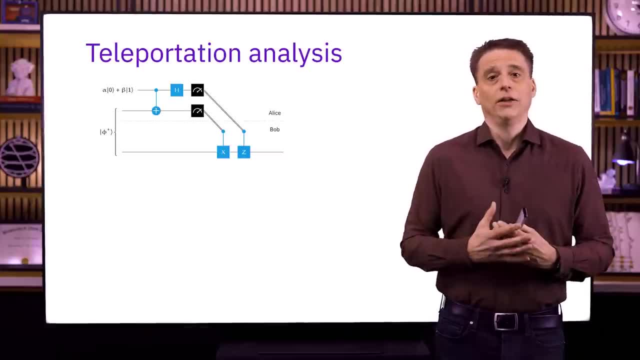 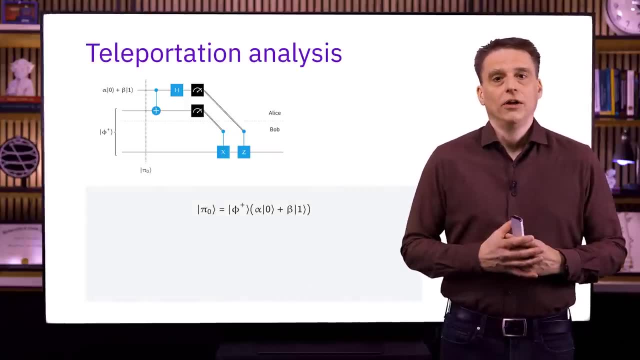 but this is a good starting point, just to keep things simple and to see how the analysis works a little bit more clearly. If we consider the state of the three qubits together here at the start, we see that this state has the form that you see right here. 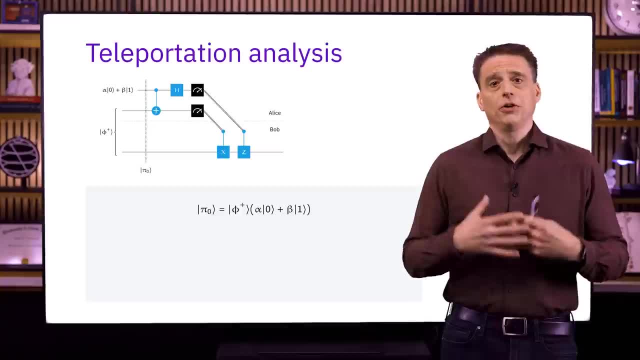 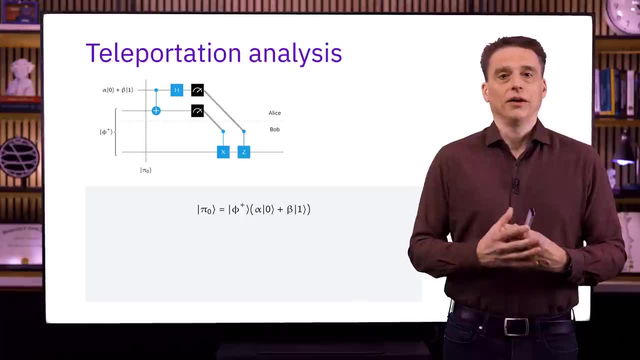 The first two qubits are in the five plus state. The third qubit is the top one according to the convention for ordering qubits that I described in the previous lesson, And so we take the tensor product to get the state of the three qubits together. 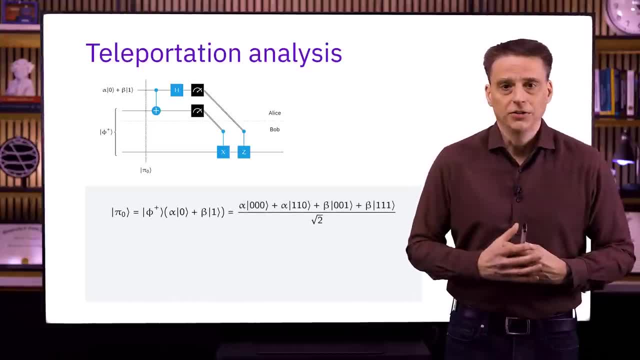 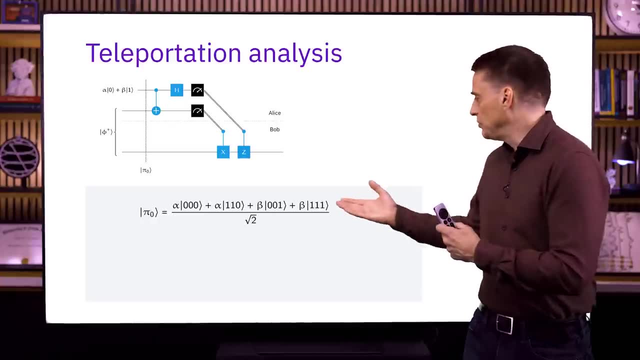 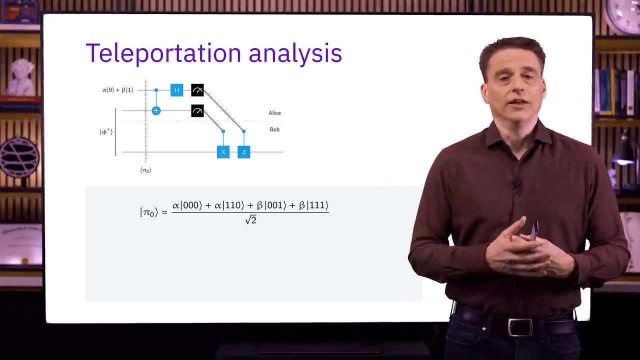 We can expand this expression by first substituting the definition of the five plus state and then computing the tensor product, And we get the state that you see right here. It's not always the best strategy, by the way, to completely expand out a vector like this. 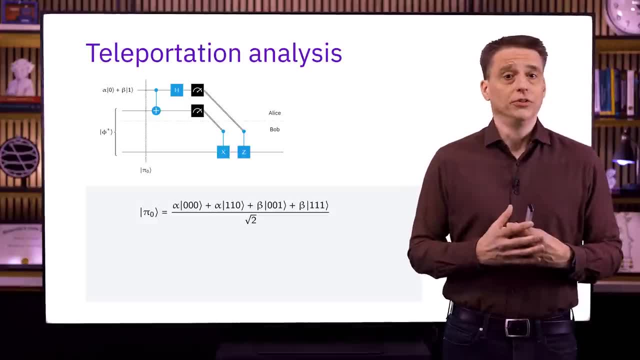 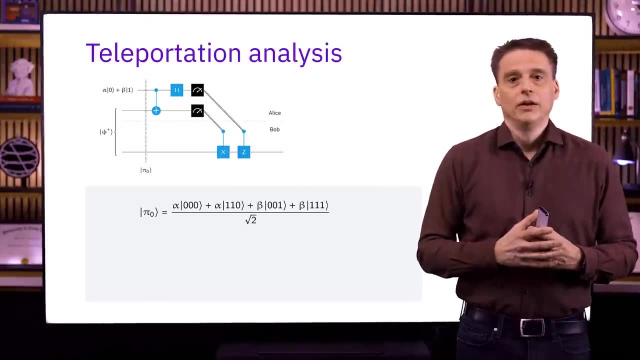 It's generally a good idea to wait until you have a good reason to do this, But here we do have a reason, which is that we would like to compute the action of this controlled, NOT gate, And by writing the state in this form we can very easily do that. 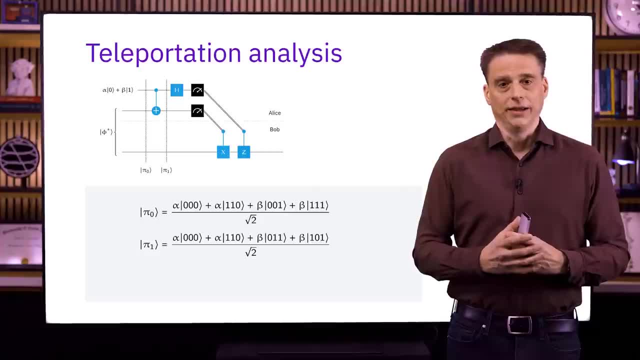 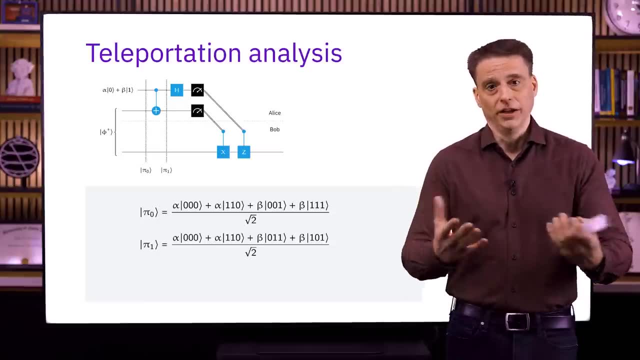 And, in particular, this is the state of the three qubits after the controlled, NOT gate is applied. The third qubit is the control qubit, because that's the one that's on top by our convention, And the second qubit, which is the middle one, is the target. 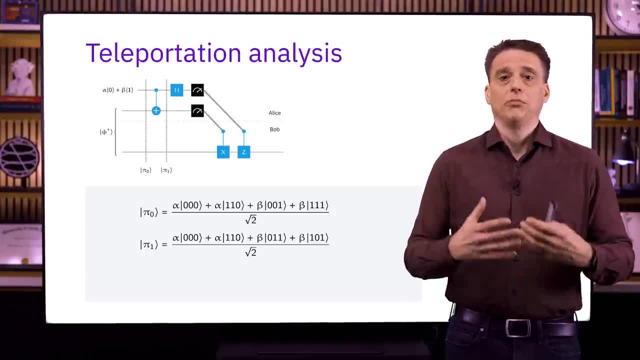 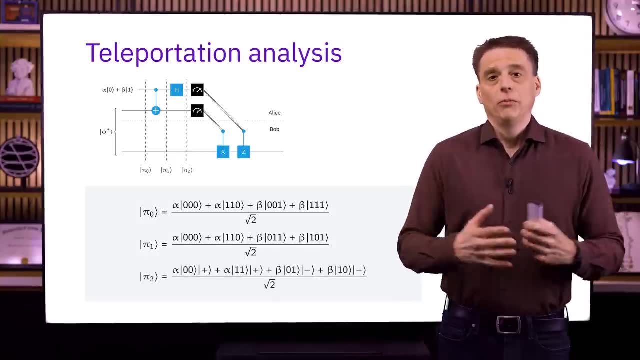 So we just operate on the kets accordingly. If the third bit is a zero, nothing happens, and if the third bit is a one, then we flip the second bit, Then we perform the Hadamard gate on the third qubit. 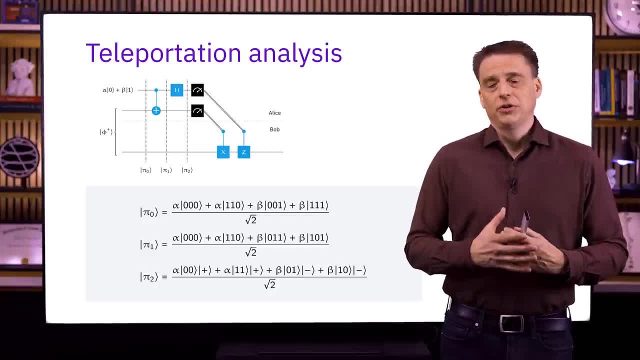 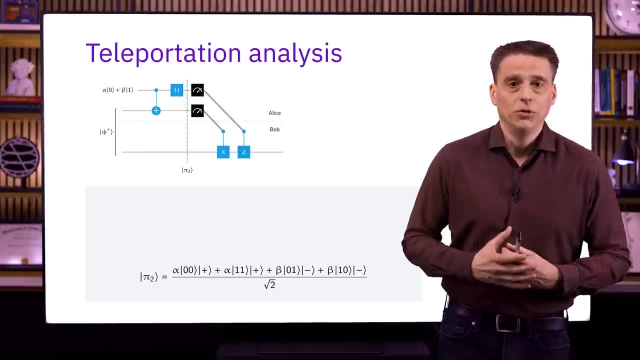 We can write the resulting vector, like you can see right here, substituting the plus and the minus state for the zero and the one state, And if we want to have enough room to expand this one out, we're going to need to shrink it down a little bit. 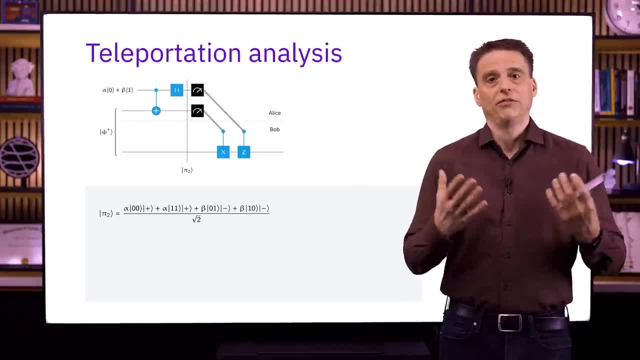 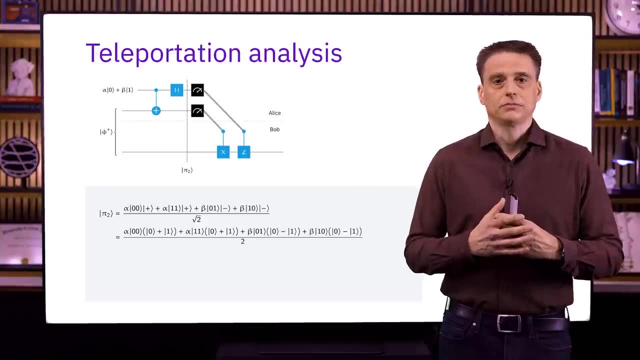 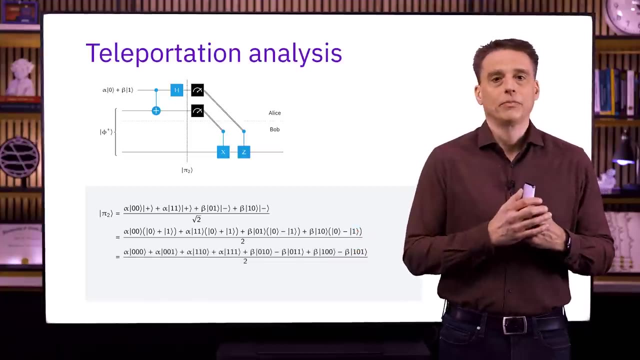 And now, by substituting the plus and the minus states with their definitions, bringing the square root of two into the denominator, we get the state that you see right here. And by expanding that one out, we get the state that you see right here. 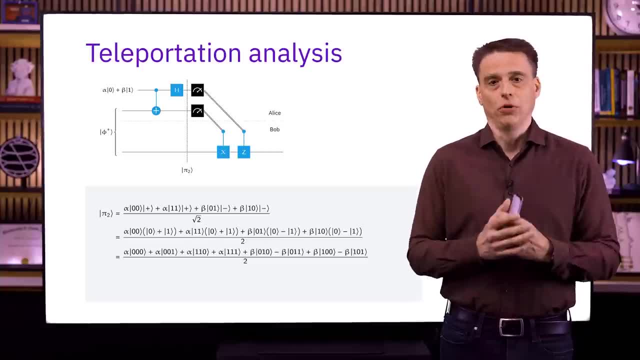 So that is the state of the three qubits after Alice performs her two operations. Alice then measures, And if we want to analyze the measurements, what we do is to isolate the standard basis vectors for the systems being measured, just like we talked about in lesson two. 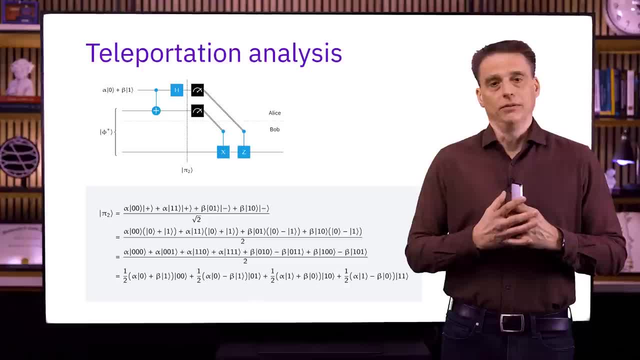 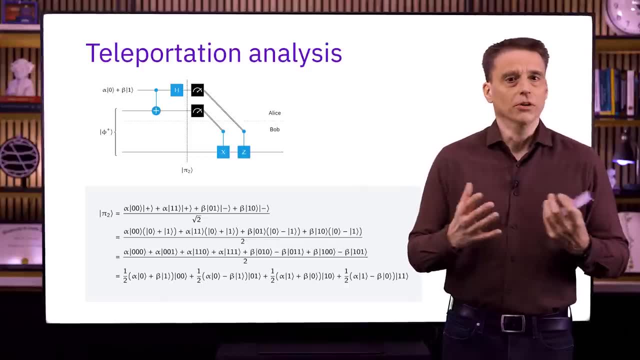 And if we do that in this particular case, this is what we obtain. And if you look at that expression for a moment, it might seem a little bit peculiar, Because now it looks like the first qubit, which is the bottom qubit, somehow depends. 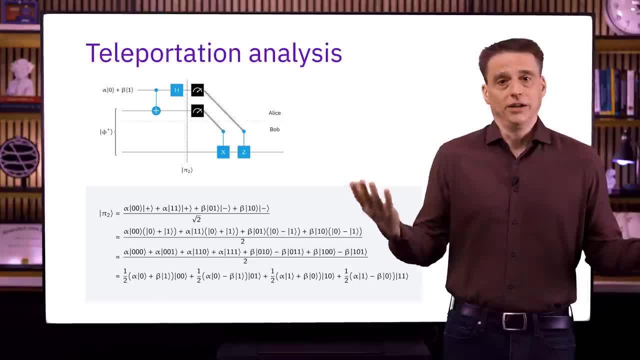 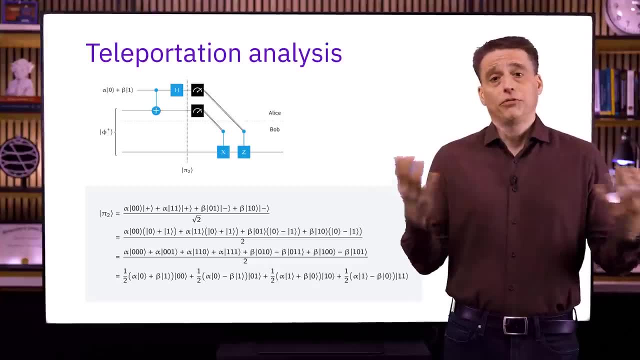 upon alpha and beta, even though at this point there hasn't been any communication across the dotted line. But that's just an illusion. Remember that scalars float freely through tensor products, so there's really no sense in which alpha and beta are associated. 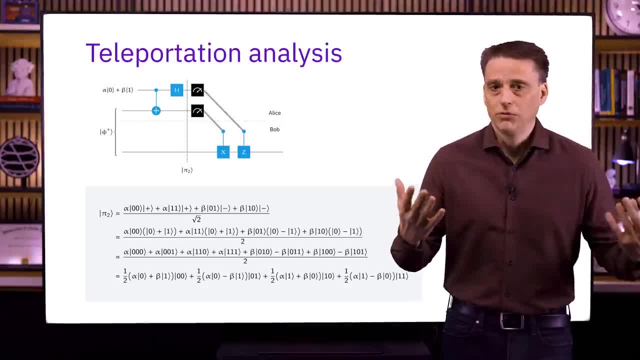 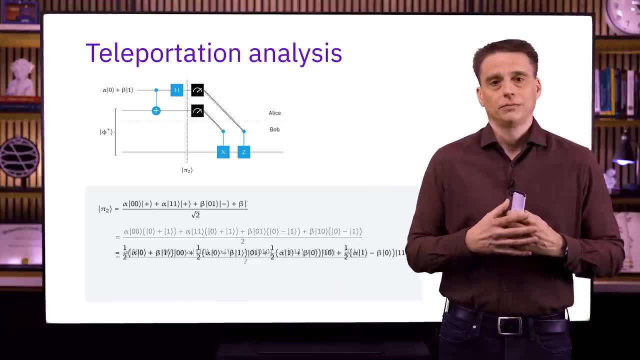 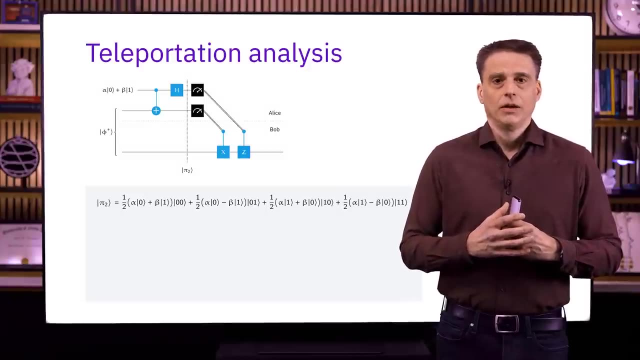 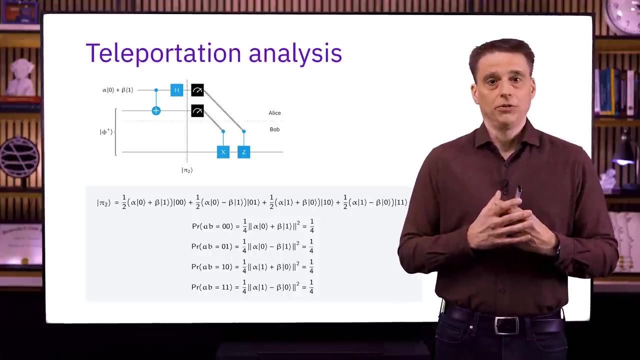 All we've really done here is to use parentheses in accordance with the multilinearity of tensor products. Anyway, that's the form that we need to see what the measurement does, And we can see one interesting thing right away, And that is that the probabilities of the four possible measurement outcomes are always 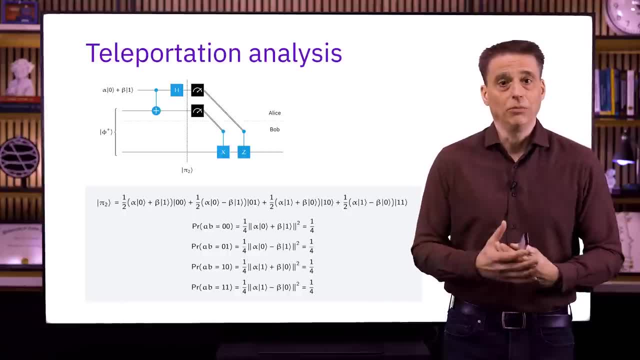 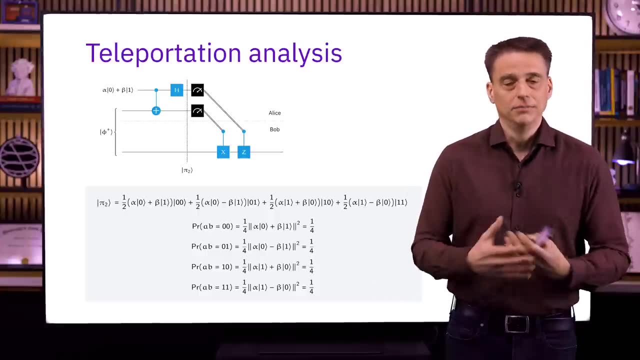 uniform. The probability to measure each pair of measurement outcomes is one-quarter. So, in particular, there's no dependence whatsoever on alpha and beta. We can see that in each case, by computing the Euclidean norm, squared of whatever vector is tensored to the standard basis vector that we isolated, and in each case we have a one-quarter. 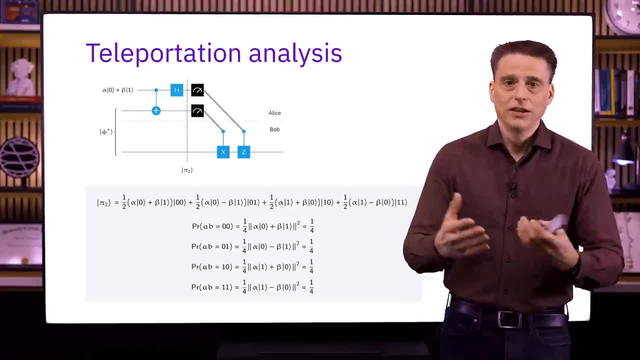 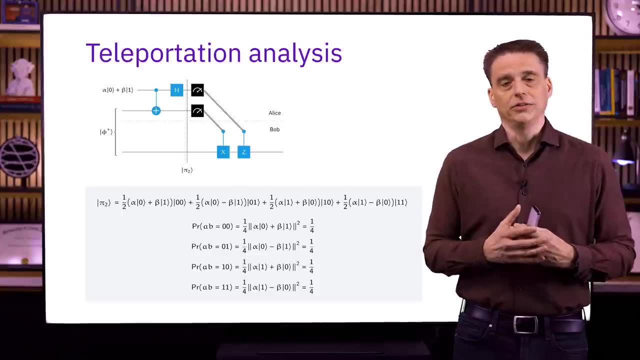 which we get by squaring one-half times the absolute value squared of alpha plus the absolute value squared of beta, which is one, And so we get one-quarter in each case, And so we get one-quarter in each case. It's quite important, in fact, that the probabilities of these different outcomes don't depend in 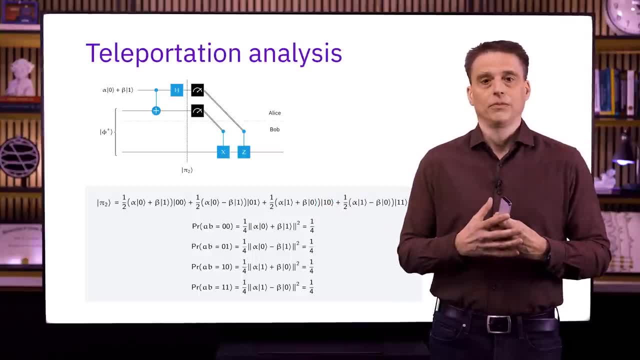 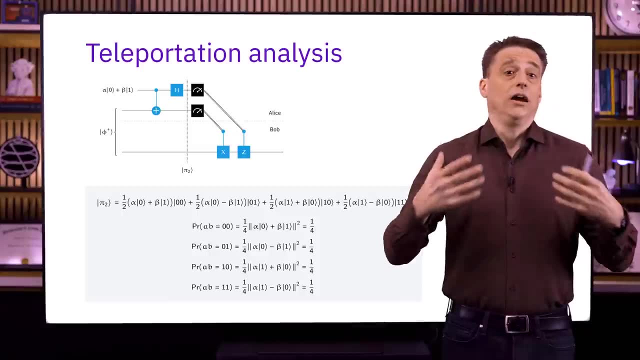 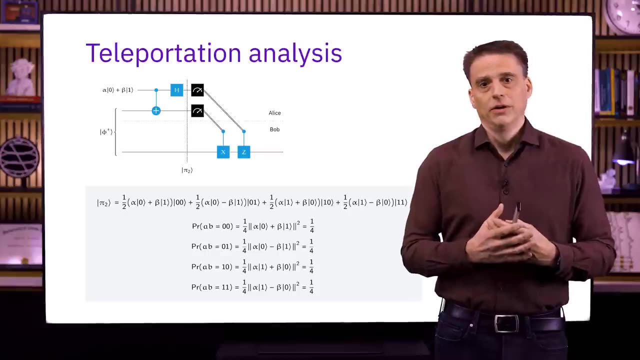 any way on the qubit that Alice wants to transmit. We couldn't have that. an arbitrary state comes in up here and comes out down here, and yet a measurement revealed information about that state. If you want to gain information about an arbitrary quantum state, you're going to have to disturb. 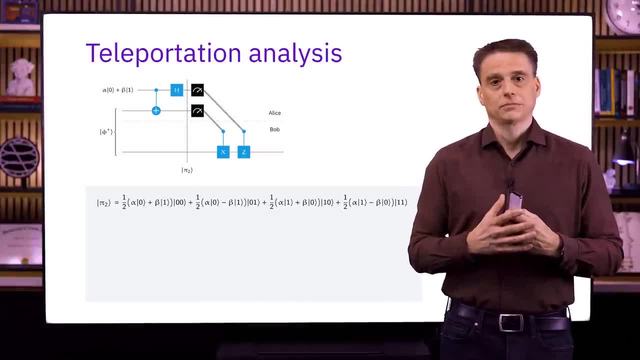 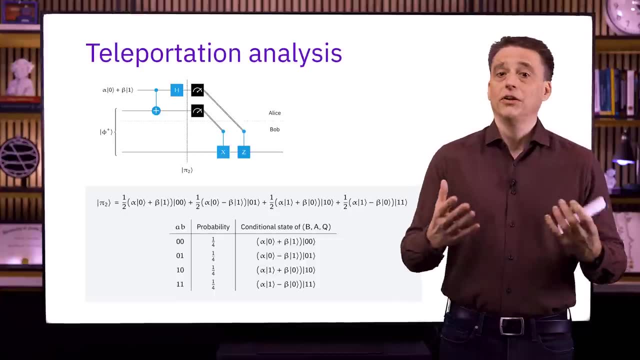 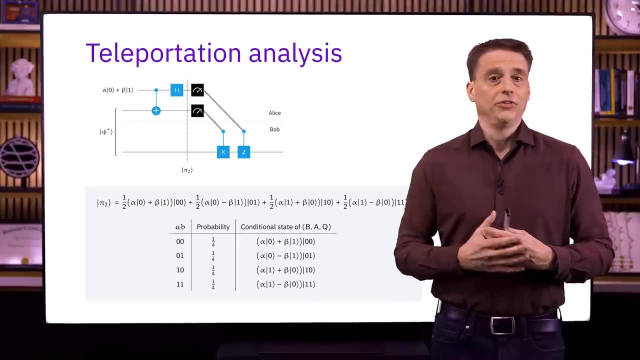 that state in general. Here's a table that describes not only the qubit that Alice wants to transmit but also the probabilities of the different outcomes, but also the state of the three qubits together, conditioned on each possible measurement outcome. We get this by normalizing the vectors tensored to the different standard basis states. but 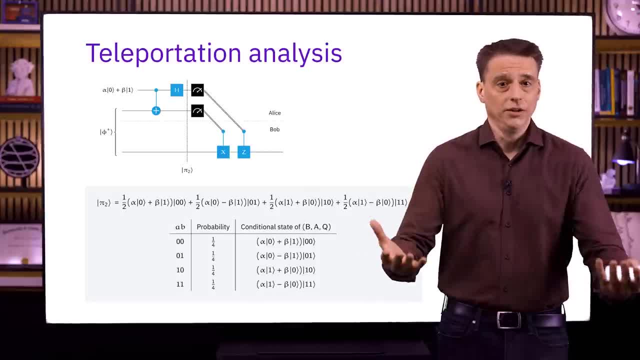 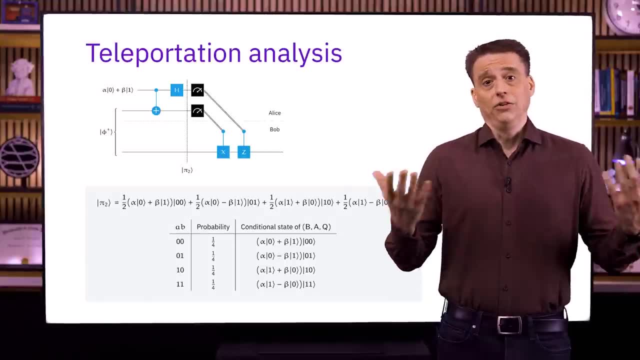 that's easy. in this case We just eliminate the factor of one-half to get a unit vector. So what we have immediately after Alice measures is that Alice has two uniform random bits, and that's it In particular. she no longer has a unit vector. 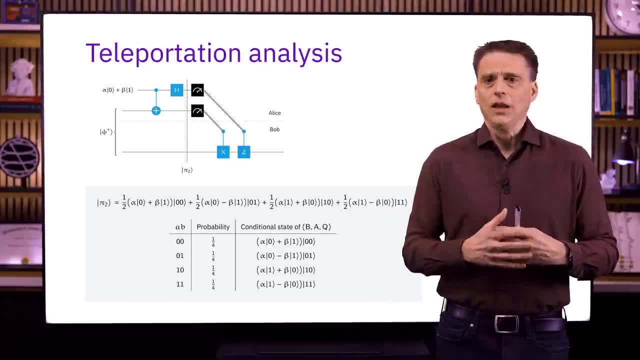 So what we have immediately after Alice measures is that Alice has two uniform random bits and that's it. Alice has the original state and she doesn't have any information about it. She just has random bits. Bob's state now does depend on alpha and beta, as well as on the measurement outcomes. 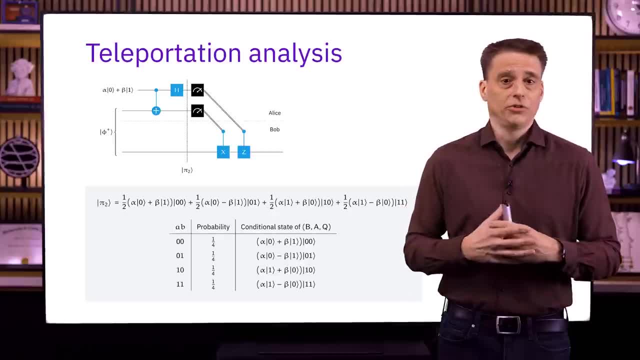 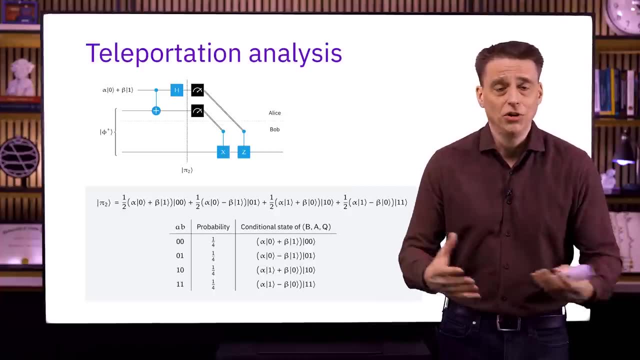 If we imagine momentarily that Alice hasn't yet sent the measurement outcomes, so that Bob doesn't know what the measurement outcomes are, then he wouldn't be able to gain any information about alpha and beta from measuring his qubit. These four possibilities that we have right here are sufficiently scrambled to your advantage. 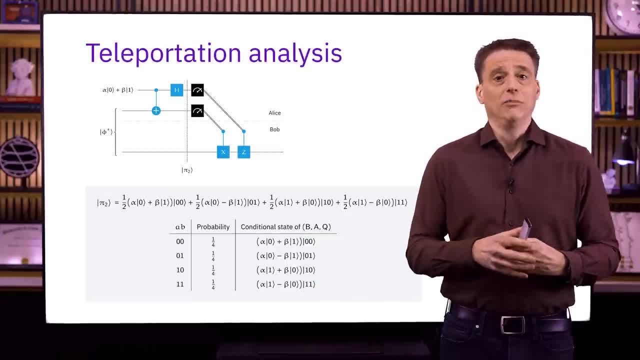 So we can now get the qubit, We can then delete the data and we can keep the business going. And now we're going to have a new elements under measurement so we can have some changes to the values we want to see. 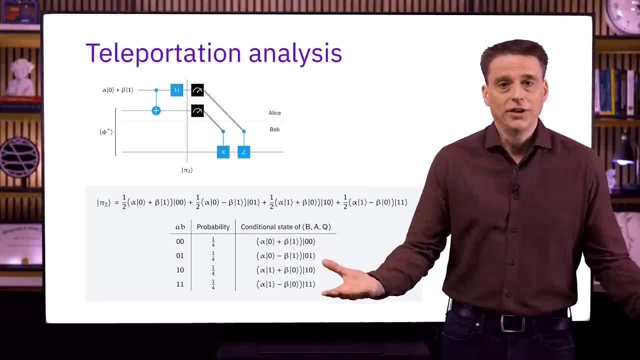 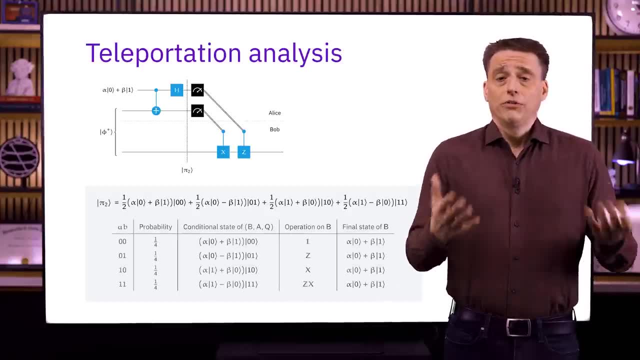 If we look at the library's count of the data- we keep the data- then we have something like 7-385-800-000.. But that doesn't mean that Alice can't transmit data to Bob without sending anything at all. But of course Alice does send the measurement outcomes to Bob. 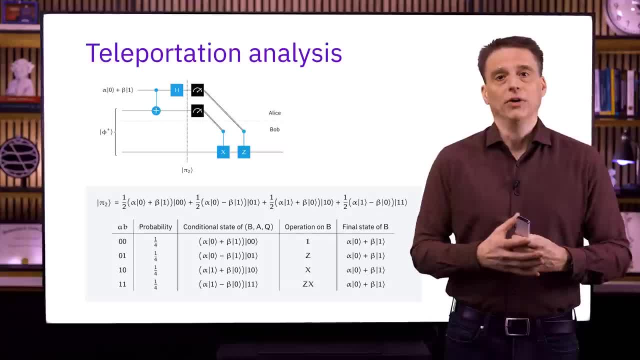 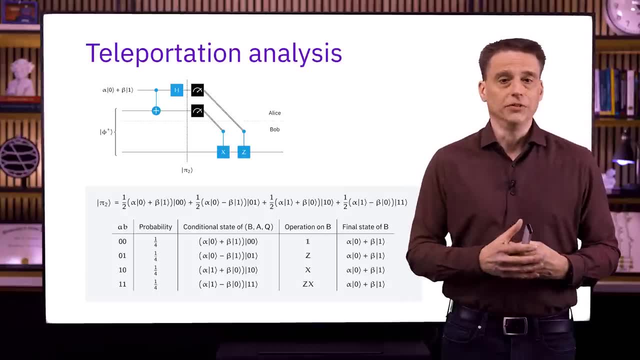 So let's expand the table to see what happens when Bob performs his operations In this column. right here we have all the different operations that Bob can perform In this column. we have the different operations that Bob can perform, operations that Bob effectively performs for each of the possible outcomes of the 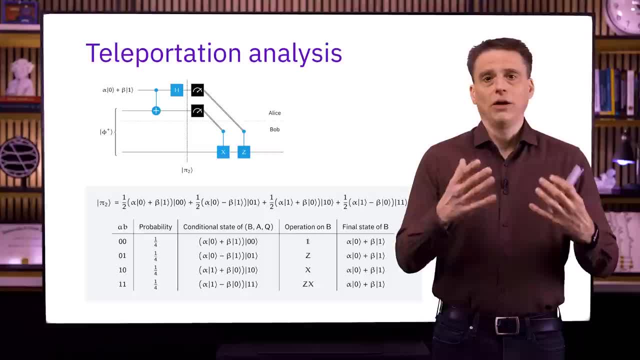 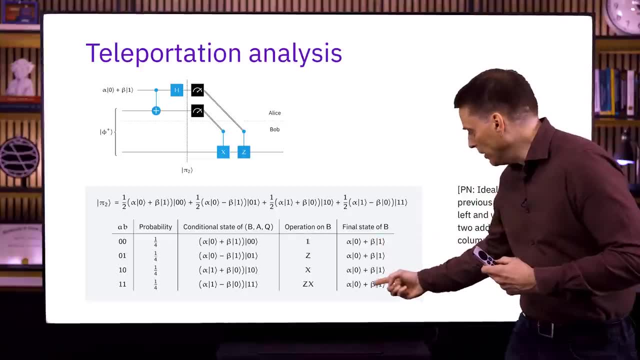 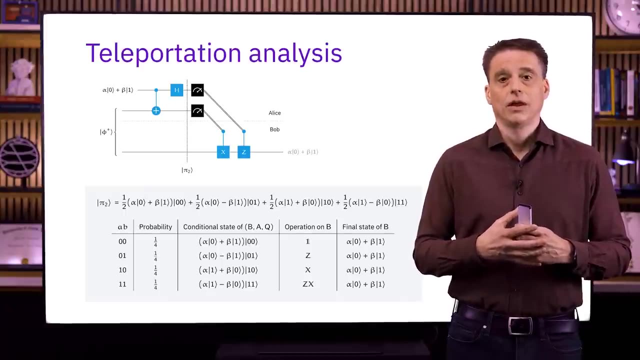 measurements, like we observed before, And if we go one by one and we apply that operation to Bob's qubit, which is the first one B, we see that we get the same outcome in all four cases and that outcome is the original state. So the 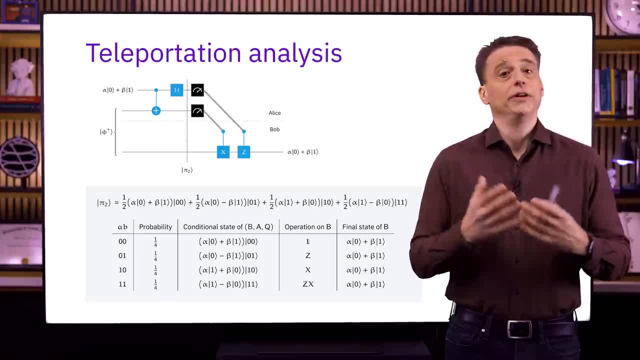 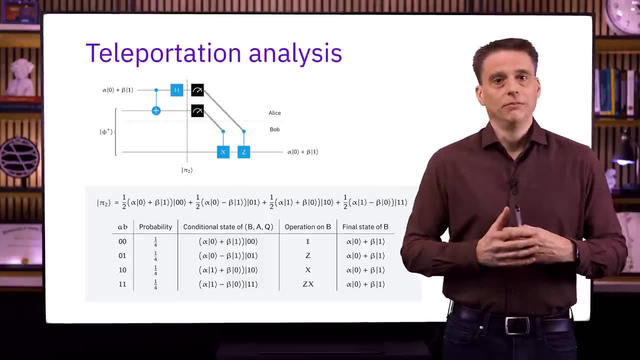 original state of the qubit Q has been successfully teleported into B. If Bob wants to rename his qubit and call it Q at this point, he's certainly welcome to do that. but the point is that now he holds the original state that Alice had. 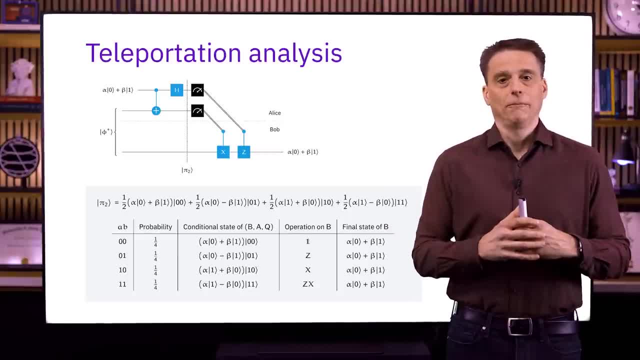 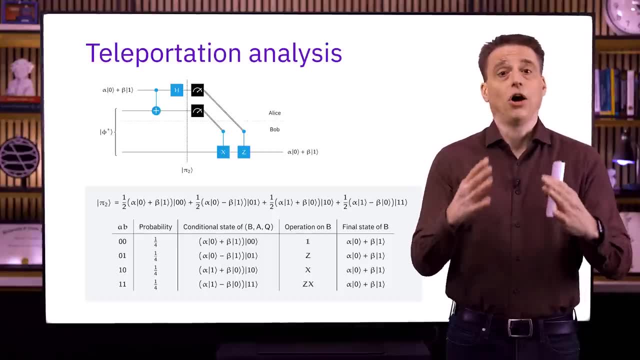 and, of course, by necessity, Alice doesn't have it anymore. Notice also that the e-bit has effectively been burned up through this process. Teleportation has a cost, and the cost is one e-bit and two classical bits of communication. And when? 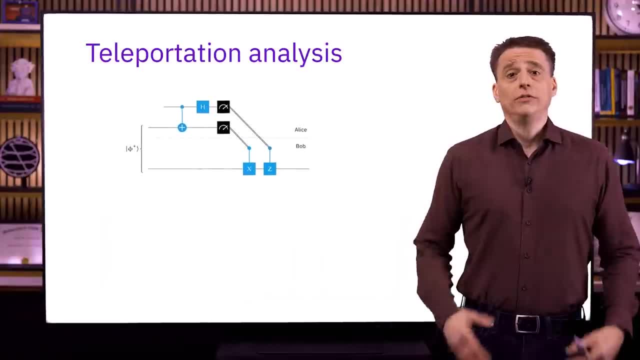 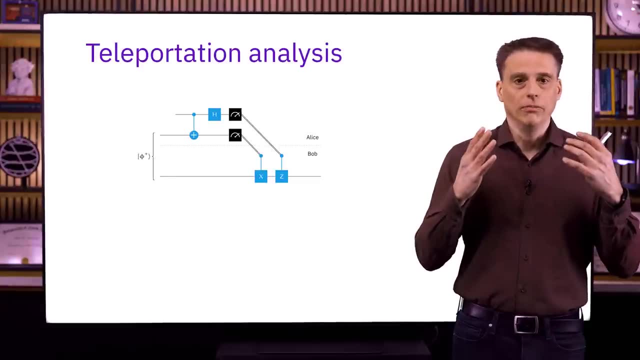 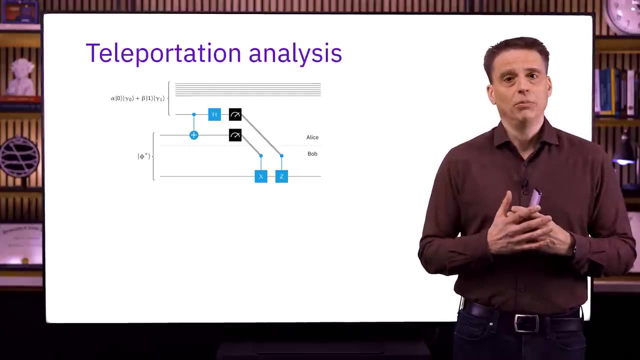 the protocol is over. the e-bit is gone. We've now established that the teleportation protocol works correctly, under the assumption that the top qubit is in a quantum state of the form alpha times ket zero plus beta times ket one. But what happens if the top qubit is entangled with some other system, such as: 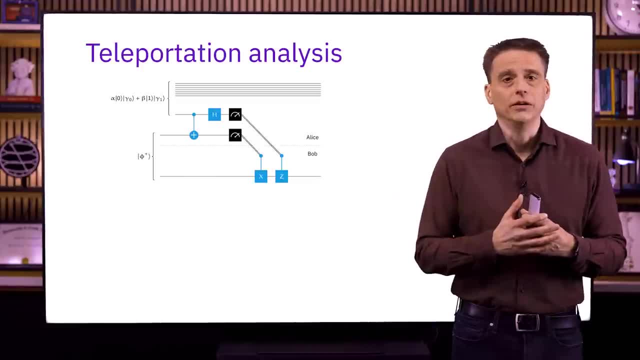 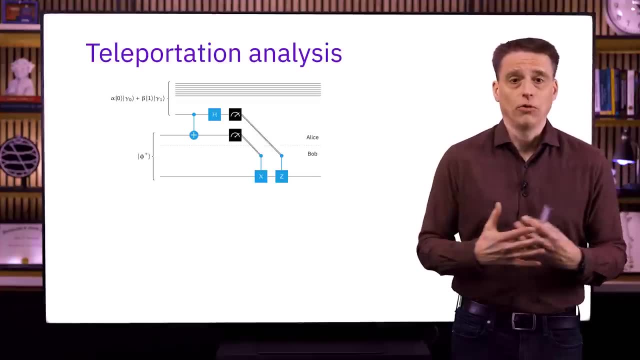 one or more additional qubits as we have here on the screen. We might wish to use teleportation under such circumstances. Maybe Alice and Bob actually plan to perform teleportation 100 times so that Alice can transmit the e-bit to the top qubit. 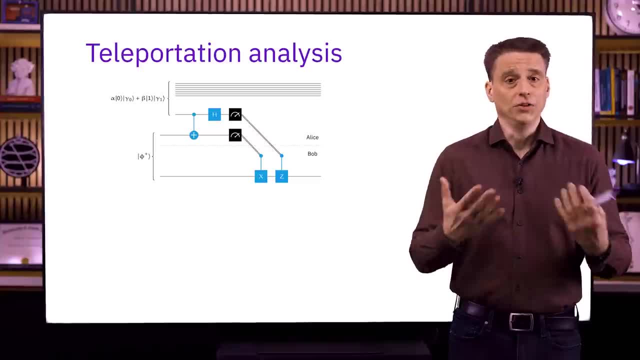 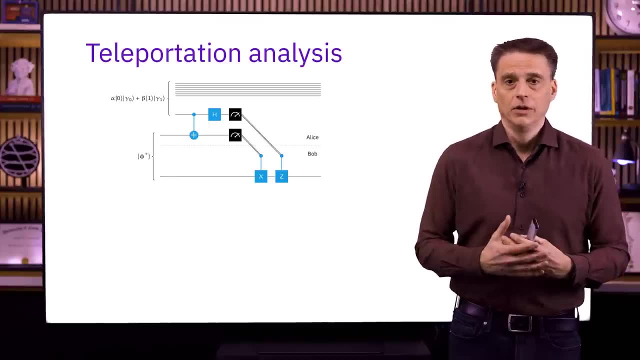 Maybe Alice can transmit some 100-qubit quantum register to Bob, one qubit at a time. Or maybe these additional qubits aren't even in Alice's possession at all and somebody else has them. Maybe Alice doesn't even know that they exist. The 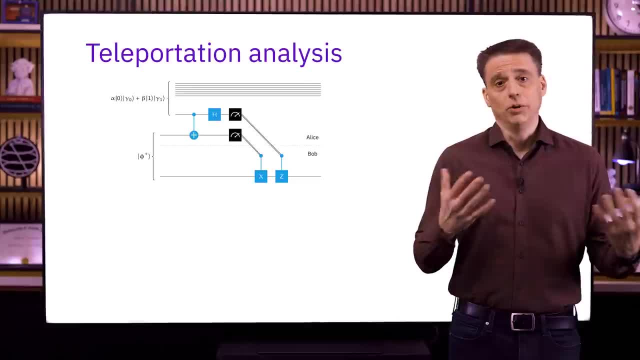 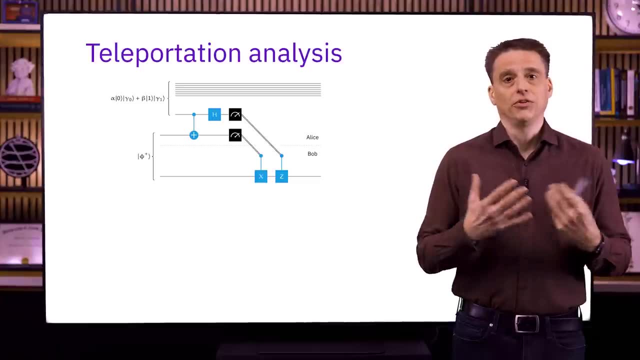 question is: does teleportation still work even though the qubit being teleported is entangled with another system? Here the state of the qubit Q, together with the additional system that we're considering, is expressed as you can see right up here, where gamma zero and gamma one are unit vectors. 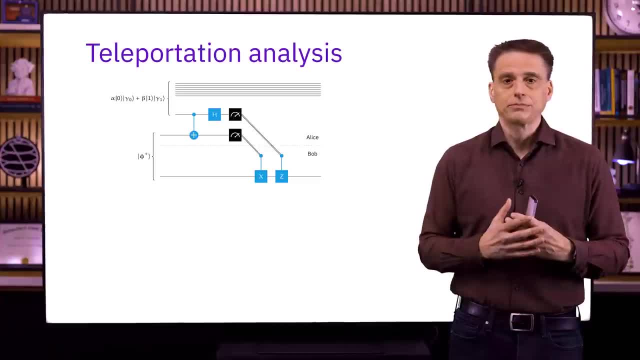 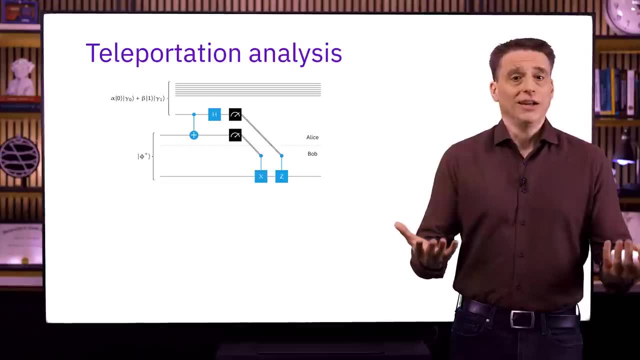 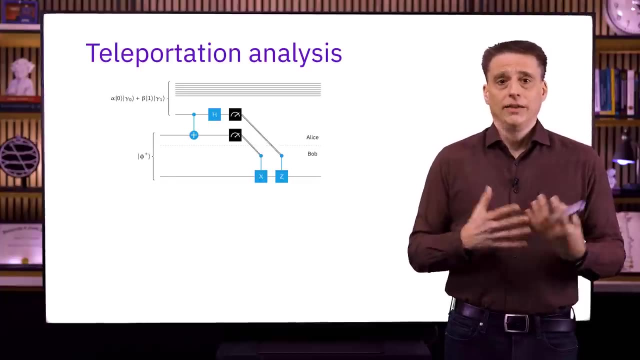 Representing quantum states of this additional system. We can always write an arbitrary state of the combined system in this way. We don't actually even need alpha and beta here, but if we include them, then we can take gamma zero and gamma one to be unit vectors and that'll make the connection to the simpler case. 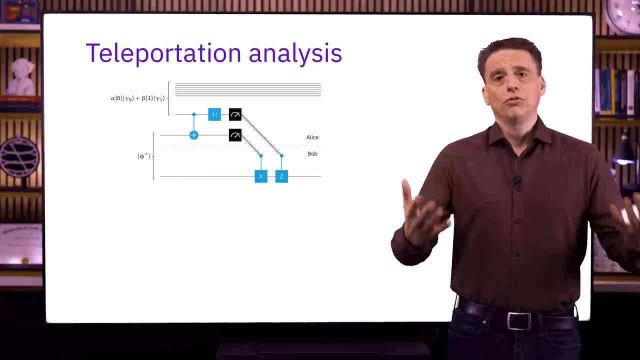 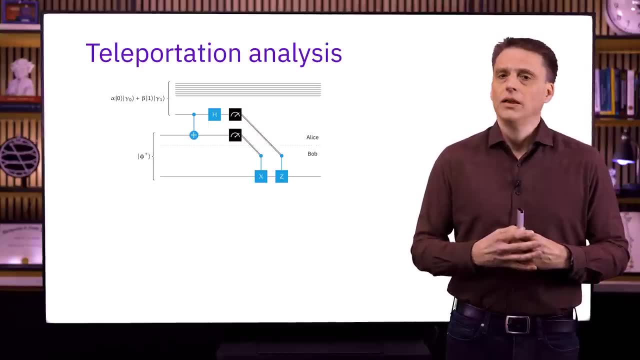 we've already considered more transparent. We can go through a similar analysis to the one that we already went through, but where we also keep track of this additional system. It's a little bit messier because we have the additional system, but the idea. 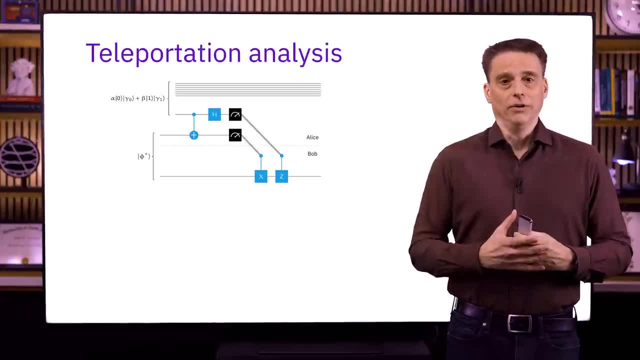 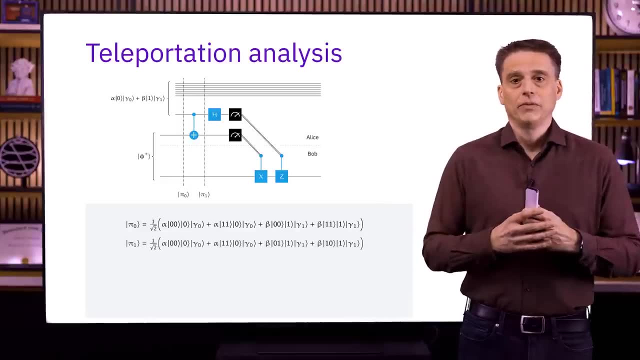 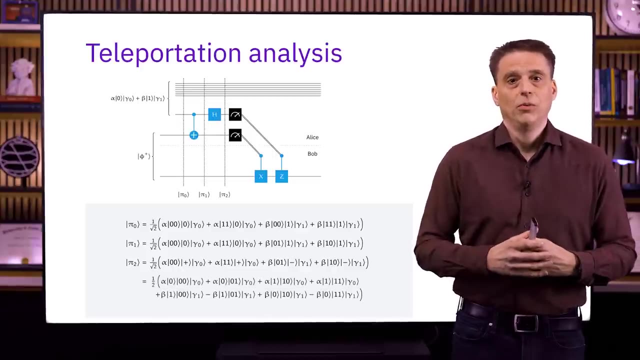 is exactly the same. Here's a very quick summary. This is the initial state. Here's the state after the controlled NOT- gate and here's the state after the Hadamard operation. If we expand these things out, we can express that state, as you can see. 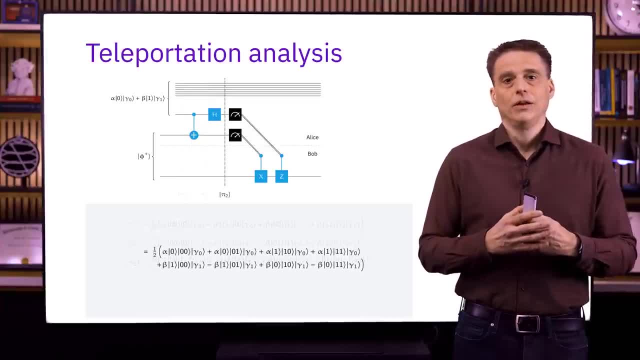 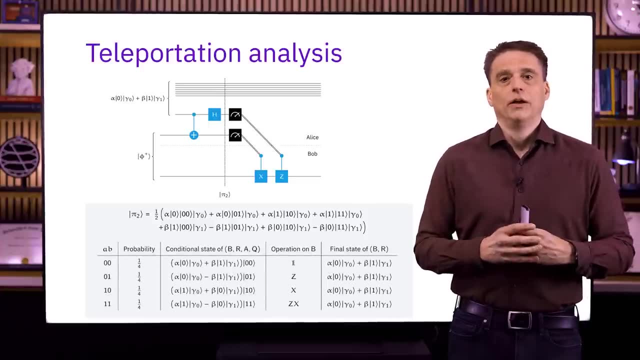 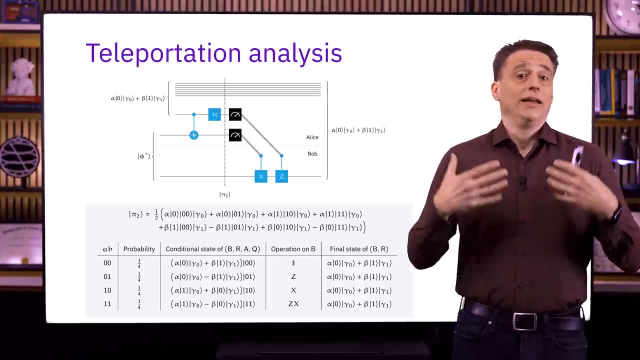 right here. That's the state immediately before Alice's measure, And if we go through the possibilities just like before and we consider what happens when Bob applies whatever operation he's supposed to apply, then we find that indeed, the correct state comes out and the protocol works as expected. 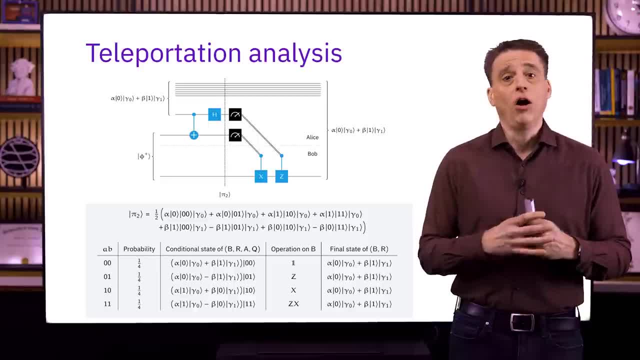 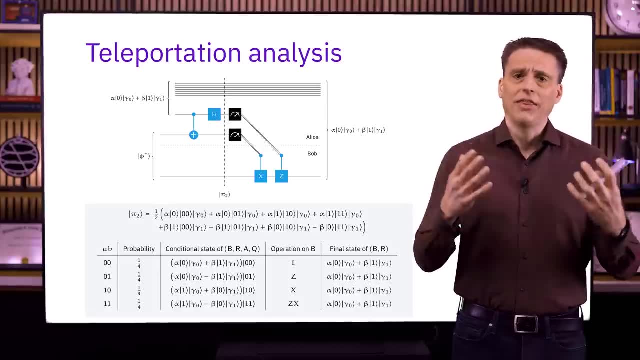 In this table. by the way, we're using the letter R to refer to this additional system, and you can see that we're using a pretty simple trick, which is to decide that we would rather, at least momentarily, order the systems as B, R, A. 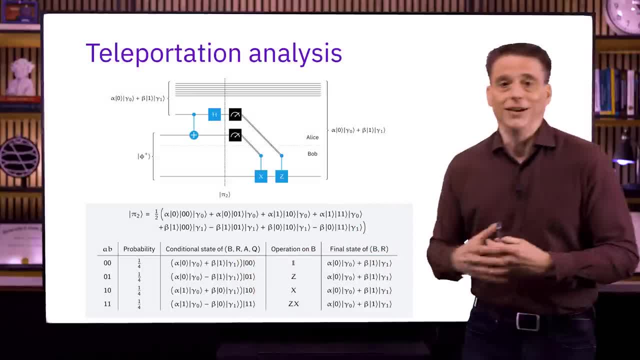 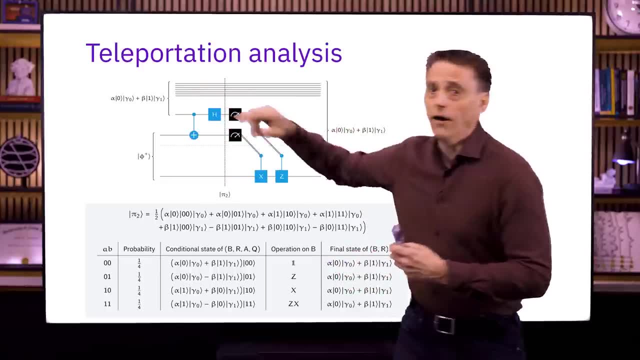 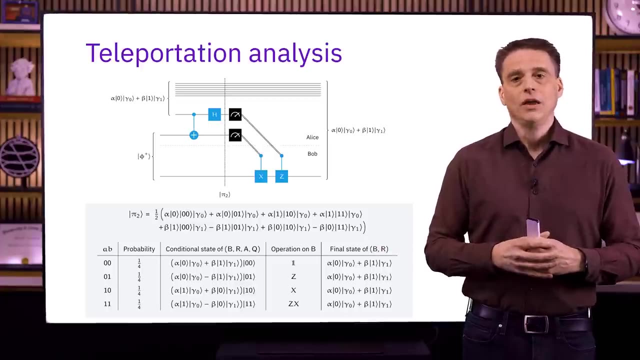 Q because that's more convenient for writing the states right here. According to the diagram, the systems should be ordered as B, A, Q, R, but as long as we make it clear, we can choose a different ordering. that's more convenient In a. 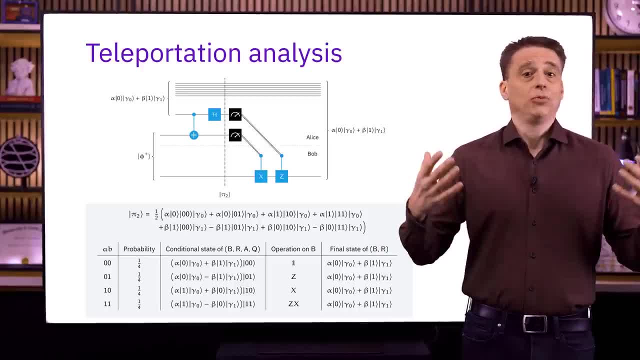 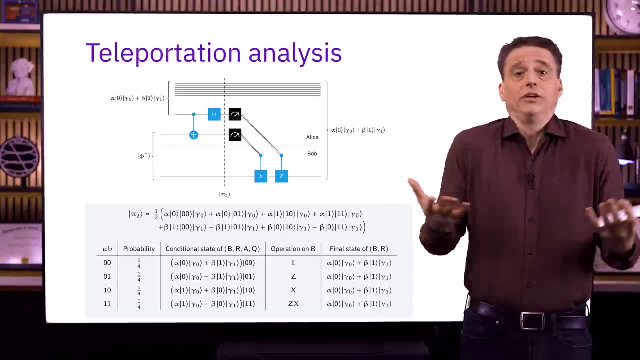 nutshell, everything that's happening in this analysis is the same as what happened in the simpler analysis, but we happen to have these additional vectors- gamma 0 and gamma 1, that basically come along for the ride. So let's take a look at what happens when we order the systems as B, A, Q, R. but we happen to have these additional vectors- gamma 0 and gamma 1, that basically come along for the ride. 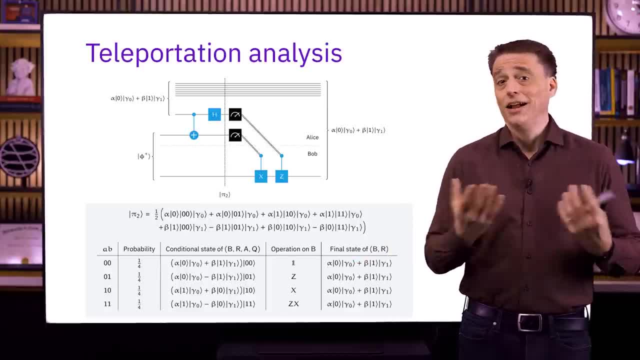 So let's take a look at what happens when we order the systems as B, A, Q, R. but we happen to have these additional vectors- gamma 0 and gamma 1, that basically come along for the ride. We always have gamma 0 when there's a factor of alpha and gamma 1 when there's a factor 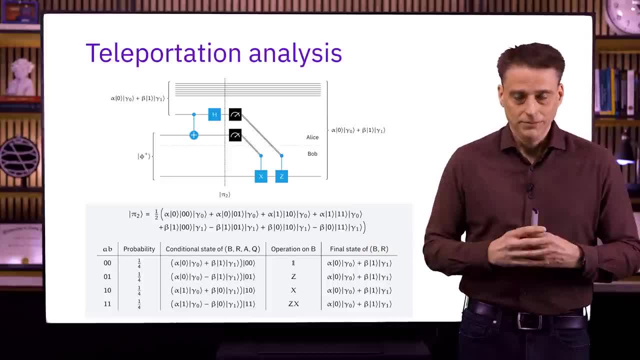 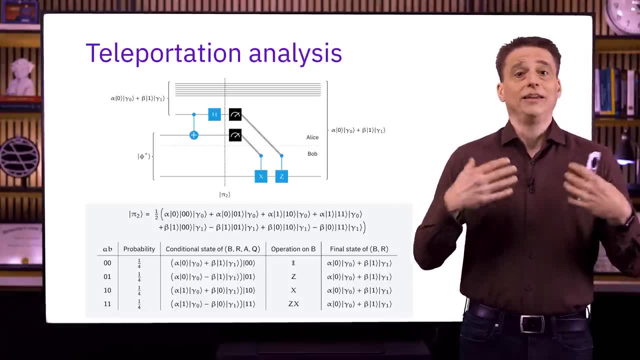 of beta and at the end of the day, it all works out correctly. This is actually not at all surprising. We have a physical process that acts like the identity operation on a qubit in an arbitrary quantum state, and there's only one way. 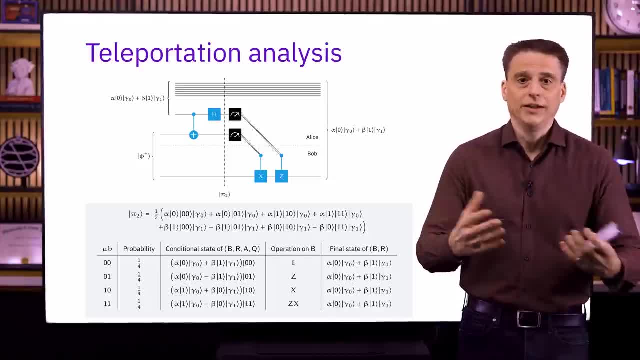 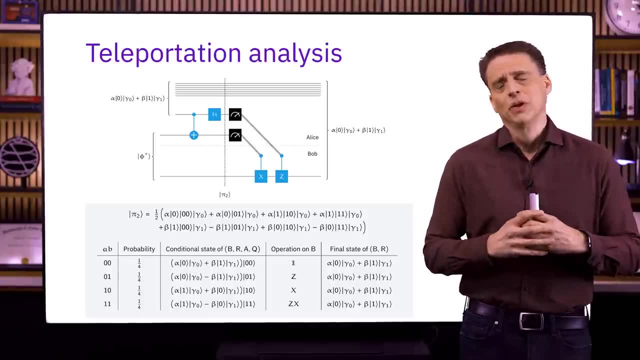 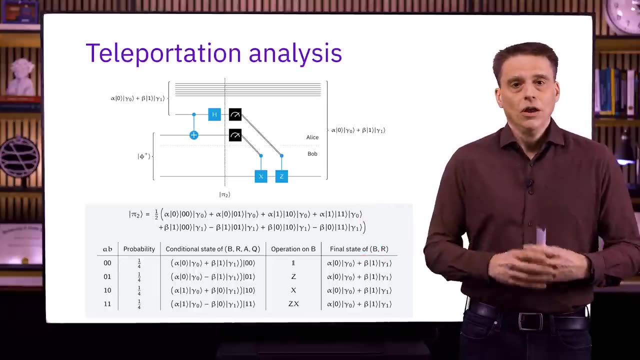 that that can happen and that is that the operation is the identity operation. That's a little bit easier to explain using the general formulation of quantum information, but the point is that by linearity, we really didn't need to go through this additional analysis. 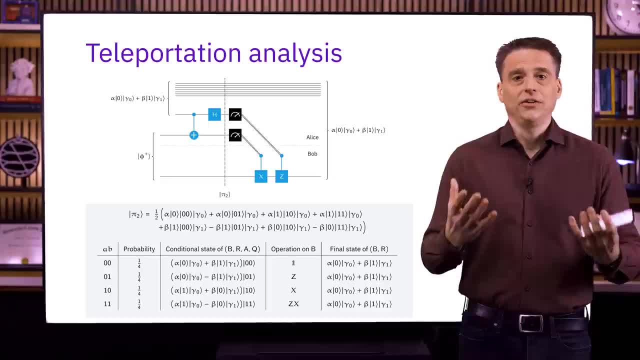 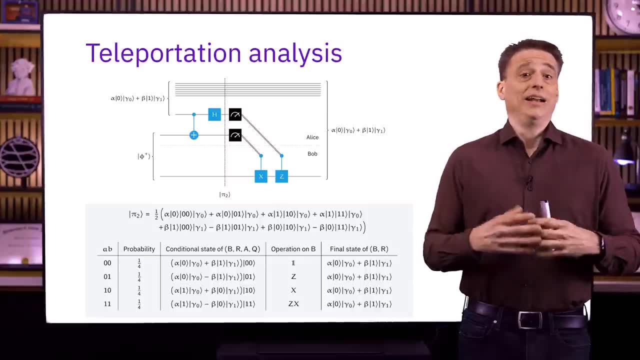 Once we know that teleportation works correctly for a single qubit in isolation, we can conclude that there's only one possible thing that can describe what the protocol does, and that is that it implements the identity operation where a qubit comes in, right here and it. 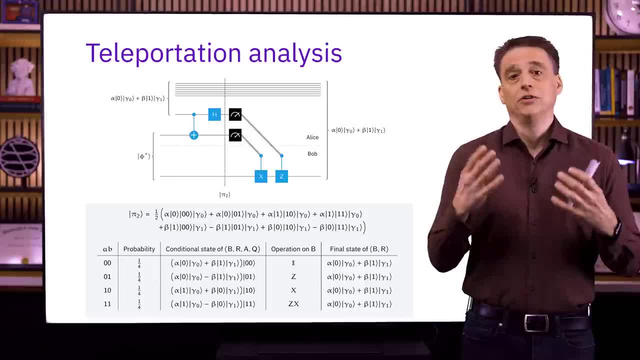 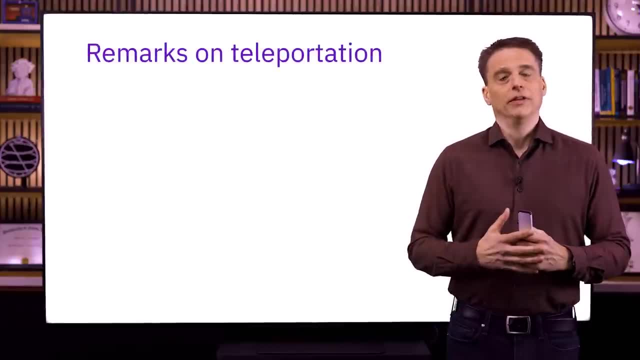 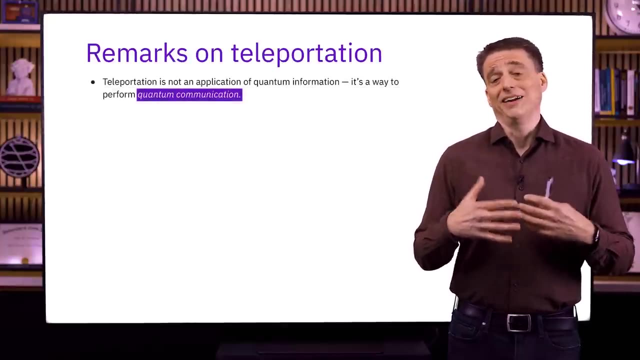 comes out right here, effectively acting as a perfect noiseless quantum channel. Just a few quick remarks about teleportation before moving on to the second example of the lesson, which is superdense coding. First, I think it's important to clarify that teleportation is not an application of 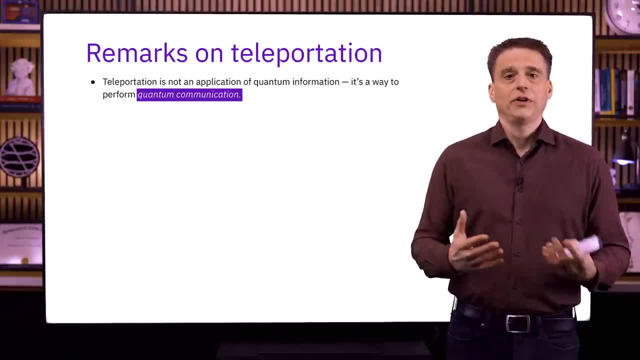 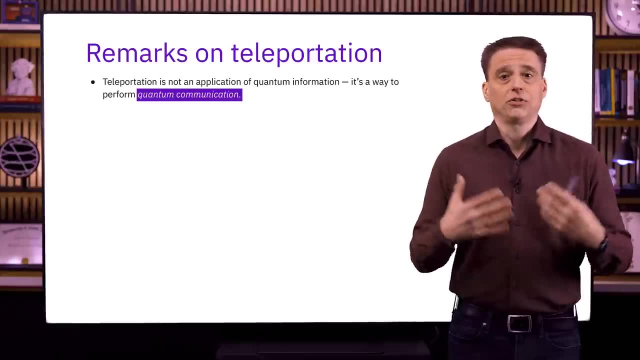 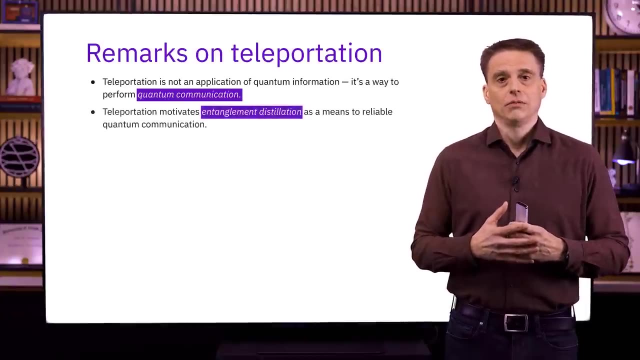 quantum information. it's a protocol, and specifically it's a protocol for performing quantum communication. In order for teleportation, as I've described it, to be useful, there has to be some reason for performing quantum communication. Second, it's reasonable to speculate that teleportation could one day become a standard. 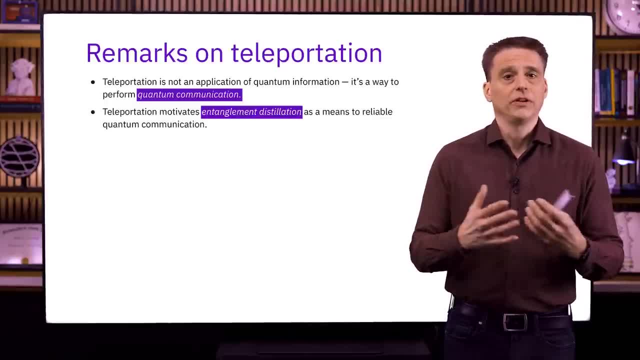 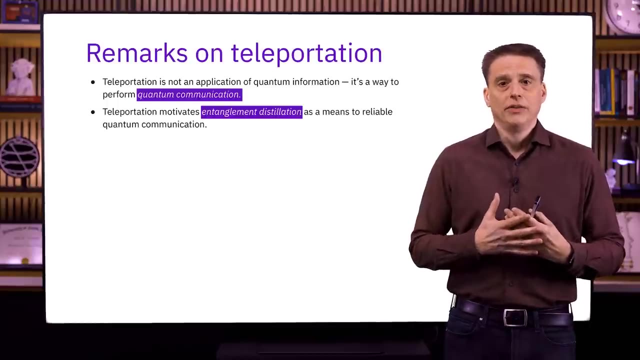 way to communicate quantum information, and specifically a process known as entanglement distillation might potentially be used as a way to communicate qubits reliably. If Alice and Bob know they're going to be communicating quantum information, or they have the need to communicate quantum information, then this process of entanglement distillation- 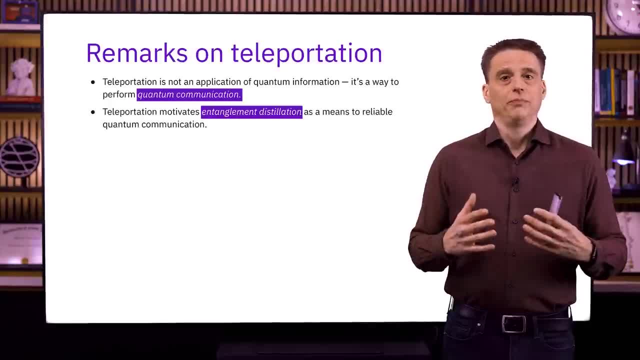 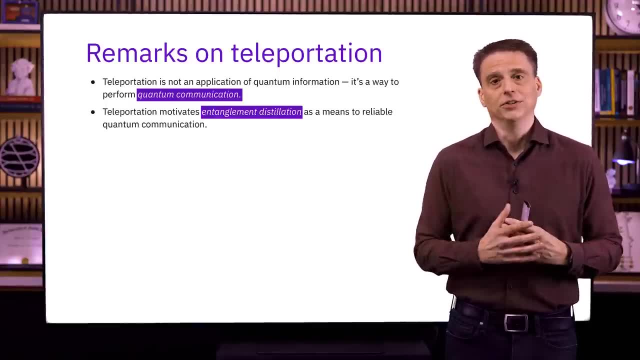 could be used to convert a larger number of non-quantum information into quantum information. Thank you. So the idea is that we could convert the noisy ebits into a smaller number of high-quality ebits that could then be used for noiseless or near-noiseless teleportation. 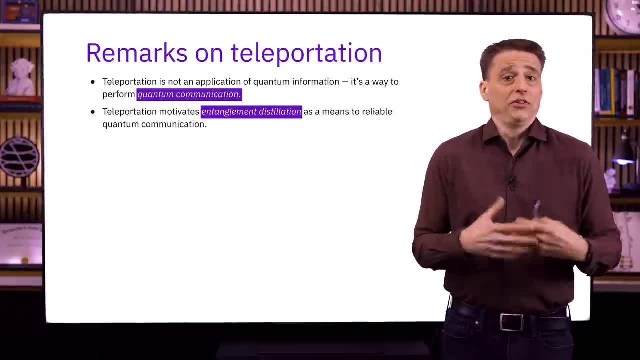 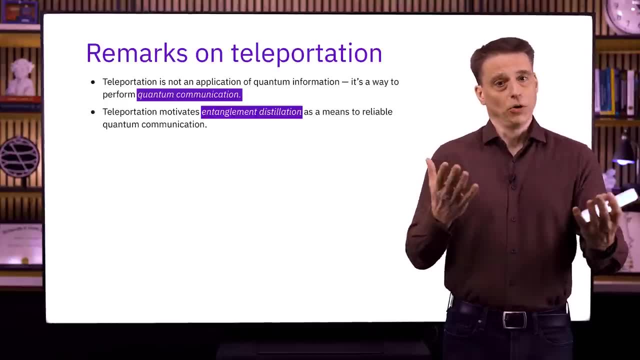 The idea is that the process of entanglement distillation isn't as delicate. in some sense, We could accept losses and if it doesn't work out, then we could just try it again, whereas the actual qubits that we would like to communicate might be considered much more. 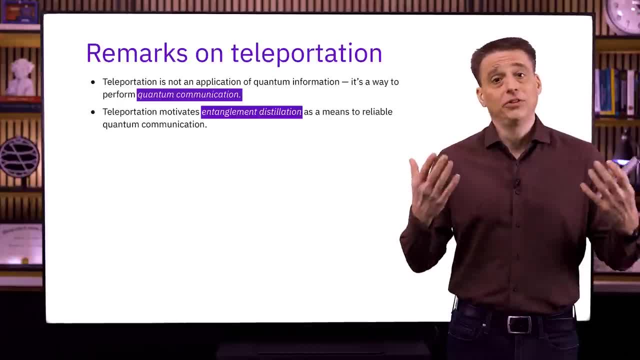 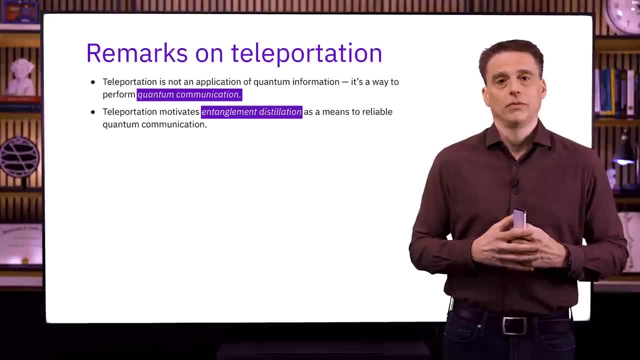 precious difficult to hypothesize situations in which teleportation could be a very practical way to communicate qubits. And the final point concerning teleportation is that the idea behind teleportation and the way that it works is quite fundamental in quantum information and computation. Teleportation is really a cornerstone of quantum information theory, and variations on the idea also often come up. As just one example, there are proposals for implementing different quantum gates using teleportation, but where different initial states and measurements are chosen so that the outcome is to apply a chosen operation rather than to communicate. 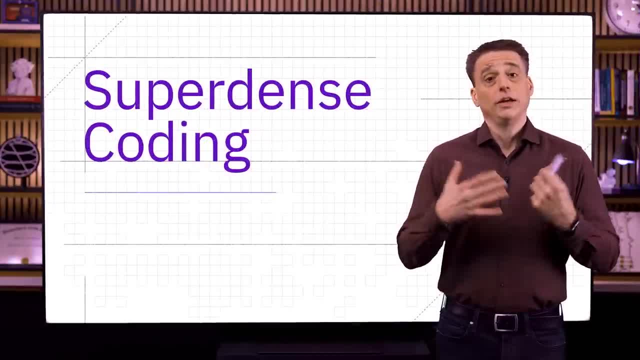 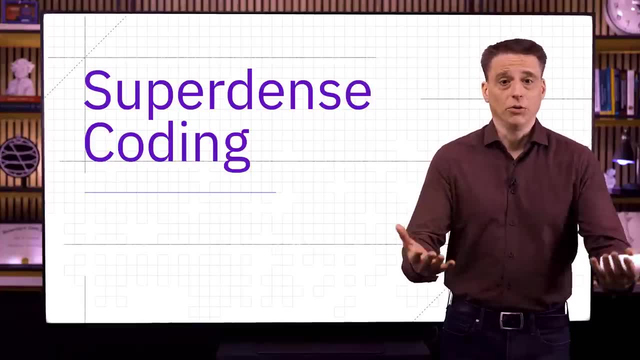 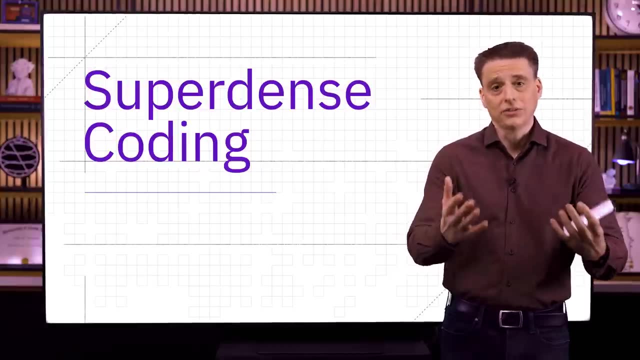 The next example is superdense coding. Like quantum teleportation, superdense coding is a protocol and what it accomplishes is complementary to teleportation. Whereas teleportation is a protocol, superdense coding is a protocol. Transmission allows one qubit to be transmitted using an e-bit and two classical bits of communication. 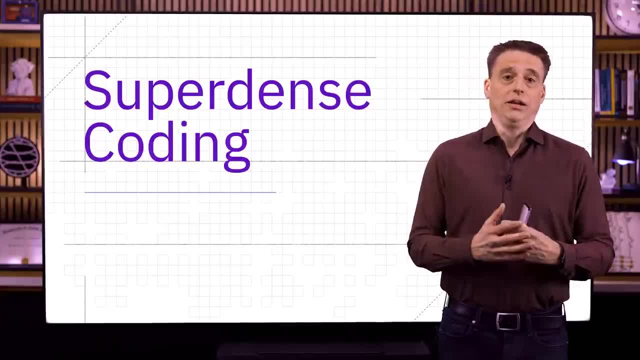 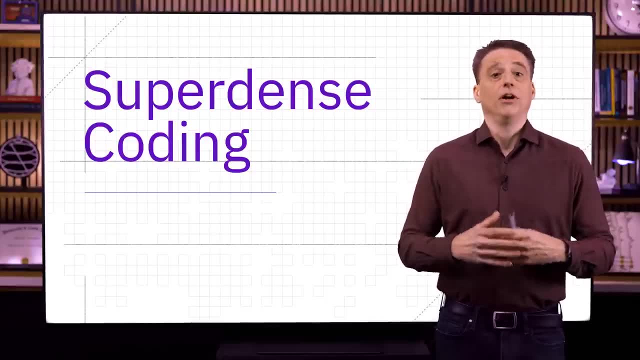 Superdense coding allows two classical bits to be transmitted using an e-bit and one qubit of quantum communication. So, in short, superdense coding allows for the transmission of classical information, And the reason it's called superdense coding is that it allows for two classical bits of 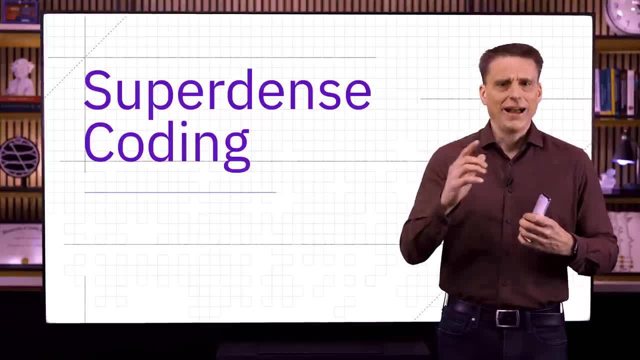 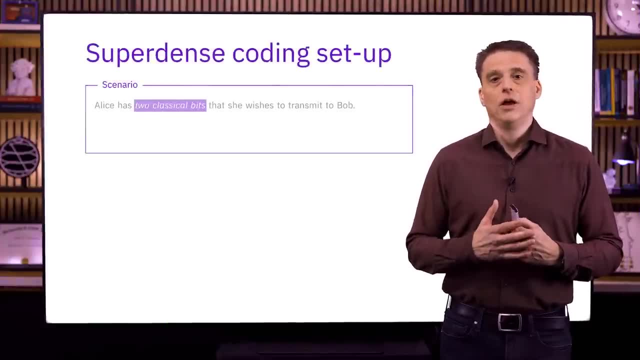 communication to be packed into a single qubit, But we have to burn an e-bit to accomplish this. Subtitles by the Amaraorg community. Here's a more precise explanation of the setup. Once again, we have Alice and Bob, where Alice is the sender and Bob is the receiver, and 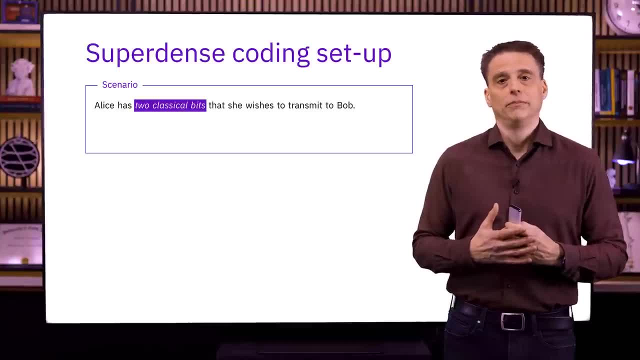 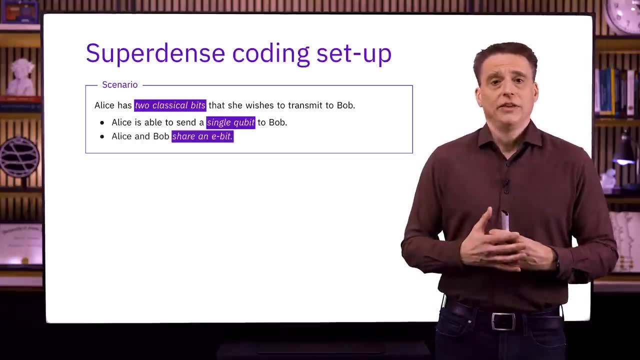 this time, Alice has two classical bits that she wants to send to Bob. Alice is able to send Bob a single qubit, and Alice and Bob share an e-bit that they can use to help them to accomplish their task, which is for Bob to receive the two classical. 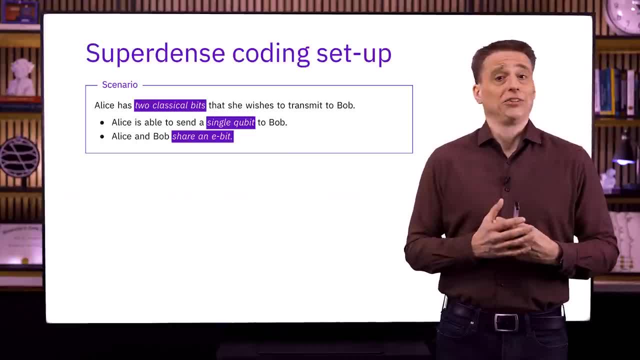 bits. Now there's a sense in which this task may seem low-key, but it's not, because Alice and Bob share an e-bit that they can use to help them to accomplish their task, which is for Bob to receive the two classical bits. 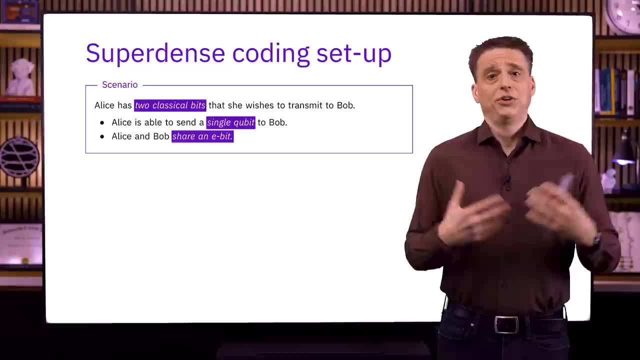 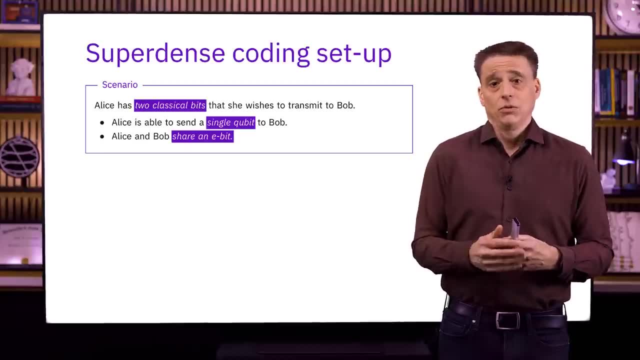 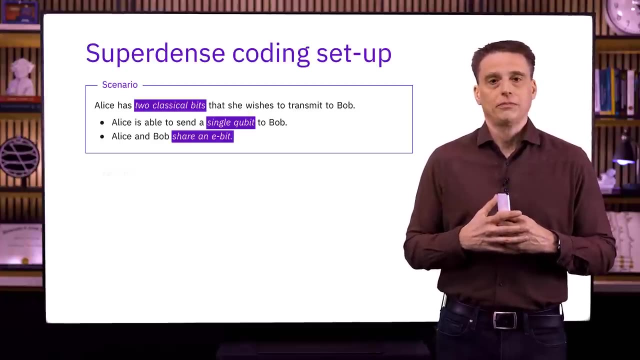 This is less interesting than the task that teleportation accomplishes, particularly if we view that sending qubits is significantly more difficult or more challenging than sending classical bits, which is a pretty reasonable point of view, But it is definitely interesting that it's possible to do this. 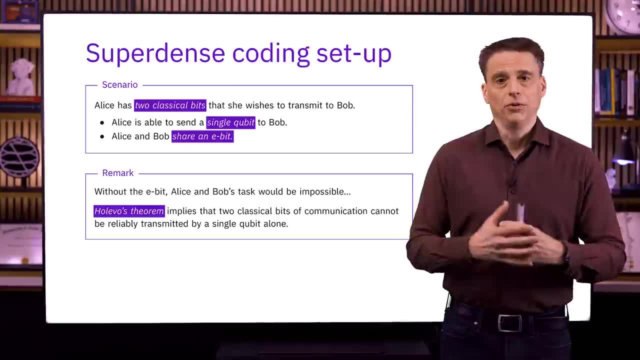 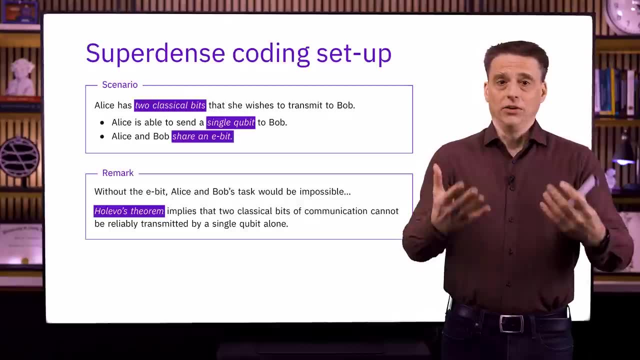 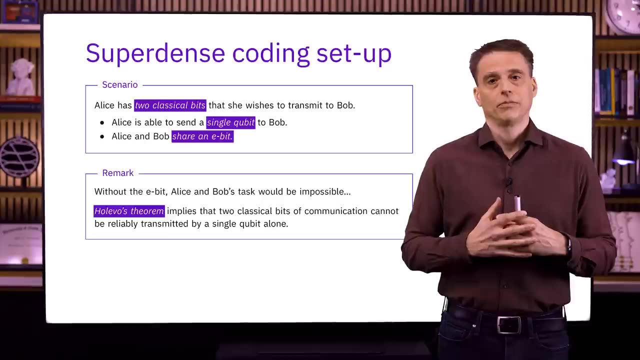 One reason why it's interesting is that it is in fact impossible to accomplish this task of transmitting two classical bits of information using a single qubit without making use of the e-bit. We know this because of a famous theorem known as Holowohl's theorem. 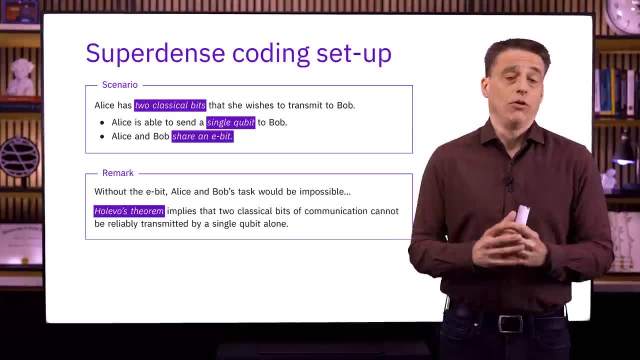 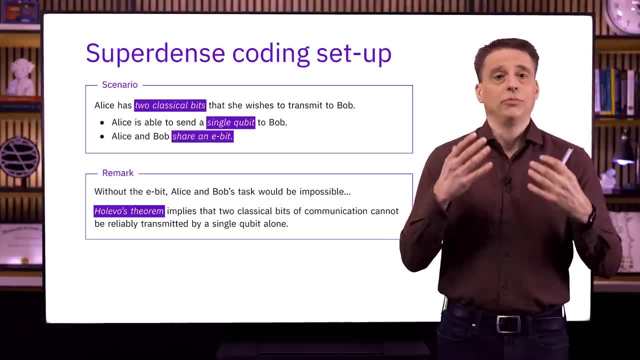 Holowohl's theorem is more general than this and the precise statement of Holowohl's theorem is a bit technical and it requires some explanation. but one implication of it is that you cannot transmit any number of classical bits of communication using fewer qubits of quantum communication. alone. If you want to reliably transmit two classical bits of information using qubits and you don't have an e-bit to make use of, you're going to have to send two qubits, so they might as well store the bits that you want to transmit. 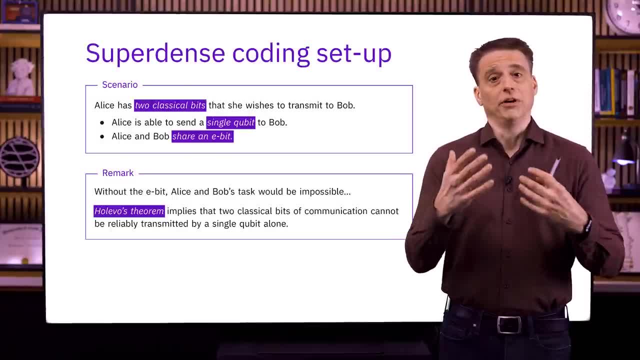 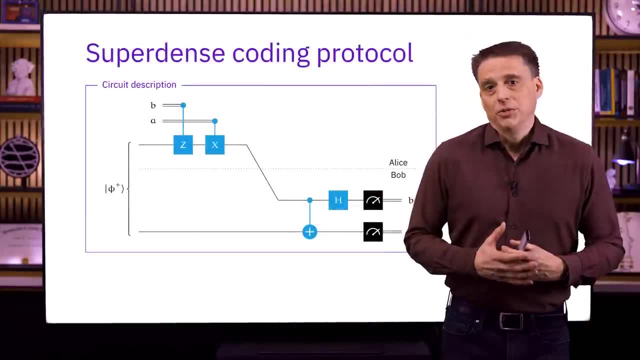 Another reason why superdense coding is interesting is because of the close complementary relationship it has to teleportation, and we'll come back to this a little bit later. Here is a quantum circuit description of the superdense coding protocol. For this one I won't list out all the steps, but instead we'll just stick with the circuit. 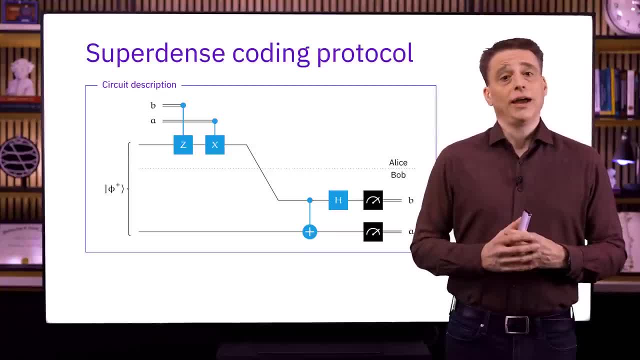 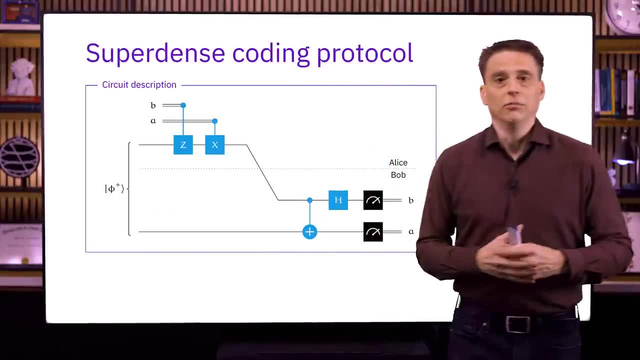 diagram: description. As you can see, we again have Alice and Bob, where Alice is on the top and Bob is on the bottom. Here is the e-bit that's initially shared between Alice and Bob, which has somehow been established prior to the protocol being run. 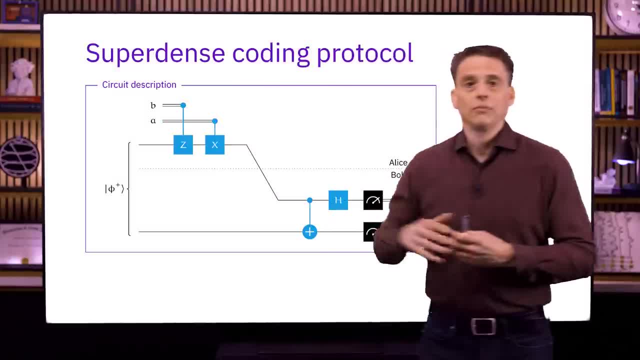 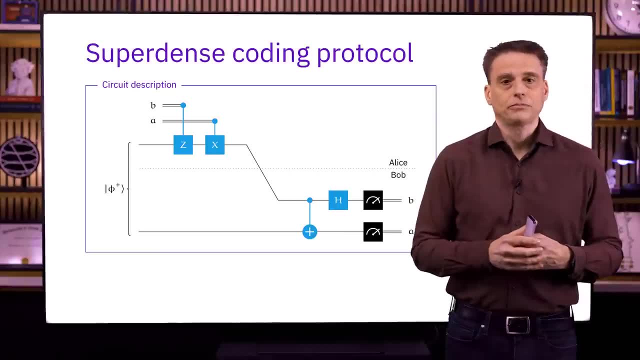 Alice has two classical bits, A and B, which you can see up here, and, through the protocol that the circuit describes, these two classical bits will end up in the hands of Bob. There's just one qubit that crosses the line between Alice and Bob. 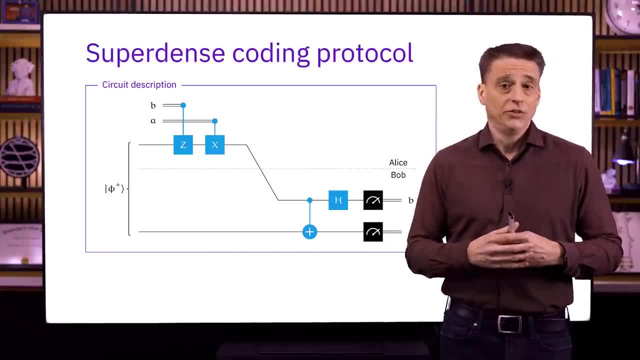 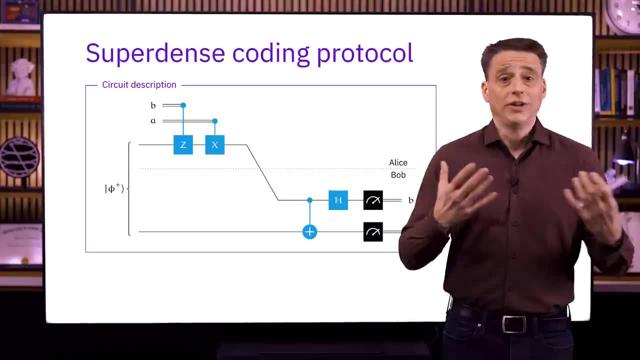 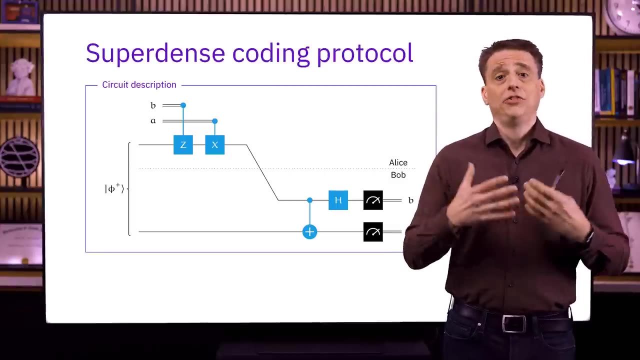 And, of course, there aren't any classical bits being sent. It's the transmission of the two classical bits. that's the point of the protocol. You'll also notice that it has exactly the same components that are used in teleportation. We have a controlled NOT gate, a Hadamard gate, and a Z and an X gate controlled by. 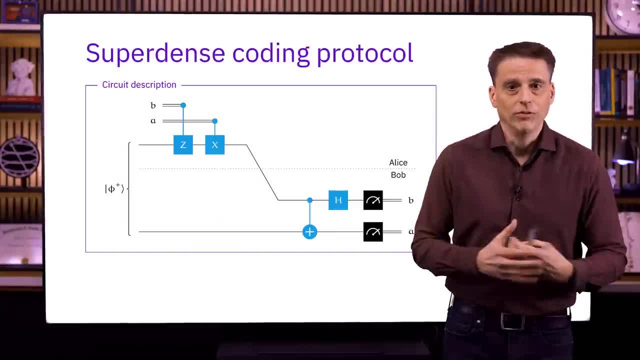 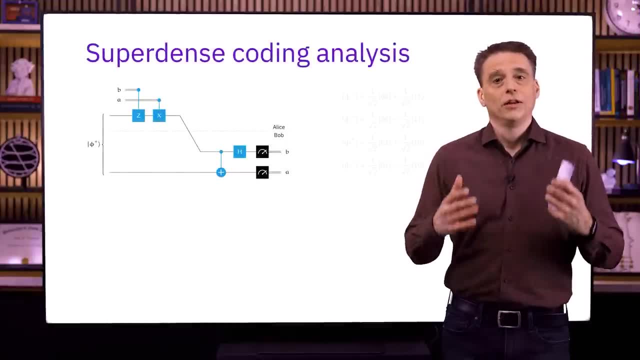 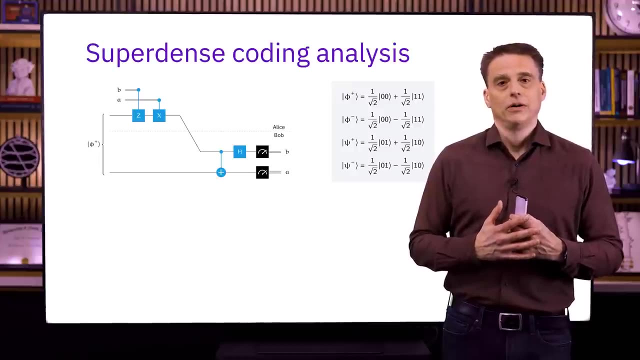 classical bits. They're arranged differently, however, so let's move on to the analysis to see how it works. To analyze how superdense coding works, let's start by looking at a simple example of a superdense coding protocol. Let's start by writing down the Bell basis, which is very much at the heart of the analysis. 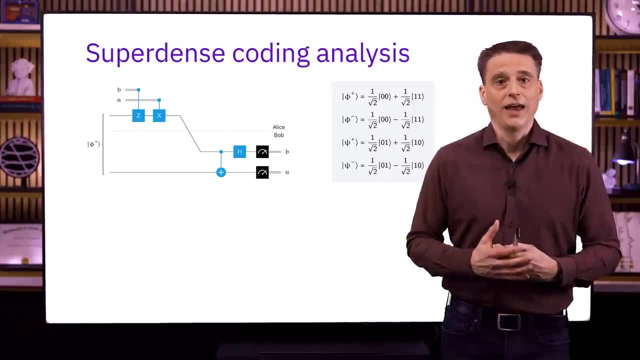 What we're going to do is to first take a look at the effect that Alice's actions have on the phi-plus state, And what we'll see is that Alice transforms this phi-plus state into one of the four Bell states, depending on the bits that she wants to send. 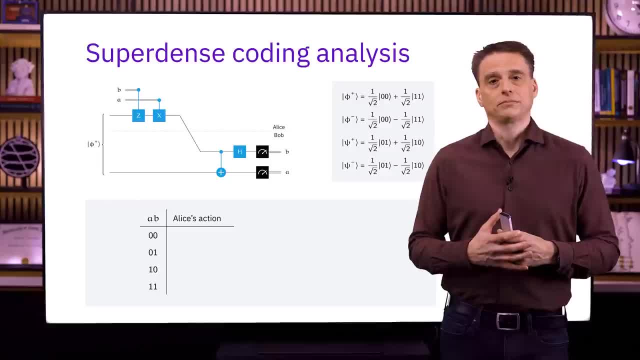 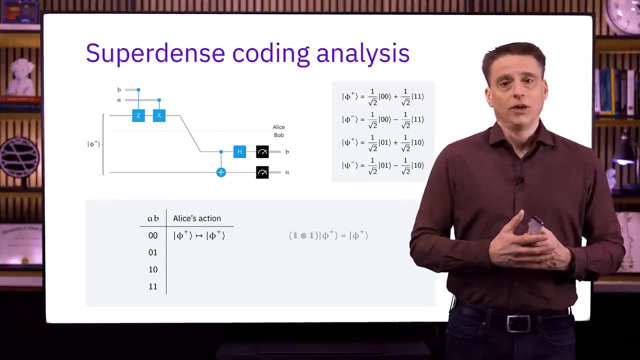 So let's write down a table so that we can keep track of what's going on. First, if A and B are both zero, then neither of the zeroes are zeroes and neither of the Z gate nor the X gate gets applied, So Alice's actions don't do anything, which is to say that phi-plus gets mapped to phi-plus. 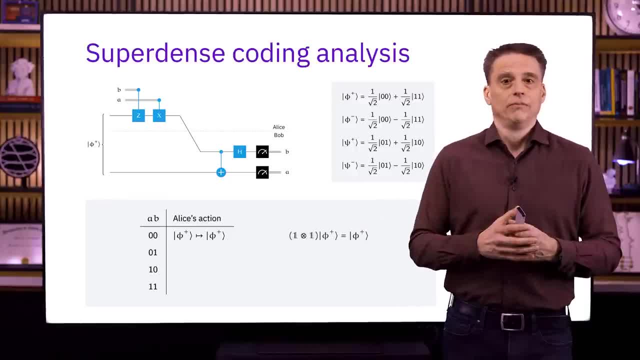 We can also express that as an equation. like you see right here, Nothing happens to Alice's qubit and nothing happens to Bob's qubit. and doing nothing is represented by the identity matrix. Now what happens if A is equal to zero and B is equal to one? 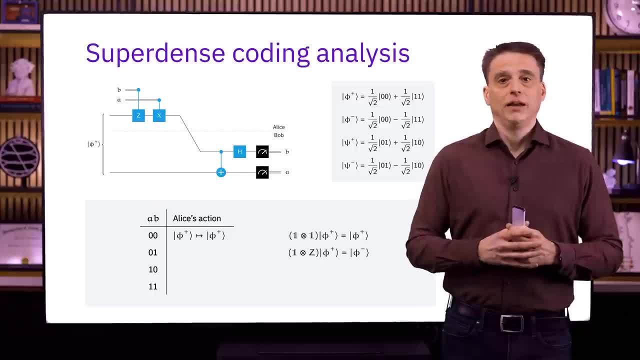 Well, because B is equal to one, we apply the Z gate and we don't apply the X gate because A is equal to zero, and we see that the overall effect is that Alice performs a Z gate. Alice is on the right because she's on the top, although it wouldn't actually make any. 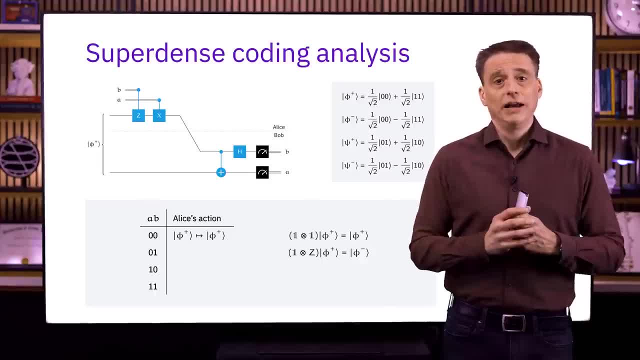 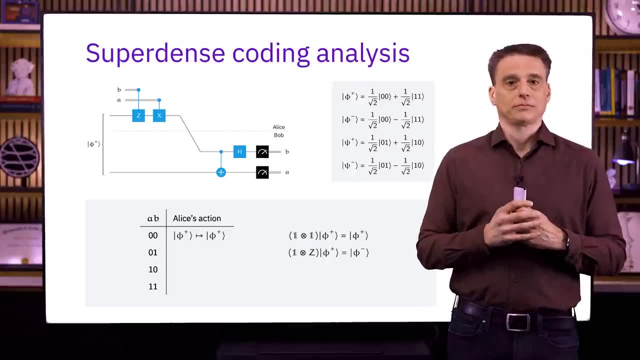 difference. in this particular case, The effect is that the phi-plus state gets mapped to phi-minus, which you can eyeball from these expressions if you remember how a Z gate works. So we can add this one to our table. There are two more cases to go through. 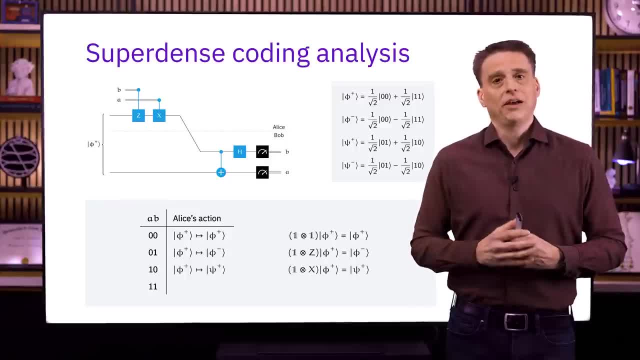 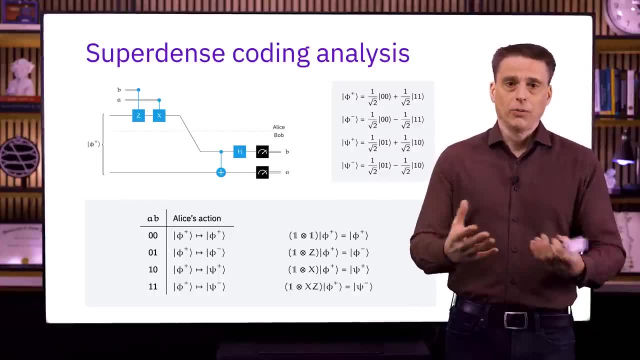 If A is equal to one and B is equal to zero, Then Alice performs an X gate which transforms phi-plus into psi-plus. And if A is equal to one and B is equal to one, then Alice performs Z, then X and we: 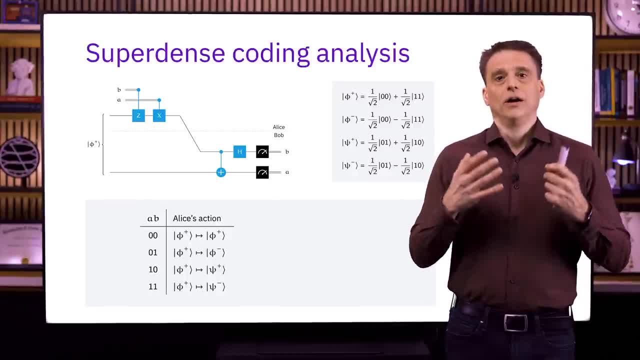 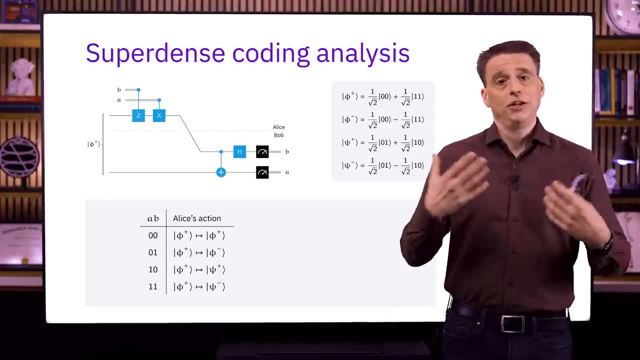 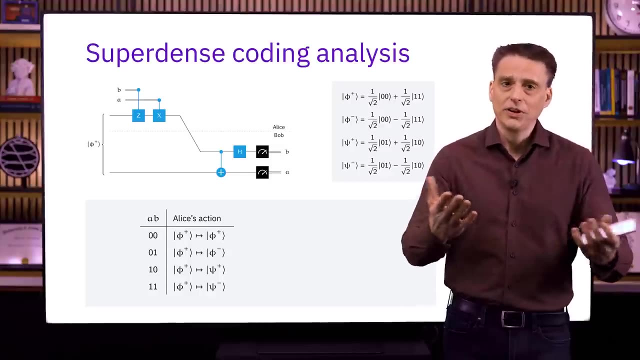 get psi-minus. So our table tells us what happens in the four possible cases, And that is that Alice effectively chooses which one of the four Bell states she would like to share with Bob, And she has the freedom to choose by acting on her qubit alone. and that's a pretty interesting. 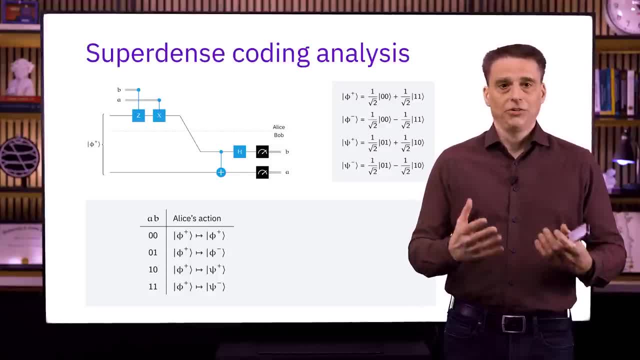 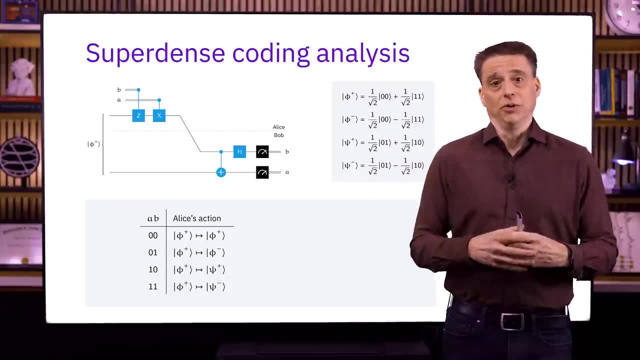 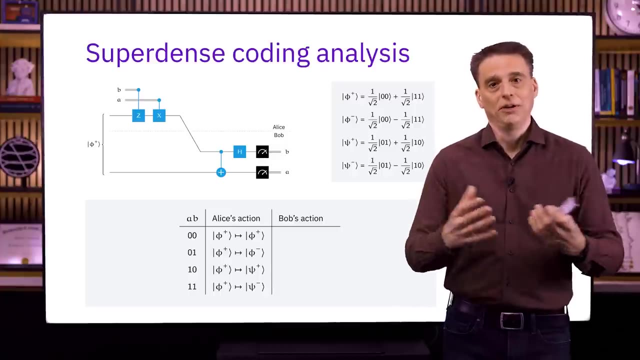 aspect of entanglement. Alice then sends her qubit to Bob. At this point Bob holds one of the four Bell states and he just needs to figure out which one it is to recover the bits. And we can check that. indeed, a controlled, NOT gate, followed by a Hadamard gate, as we 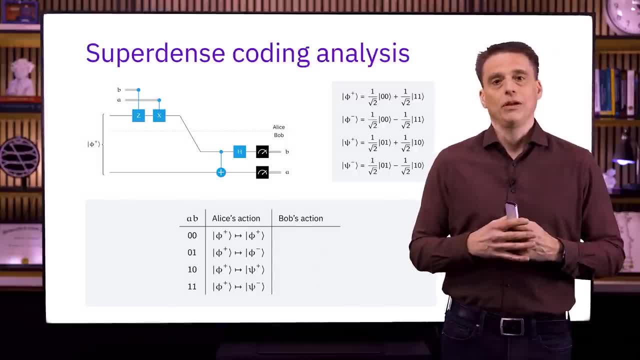 have in the diagram does the right thing. I won't go through them in detail, but if you choose to do that, you'll find that the effect is as you see here in the table. One way to check that is simply to compute. 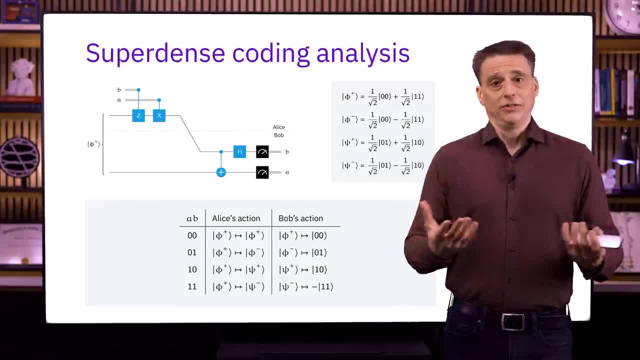 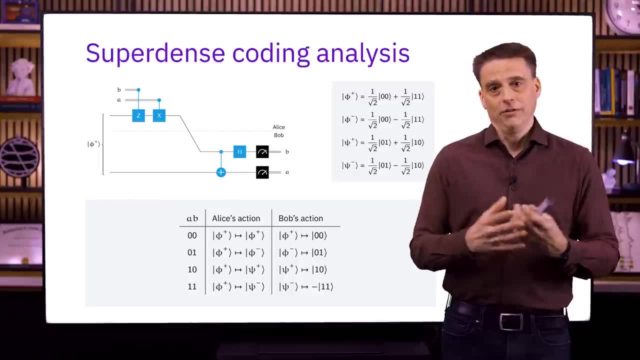 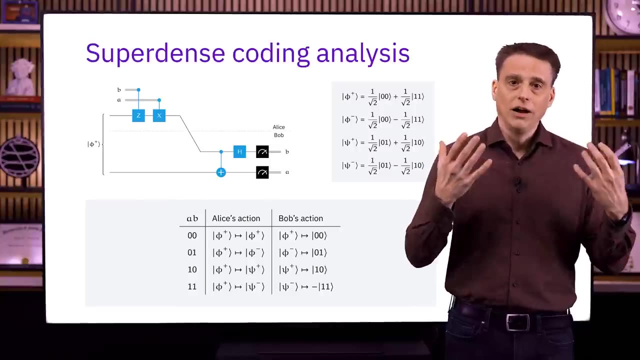 Alternatively, we can recognize that we actually already went through this in reverse in the previous lesson. In the previous lesson we had the Hadamard gate first and the controlled- NOT- gate second and we saw that that circuit mapped standard basis states to Bell states with a pesky. 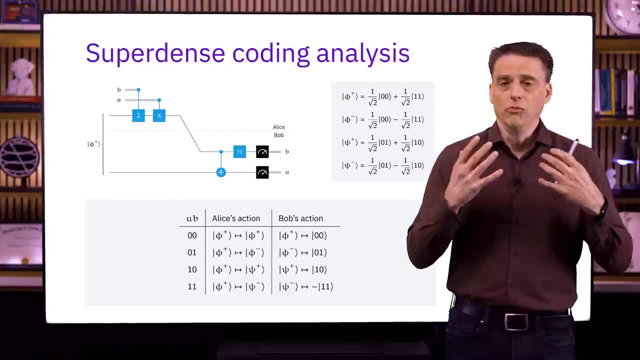 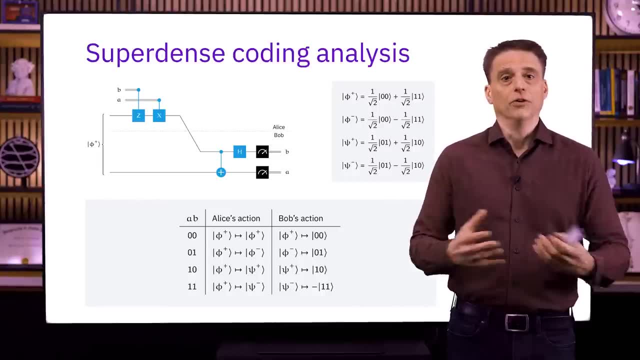 minus sign. in one of the cases, When we reverse the order of the gates and we consider the fact that both of these two gates are their own inverses, what we get is the inverse, And so what we have in this case is that the action goes in the opposite direction and 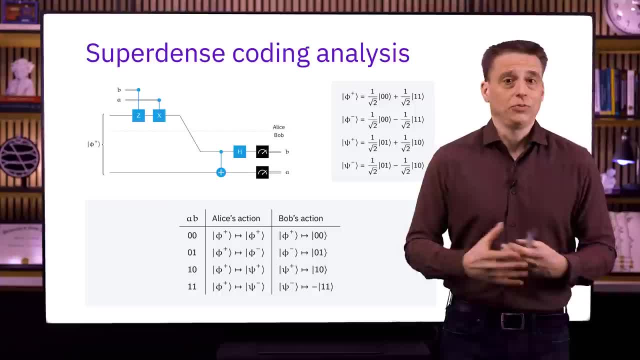 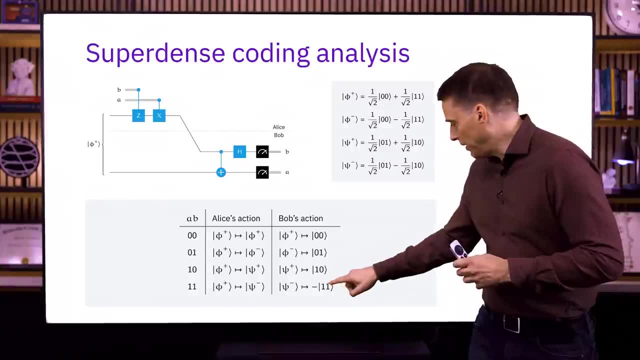 the minus sign can choose whichever side it wants to be on, but otherwise it's where it belongs And at this point it's immediate that the measurement reveals the correct values. The minus sign here doesn't bother us because 1, 1 appears with probability 1 in this case. 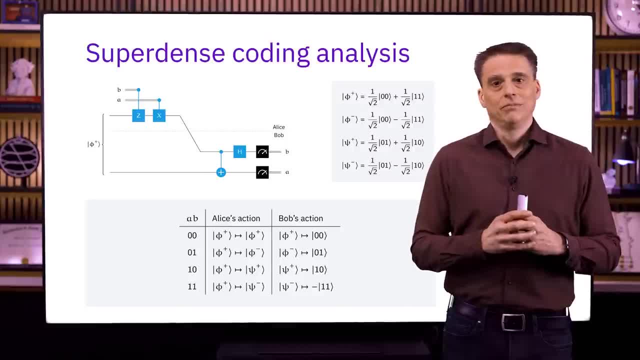 and that's all there is to the analysis. In a nutshell, Alice picks a Bell state and Bob figures out which one. it is Just a couple of brief notes. If you have any questions, please feel free to reach out to me. 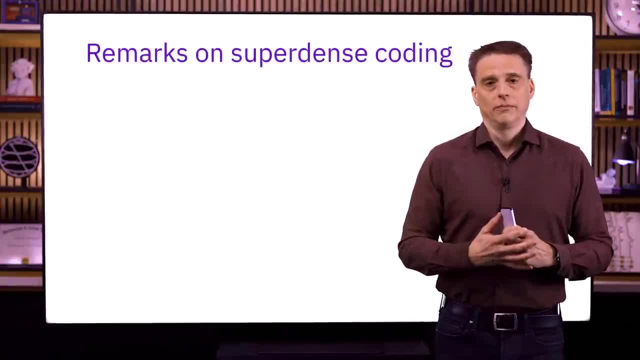 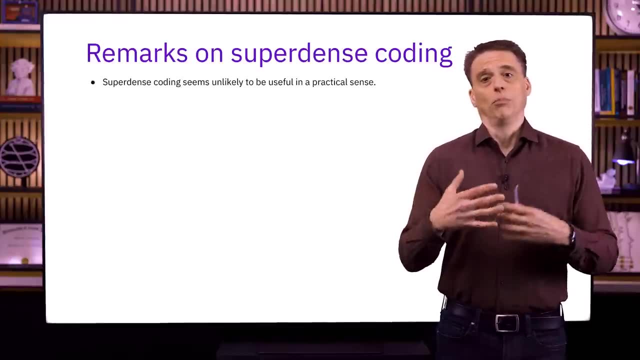 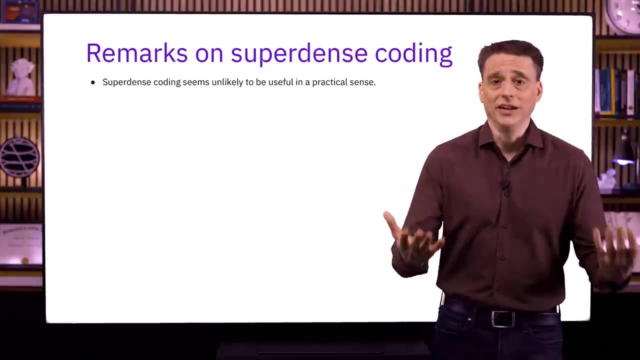 Thank you. Let's take a few more brief remarks about superdense coding before we move on. First, we should acknowledge that superdense coding is probably not likely to be useful or practical in any sense as a means to transmit classical information. Classical communication is very inexpensive and physically sending qubits is challenging. 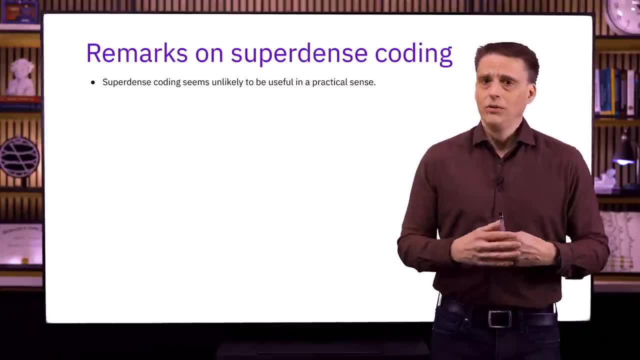 to say the least. And so long as that's the case, we wouldn't expect any practical advantage at all to come from superdense coding. But just because superdense coding is superdense doesn't mean that superdense coding is superdense. 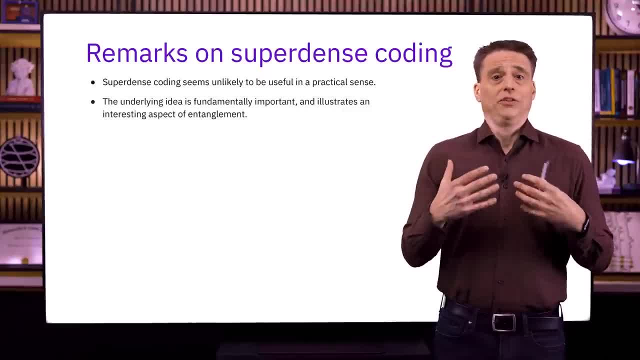 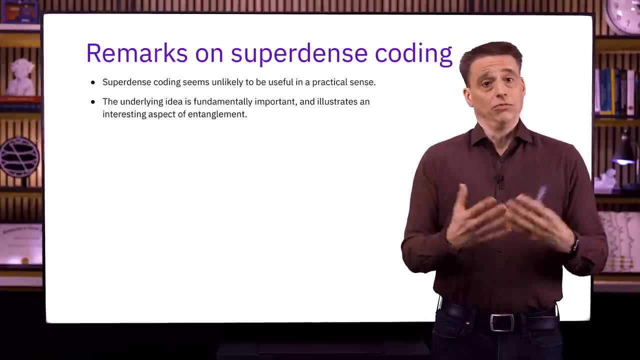 But just because it isn't likely to be practical doesn't mean that superdense coding is not interesting. It's very interesting, in fact. For one, the underlying idea is really quite fundamental, And when I refer to the underlying idea, I mean the idea that if Alice shares a Bell, 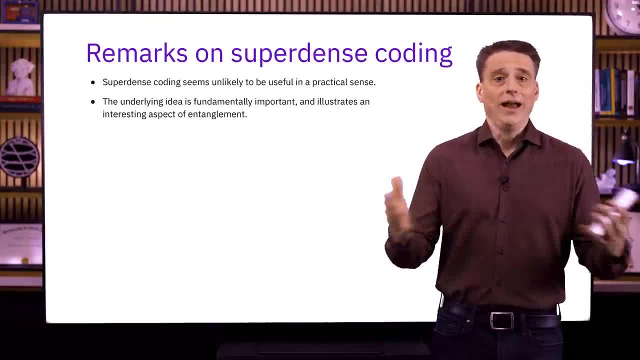 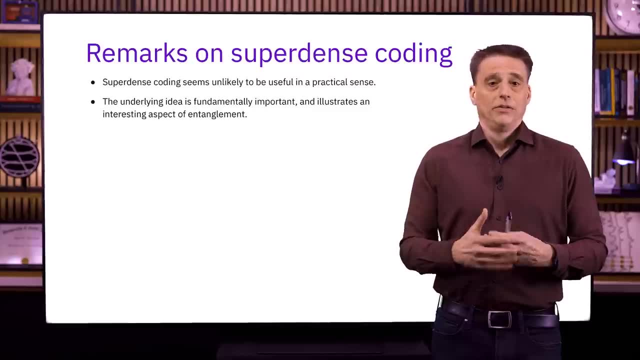 state with Bob. then she can choose to change that state to any other Bell state that she chooses, all by herself. She doesn't need Bob's help at all to do that. This is a specific example that concerns the Bell state. I'm not going to go into too much detail here. 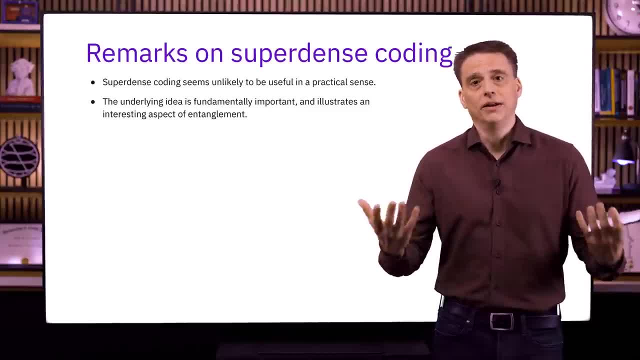 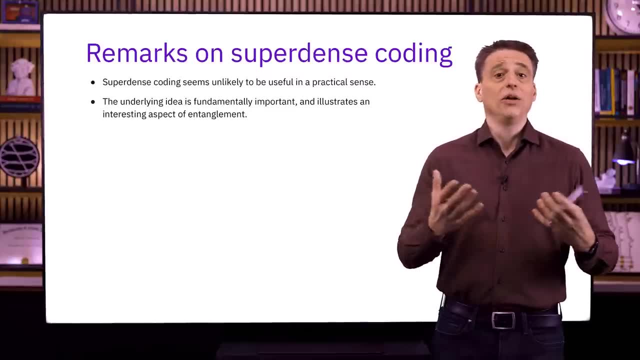 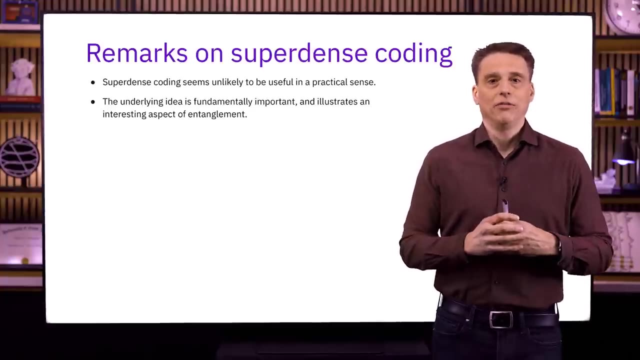 But there's a more general underlying idea that concerns the freedom that one player has to transform an entangled state that's shared with another player, And understanding exactly what that freedom is is an important step in understanding quantum information, And we'll see exactly how to describe that freedom in simple and elegant terms in the 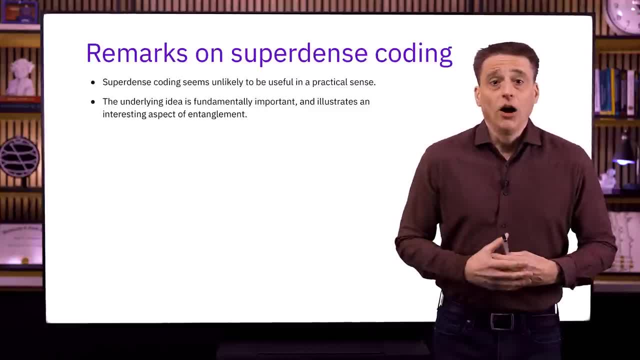 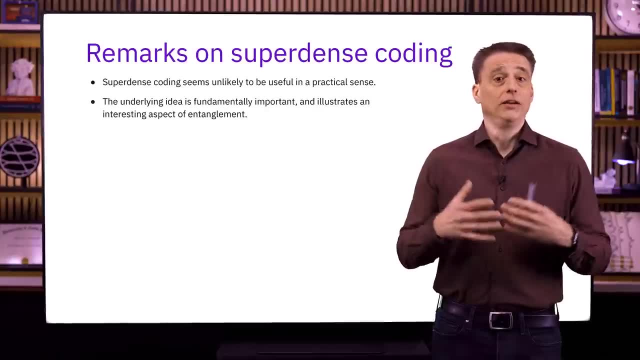 third unit of the series, Superdense coding, also provides a concrete example of what you can do with entanglement, which is to allow two classical bits to be transmitted, And that's what we're going to do. As I already mentioned, this is provably not possible by Holowohl's theorem without 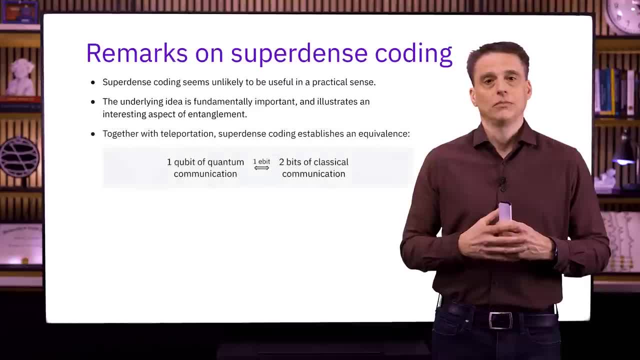 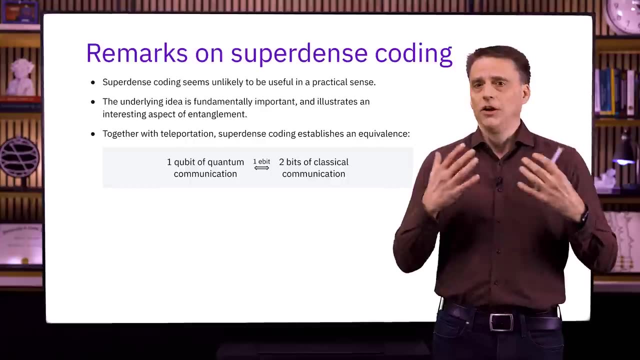 entanglement. We can also consider teleportation and superdense coding together And we see that they establish an equivalence between one qubit of quantum communication and two bits of classical communication. As long as you're willing to spend one ebit, you can effectively convert one to the other. 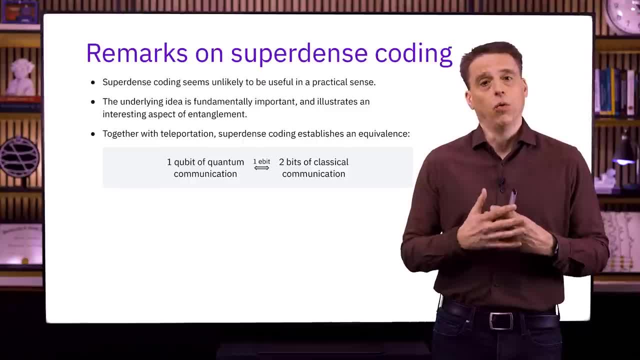 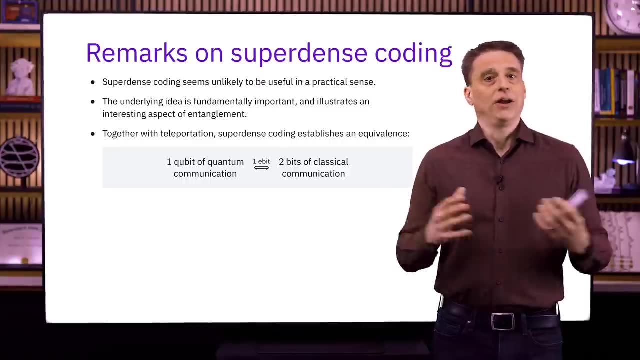 Teleportation allows for the communication of one qubit using two classical bits of communication, And superdense coding goes the other way and allows two classical bits of communication using one qubit of quantum communication Without spending the ebit. however, you cannot transform either one into the other. 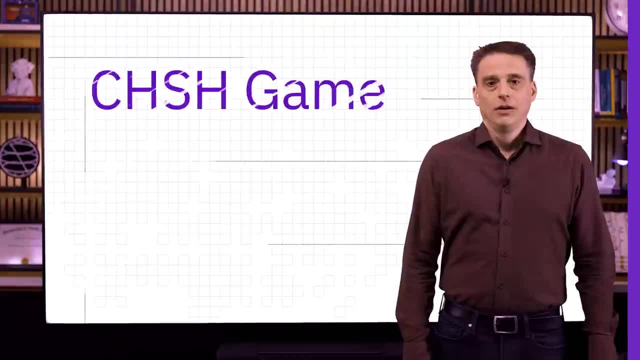 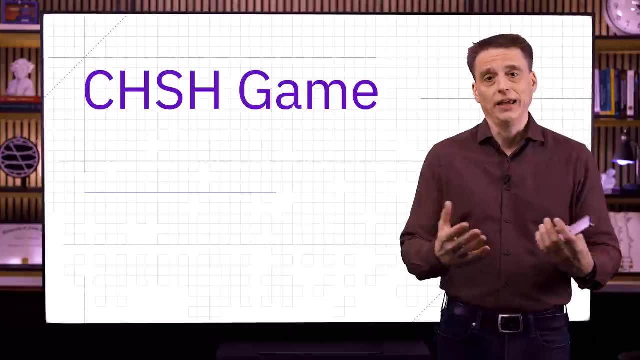 It's entanglement that makes this possible. The third and final example that we'll cover in this lesson is not a protocol, but a game known as the CHSA protocol. When we talk about a game in this context, we're not talking about something that's meant. 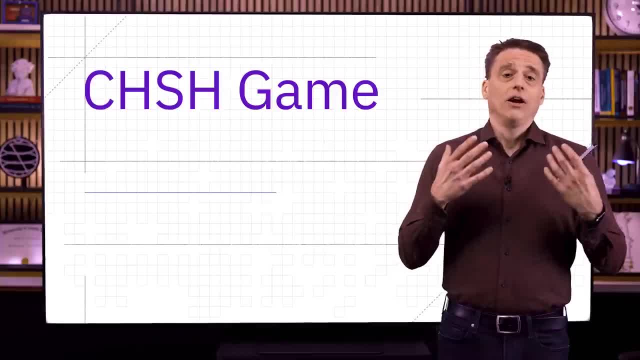 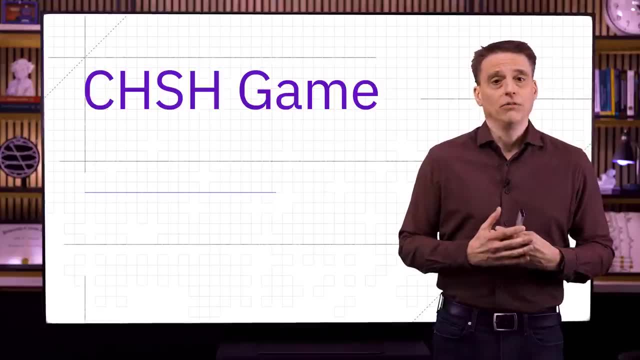 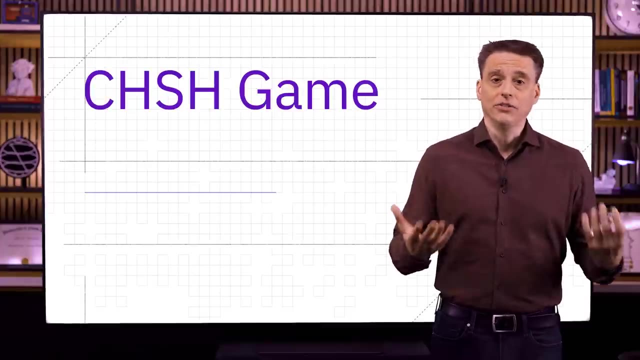 to be played for fun or sport, but rather a mathematical abstraction in the sense of game theory, for instance. Mathematical abstractions of games are very commonly studied in economics and computer science, for instance, And there's quite a lot of value to be found in this abstraction. 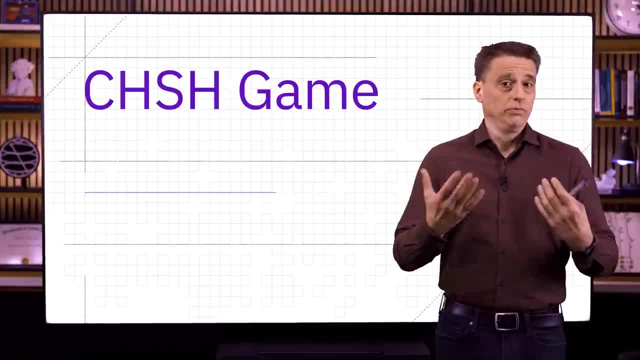 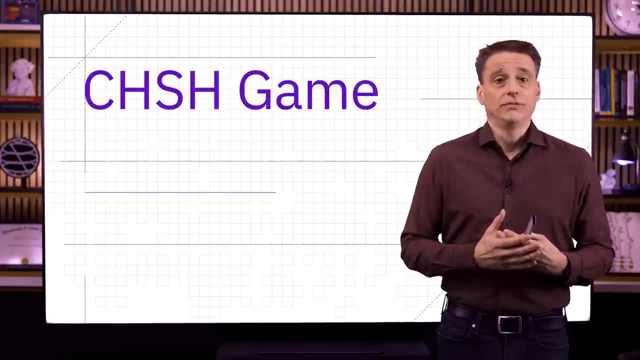 So games are not all fun, and games, as it turns out, Although it is fun to play, It's fun to think about them. In this particular case, what we have is essentially a thought experiment that can be described in a pretty intuitive way as a game. 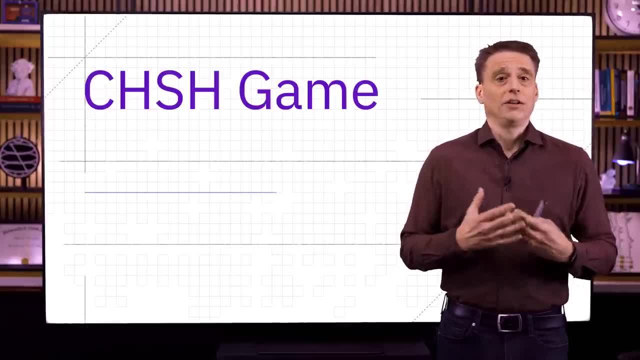 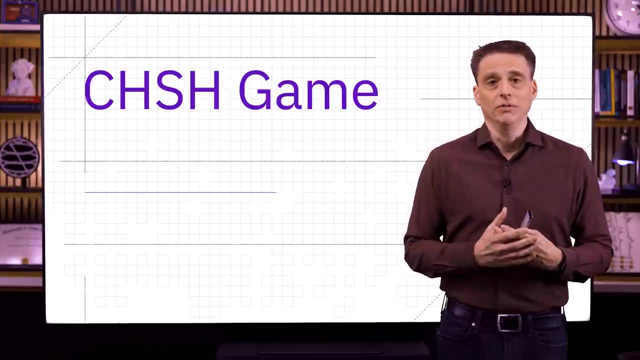 The letters CHSH refer to the authors, John Clouser, Michael Horn, Abner Shimony and Richard Holt, of a 1969 paper where the example was first described. They didn't describe it as a game, in fact, and it's pretty common to refer to this example. 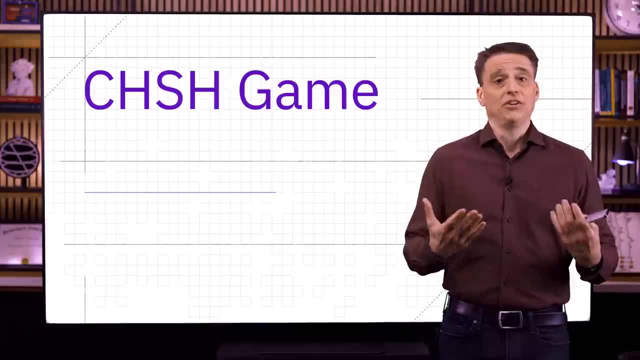 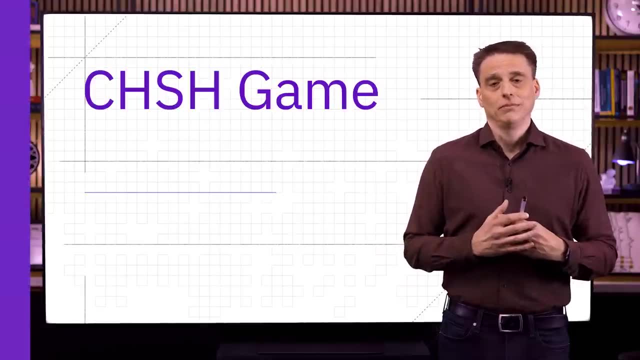 not as the CHSH game, But as a game Rather as the CHSH inequality. For a computer scientist like me, however, it's just very natural to describe it as a game. I've already suggested that mathematical abstractions of games are both important and 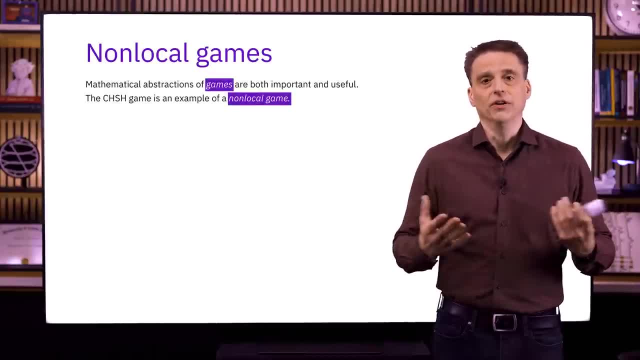 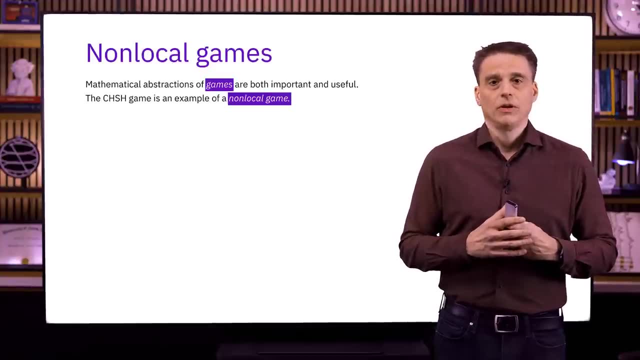 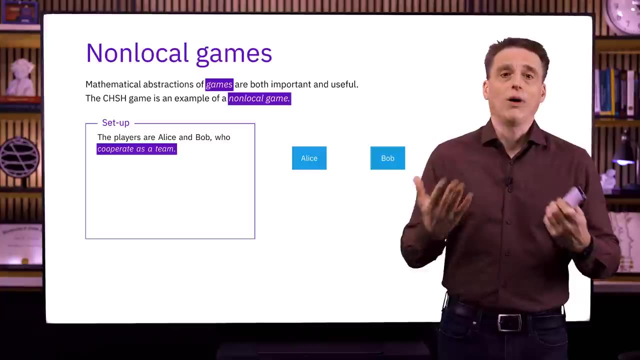 useful and there are many different categories of games that can be considered. The CHSH game is an example of a class of games called non-local games. Here's the setup in general for a non-local game. We have two players, Alice and Bob, who cooperate as a team. 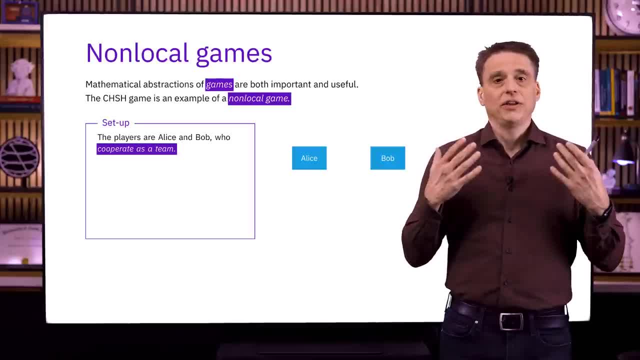 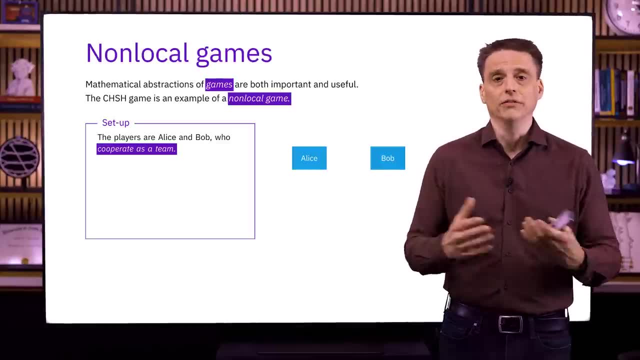 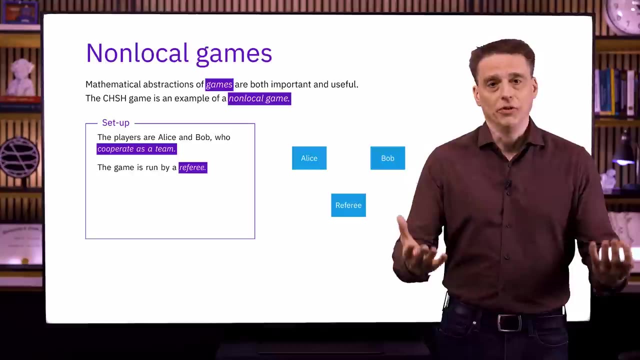 So they either win together or they lose together. This means that they have no incentive to act selfishly. so it's essentially the opposite extreme to zero-sum games, which are purely competitive. Here the game is purely cooperative. There's a third entity called the referee. 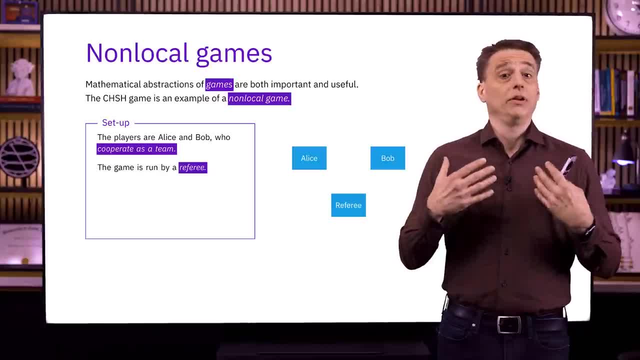 The referee isn't a player in the game, but rather the referee runs the game And in fact, you can think about the specification of a professional player. The referee is the only player in the game. The referee is the only player in the game, but the referee runs the game. 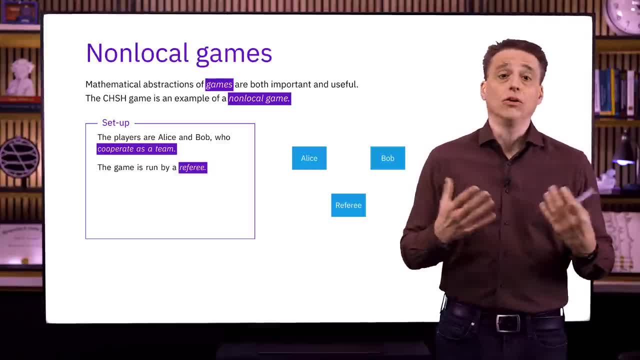 The referee is the only player in the game, but the referee runs the game. But the referee is the only player in the game, but the overstepper in the game, The referee, runs the game. And what about the specification of a particular instance of a non-local game and the specification? 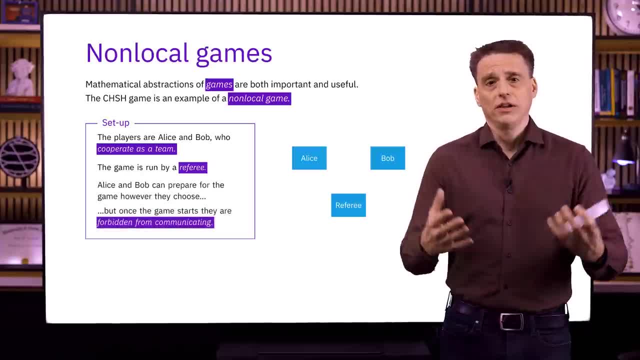 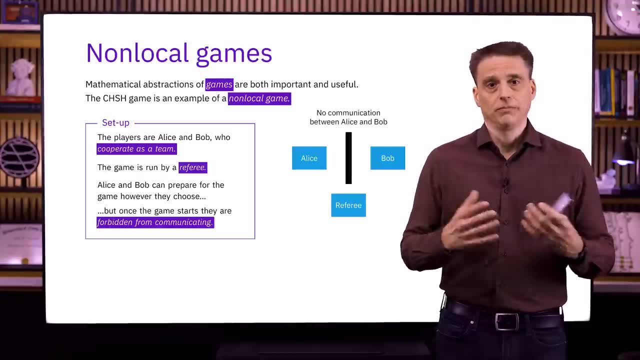 of a referee as being equivalent. There's a critically important constraint that's placed on Alice and Bob, which is that once the game starts, they're forbidden from communicating with one another. They can agree beforehand on whatever strategy they choose, but no communication is allowed. 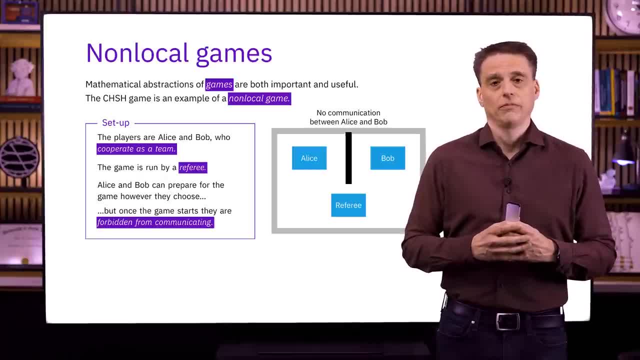 between them during the game itself. If you like, you can imagine the game taking place in a very religious setting. That's a typical case in this experience, And I'm going to go back to this example here, because there are a few things that actually 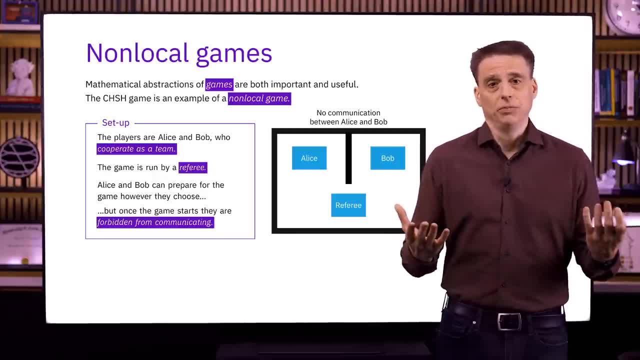 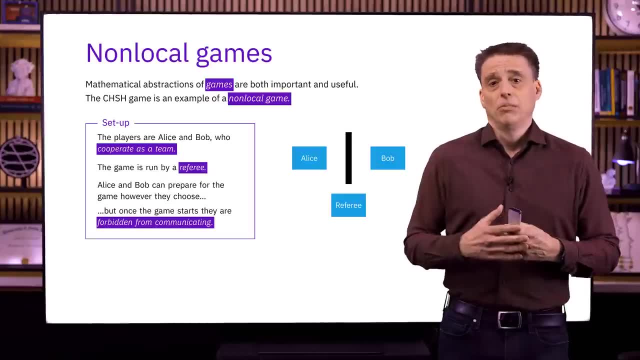 matter in the game in a secure facility of some sort, as if the referee is playing the role of a detective and Alice and Bob are suspects located in different rooms in a police station. But another way of thinking about the setup is that Alice and Bob are separated by a vast distance. 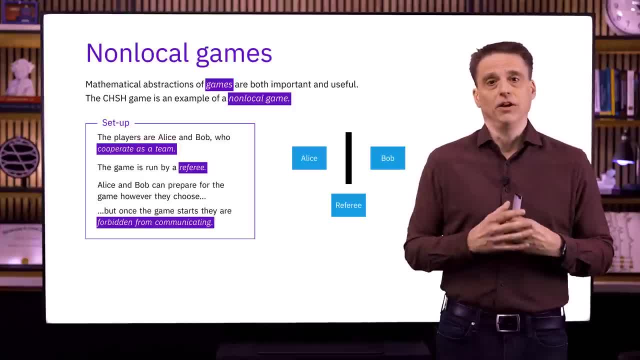 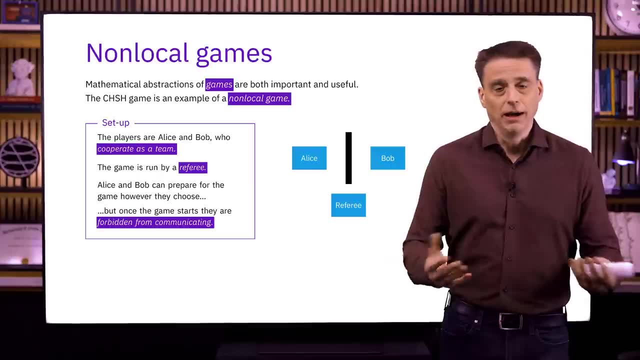 and communication is prohibited because the speed of light doesn't allow for communication to happen quickly enough. If Alice tries to send a message to Bob, for instance, the game will be over by the time Bob receives it. The way a non-local game works is that 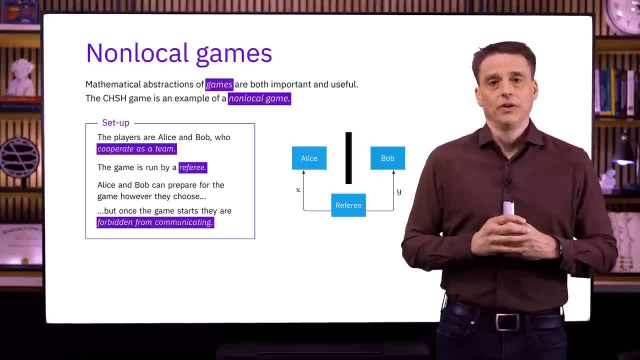 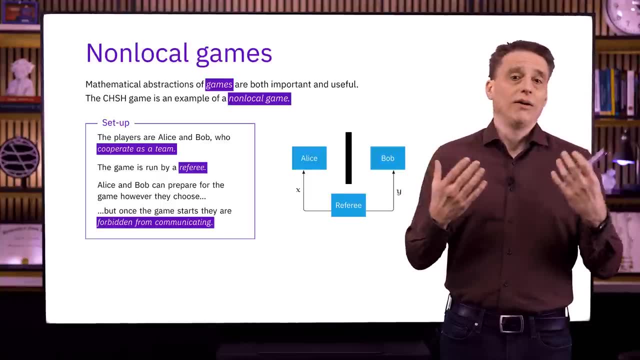 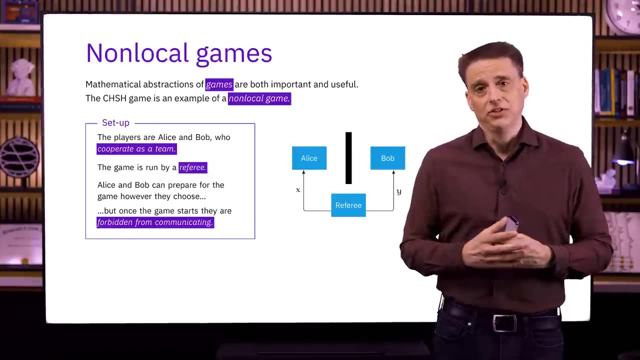 first, the referee asks both Alice and Bob a question. Alice's question is labeled X and Bob's question is labeled Y. In general, you can think about X and Y as being classical states from whatever classical states that you like, And in the specific case of the CHSH game. 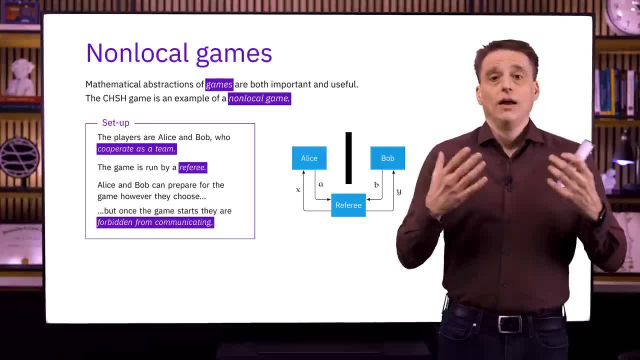 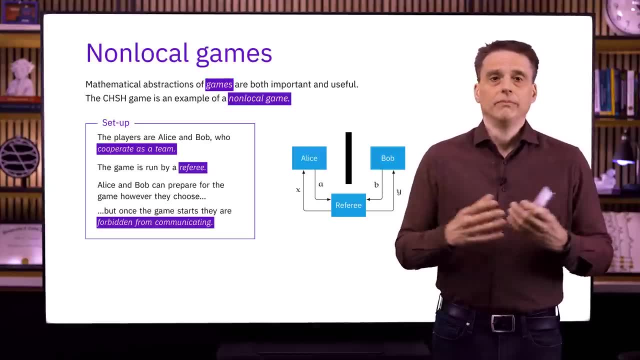 X and Y are bits. Alice and Bob must then provide answers. Alice's answer is labeled A and Bob's answer is labeled B, And again, these answers can be viewed as classical states in general And, like the questions, they will be bits in the CHSH game. 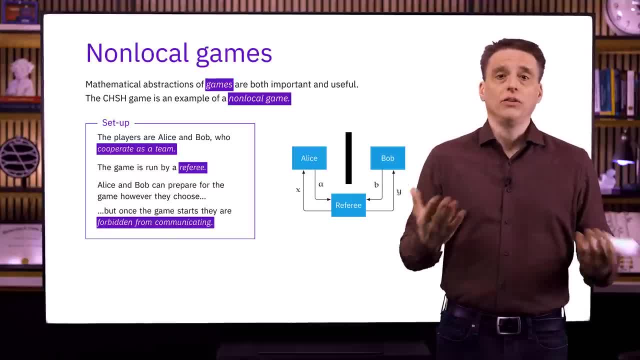 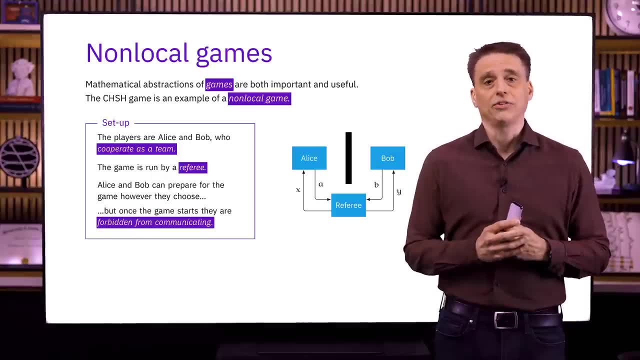 At this point the referee makes a decision. Alice and Bob either win or they lose, depending on whether or not the pair of answers A- B is deemed correct for the pair of questions X- Y that the referee asked- And I'll say a little bit more about this in just a moment- 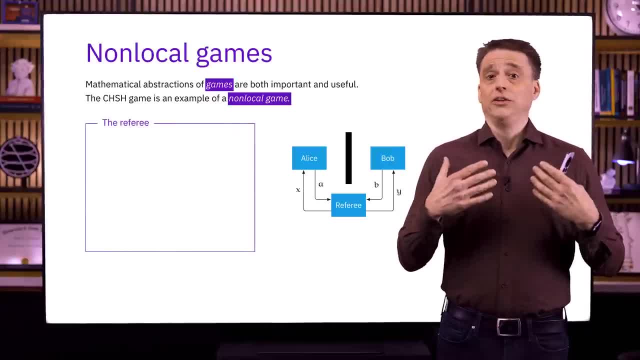 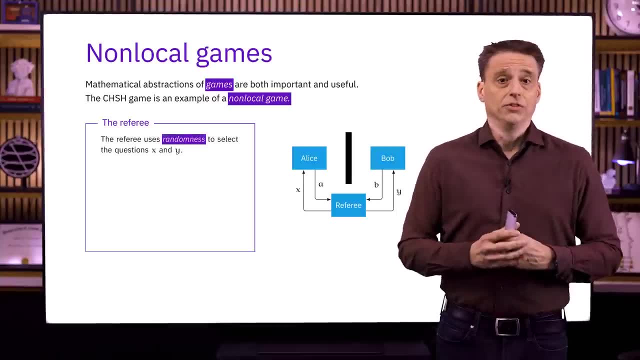 First let's take a closer look at the referee to understand what it is that's potentially changed And what makes it challenging for Alice and Bob in a non-local game. And what makes a non-local game potentially challenging is that the referee can use randomness. 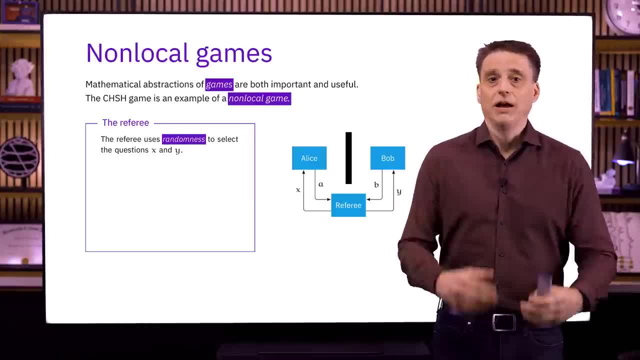 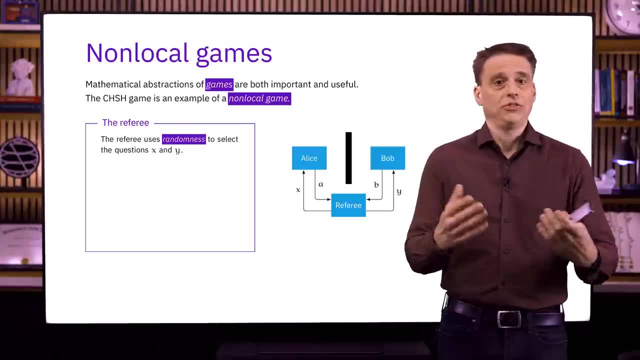 to choose the questions X and Y. That means that Alice and Bob have uncertainty. They don't know ahead of time what question they're going to be asked And perhaps, more importantly, they don't know what question the other one received. And it's that uncertainty. 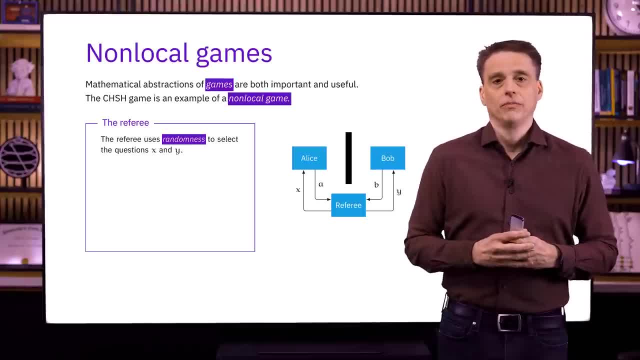 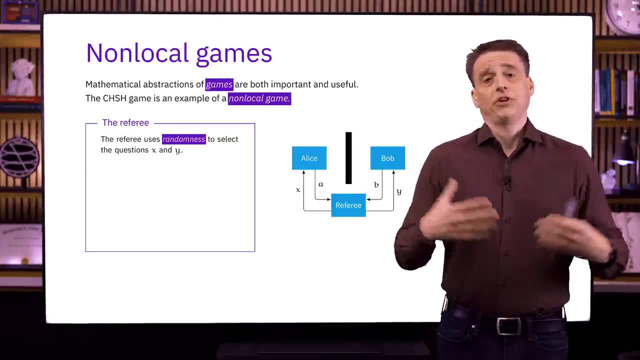 together with the fact that they can't communicate, that presents a challenge. So it's similar to the situation where a detective interrogates two suspects in different rooms If the suspects don't know what questions the other one has asked. it's much harder if they're guilty. 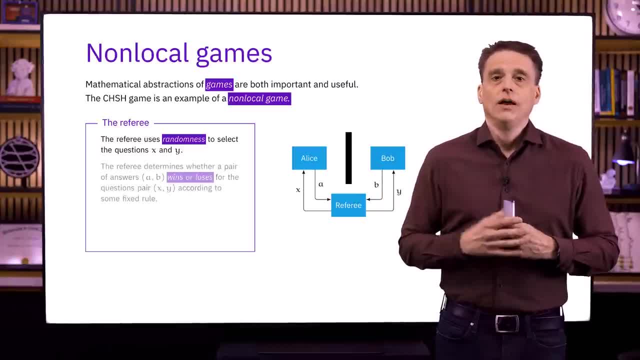 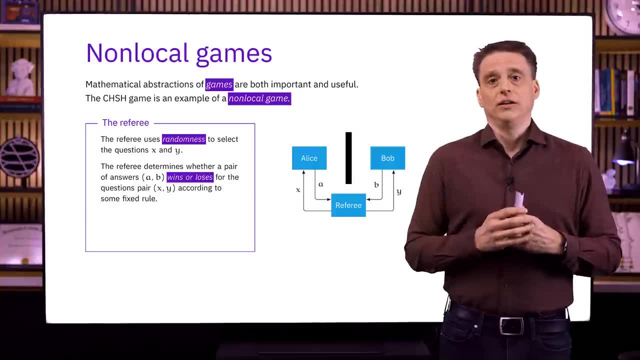 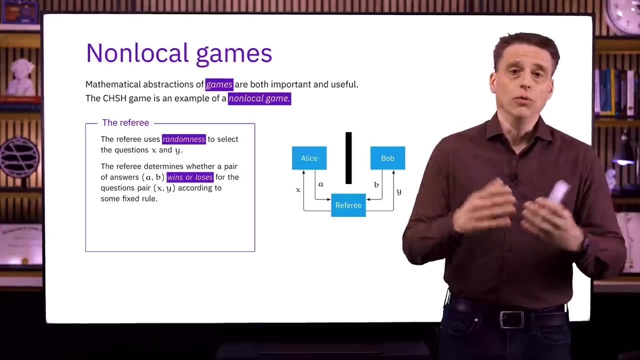 to keep their story straight Now. I mentioned a short time ago that the referee makes a determination that Alice and Bob have either answered correctly or incorrectly, depending upon the questions that they were asked. It's assumed that this determination is made according to some fixed rule. 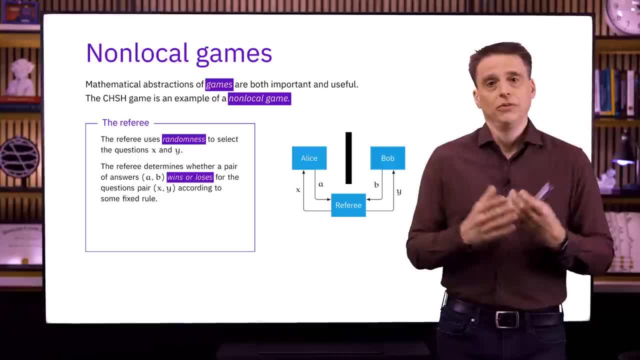 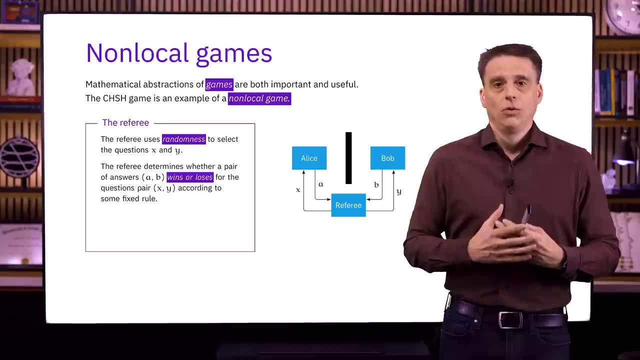 And you can consider any rule that you want. but whatever it is, it is assumed that Alice and Bob know the rule, So at least they have a fighting chance to answer correctly. We'll take a look at the rule for the CHSH game in a moment. 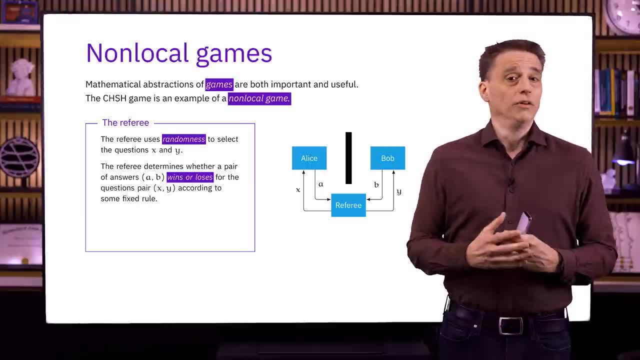 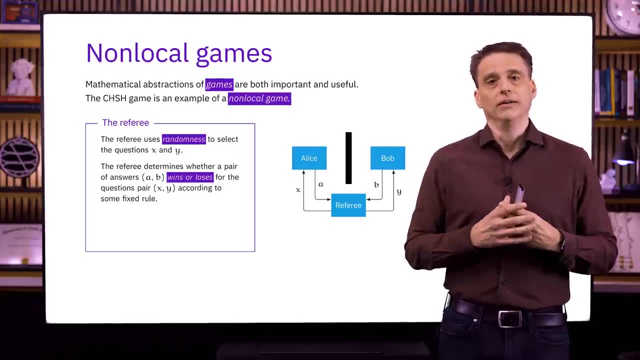 but we could consider a different rule and we would have a different example of a non-local game. Some non-local games are interesting and in fact some are quite fascinating and mysterious to this day, And some aren't so interesting. That's just the nature of the non-local game model. 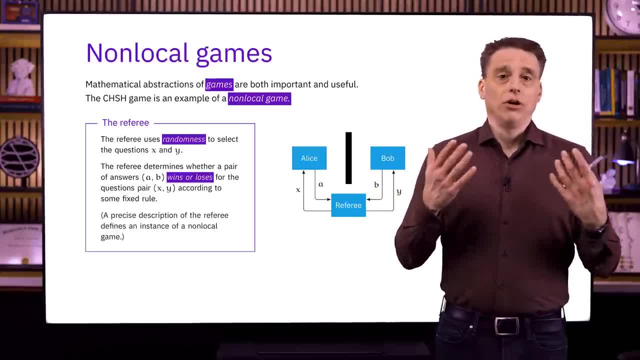 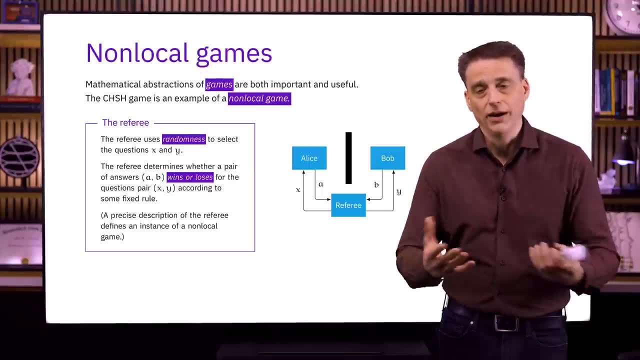 Anyway, these are the two different things that are needed to describe a referee: How exactly are the questions chosen and which answer pairs are correct for each possible question pair? If we have a description of those two things, then we have a description for the referee. 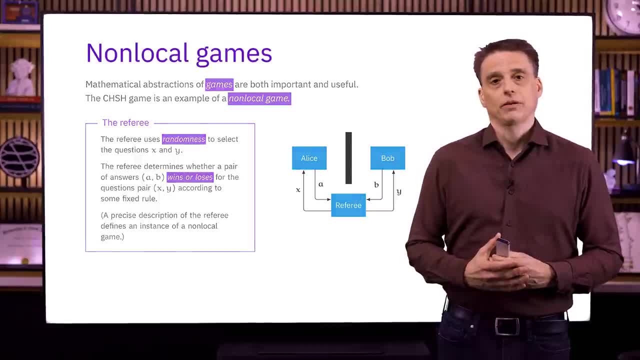 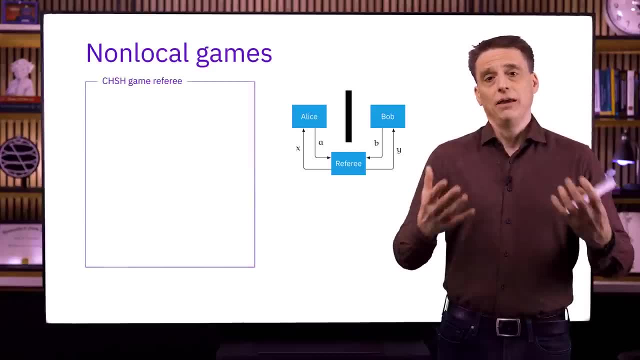 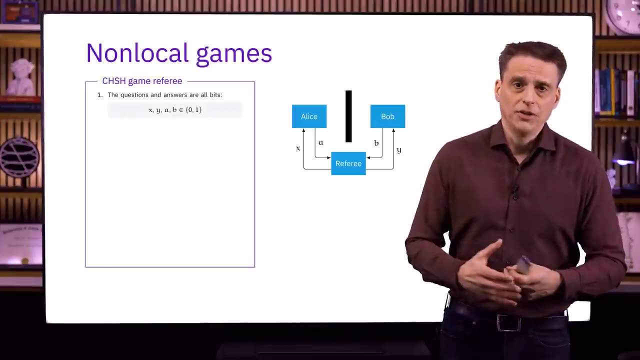 And that effectively describes an instance of a non-local game. Now let's take a look at the CHSH game specifically. The way that the game is defined or, equivalently, how the referee is defined, is as follows. First, as I've already mentioned, 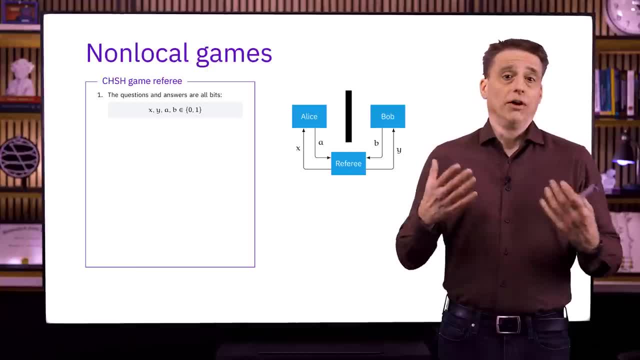 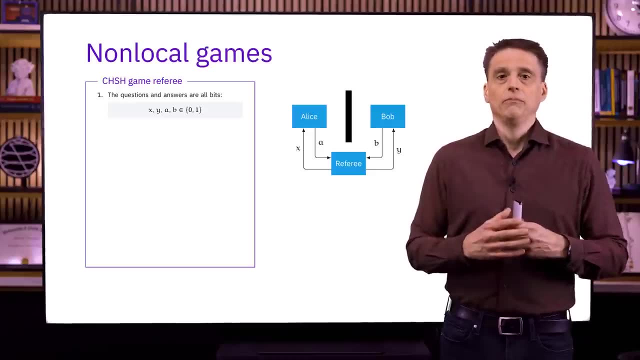 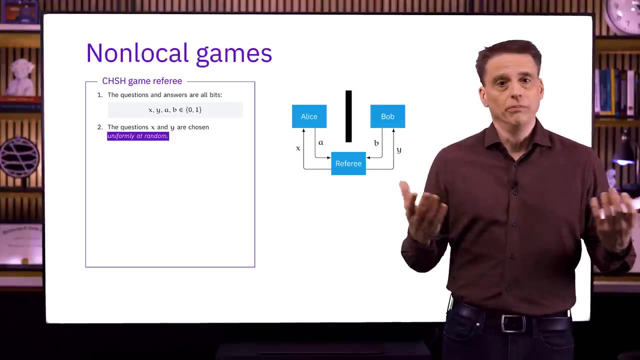 the questions and answers are all bits, So the referee sends a bit X to Alice and a bit Y to Bob and they each respond with a bit. Alice responds with A and Bob responds with B. The way the referee chooses which questions to ask is simple. 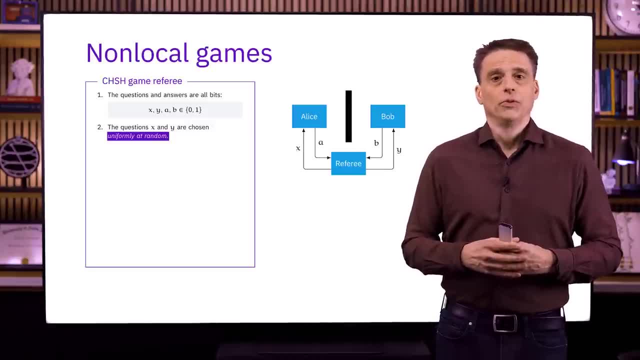 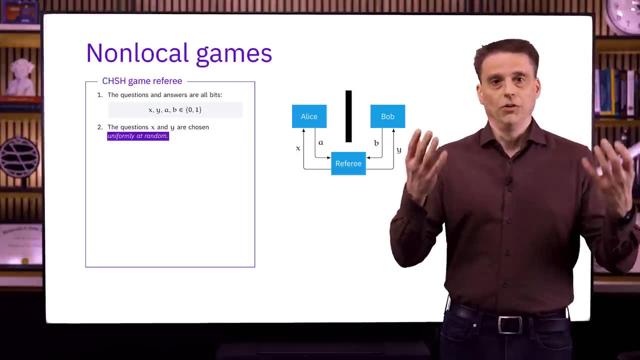 He chooses them uniformly at random. So the pair of questions X- Y is equally likely to be any one of the four possibilities: Zero, zero, Zero, one, One zero And one one. Finally, the rule that determines which answers win: 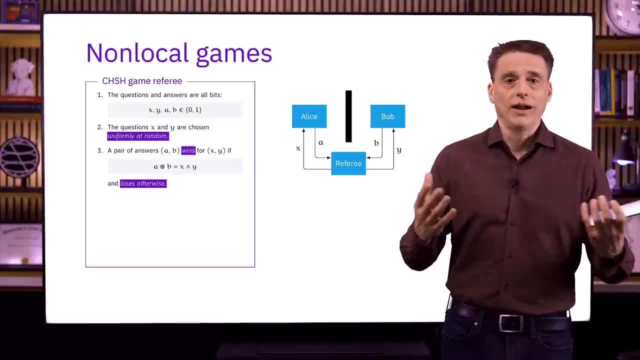 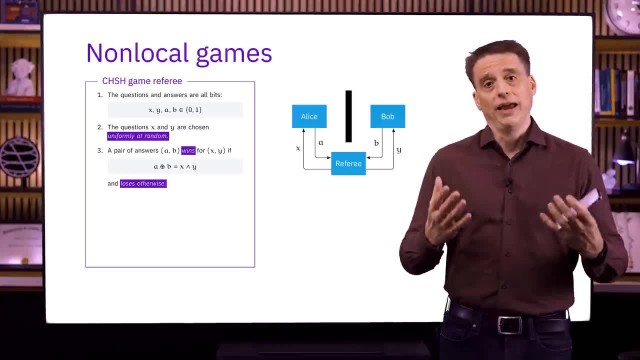 and which answers lose, is that a pair of answers- A- B- is correct for the pair of questions X- Y if, and only if, the exclusive OR of A and B is equal to the logical AND of X and Y. That may be a little bit easier to digest. 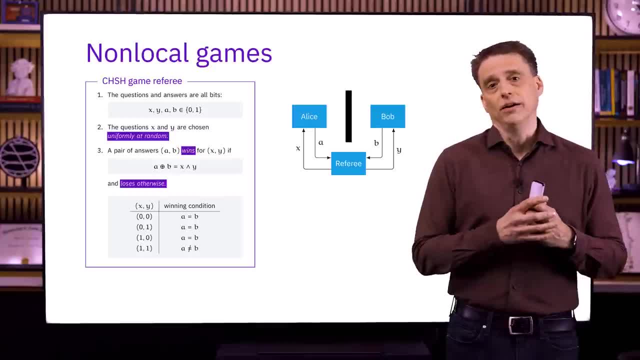 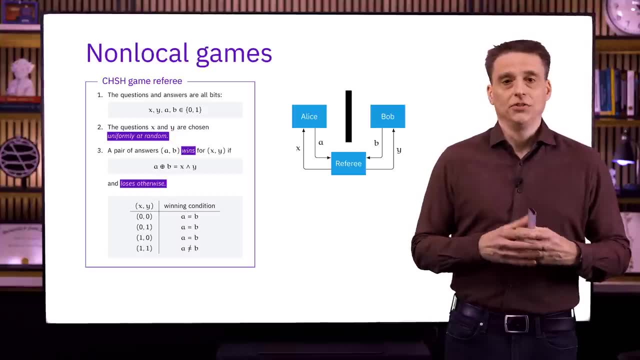 if we express those conditions in the form of a table. as you see right here, In the first column we have the four possible question pairs And in the second column we have the conditions on A and B that are required for Alice and Bob to win. 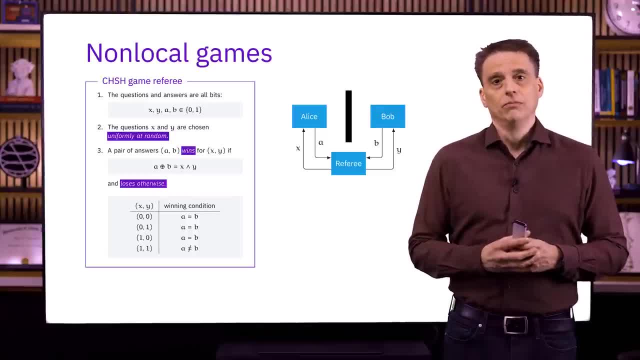 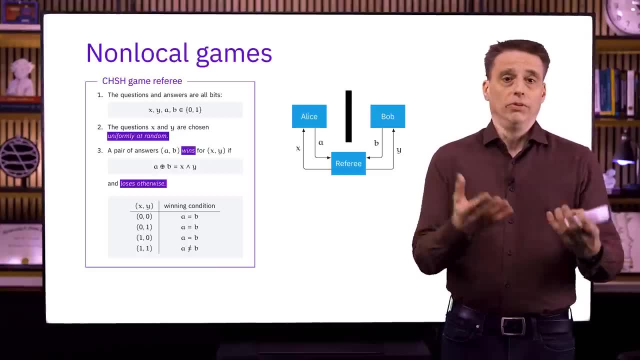 In the first three cases, the AND of X and Y is zero, So the exclusive OR must be equal to zero in order for them to win. And that's the same thing as saying that A and B must be equal, because A and B are bits. 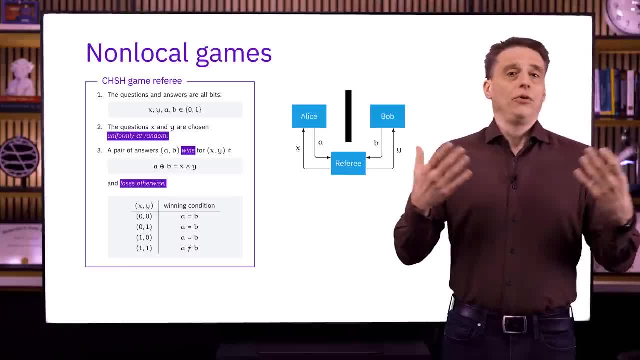 In the fourth case, the AND of X and Y is equal to one, And so the exclusive OR of A and B must be equal to one in order for Alice and Bob to win, And that's the same thing as saying that A and B. 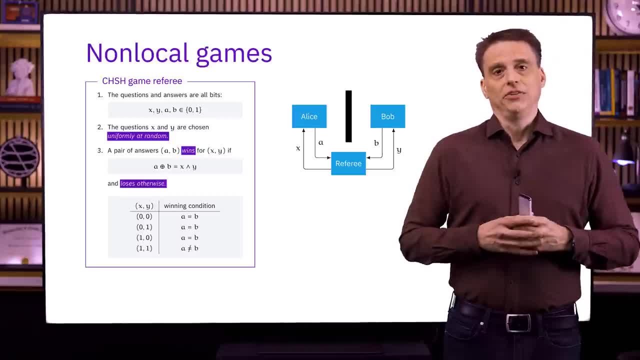 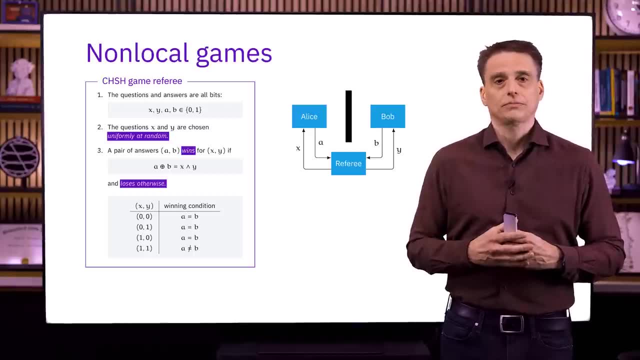 must be different. So that's the CHSH game, And now we can think about different possible strategies for Alice and Bob and how well they can do in this game. Let's start by thinking about deterministic strategies where Alice's answer A is a function. 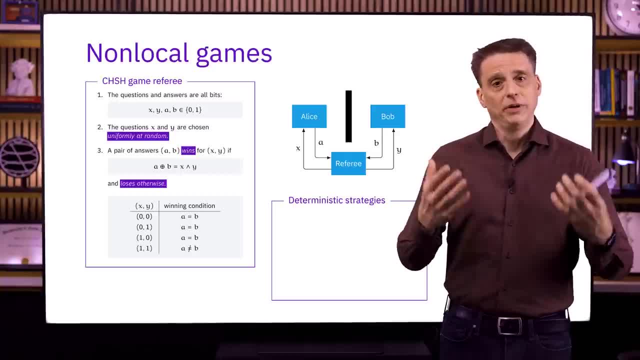 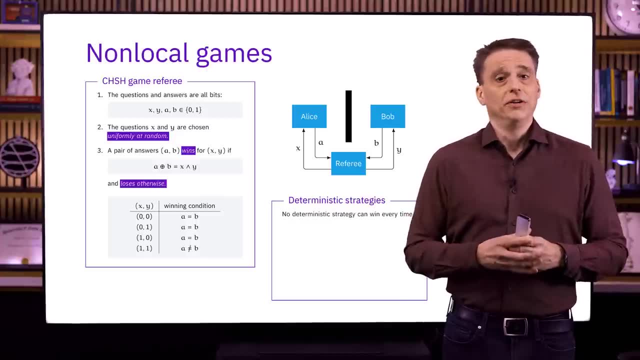 of the question X that she receives, And likewise Bob's answer B is a function of the question Y that he receives. And as it turns out, no deterministic strategy can possibly win every time. One way to reason that is simply to go one by one. 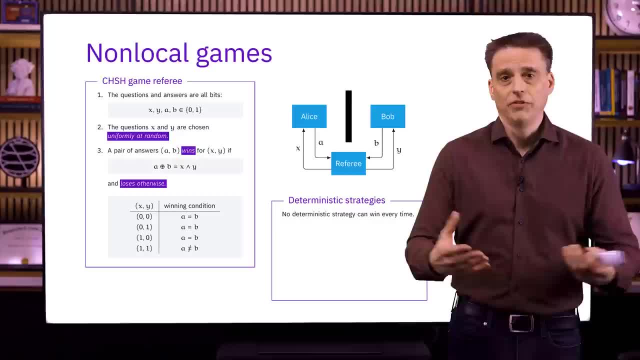 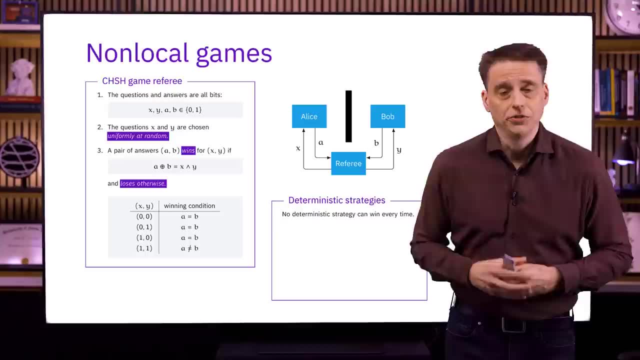 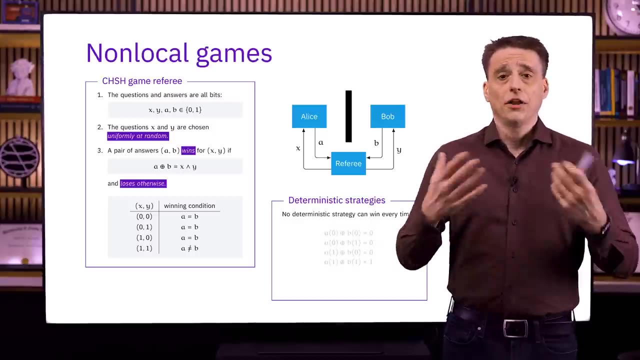 through all of the possible deterministic strategies and to check that every one of them loses. for at least one of the four possible question pairs, Alice and Bob each have four possible functions to choose from. We saw those four functions in lesson one, So there are 16 possibilities to check overall. 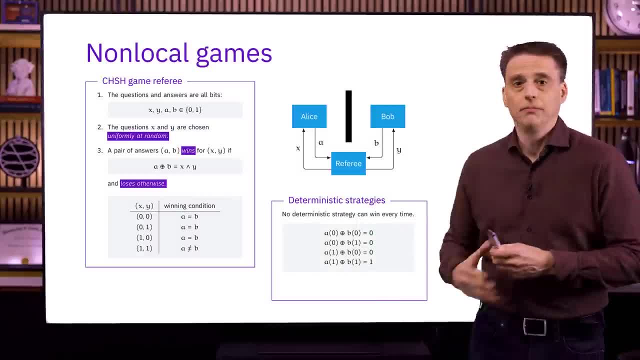 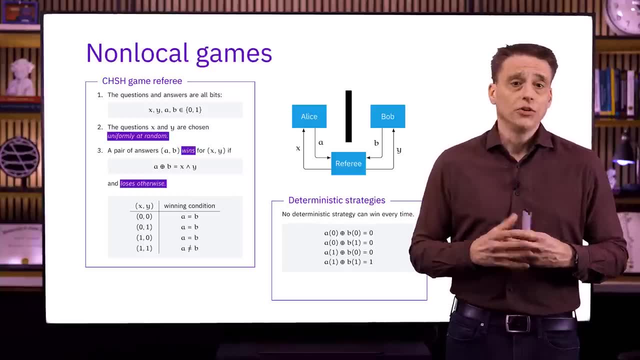 Another way to see that is to think about the equations here on the screen. We're thinking about deterministic strategies where A and B are functions of X and Y respectively. So we're going to look at the equations here on the screen. So, for example, A of zero represents Alice's answer. 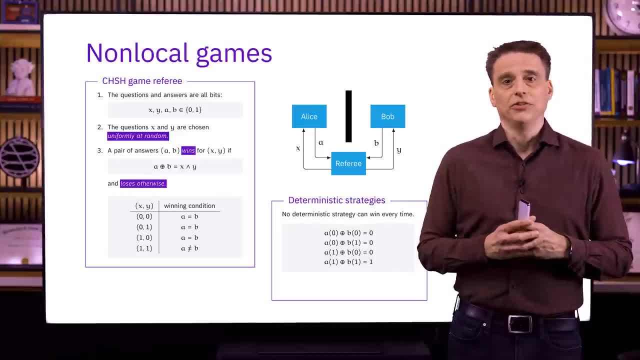 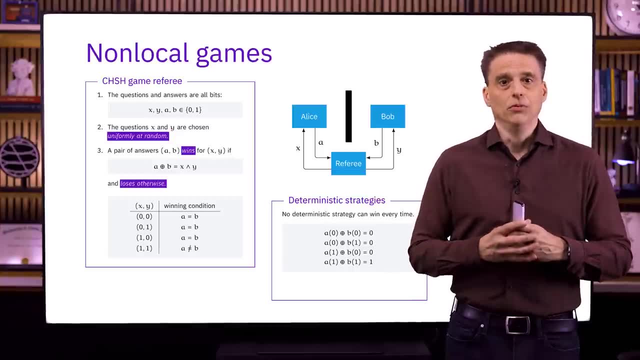 when her question X is equal to zero and A of one represents Alice's answer when her question X is equal to one. These are the four equations that have to be true in order for the winning conditions to be met in each of the four cases. 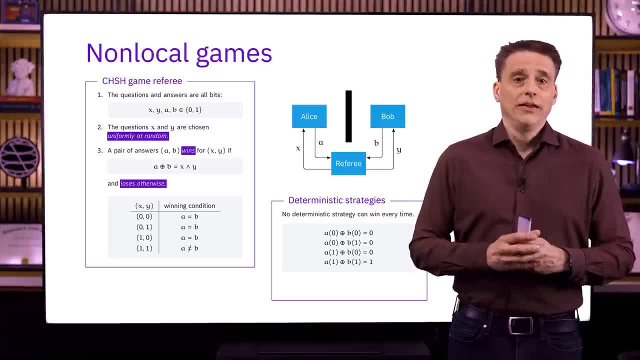 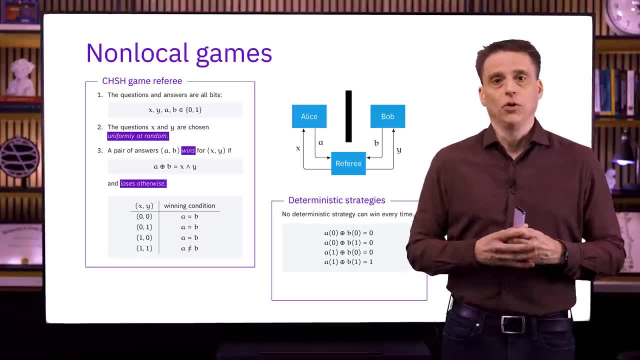 For example, if X is equal to zero and Y is equal to zero, then the exclusive or of A and B must be equal to zero, Whereas in the case that X is equal to one and Y is equal to one, the exclusive or of A and B must be equal to one. 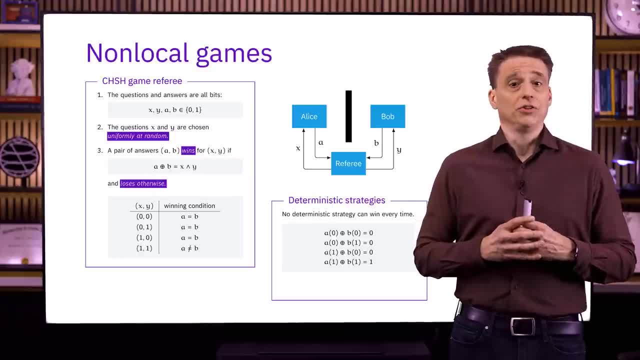 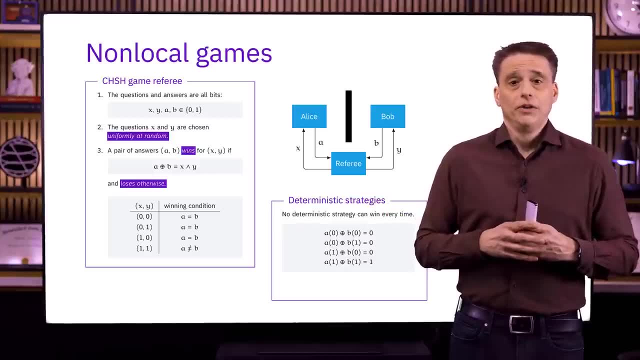 One way we can see that there's no way to choose the functions A and B so that these equations are all true is simply to take the exclusive or of all of the equations. The exclusive or of any binary value with itself is equal to zero. 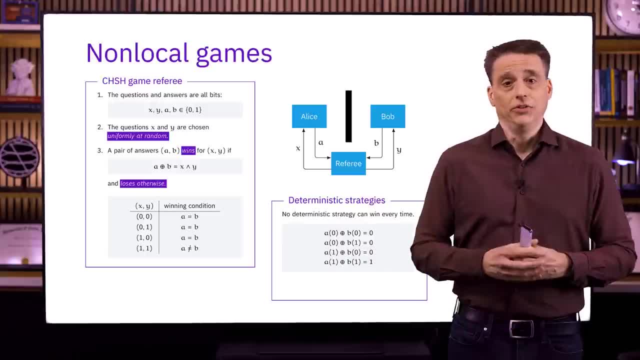 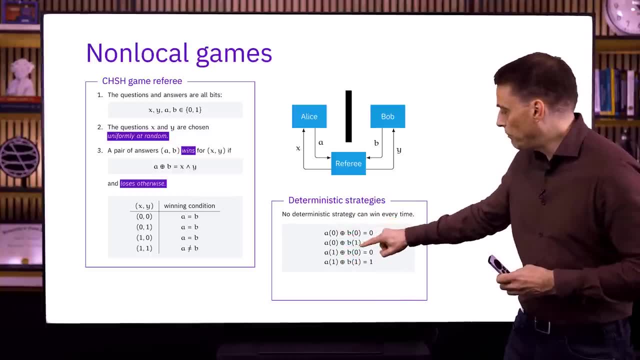 And so it follows that the exclusive or of the left-hand sides is equal to zero. That's because we have two instances of A zero, two instances of A one, two instances of B zero and two instances of A two. So XORing them all together gives us the final answer of zero. 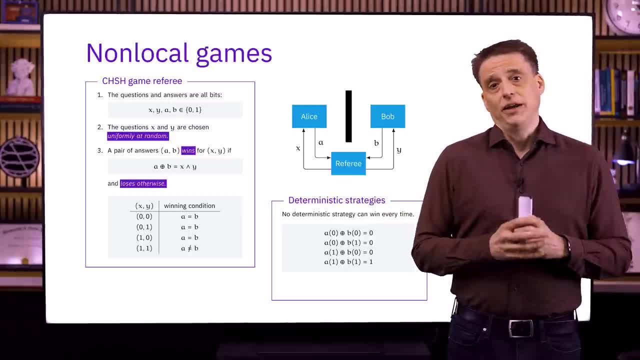 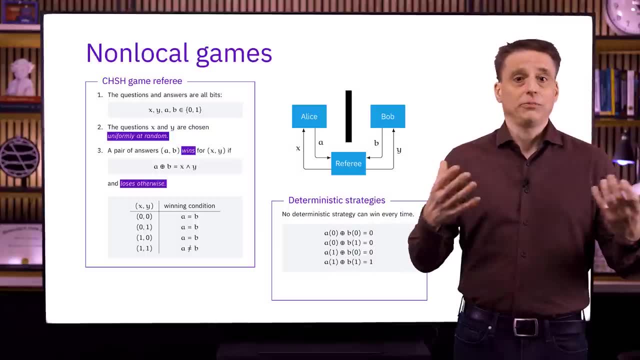 But if we take the exclusive or of the right-hand sides of the equations, we get one, not zero. So the four equations can't possibly all be true. At least one of them has to be wrong and that will lead to a loss for Alice and Bob. 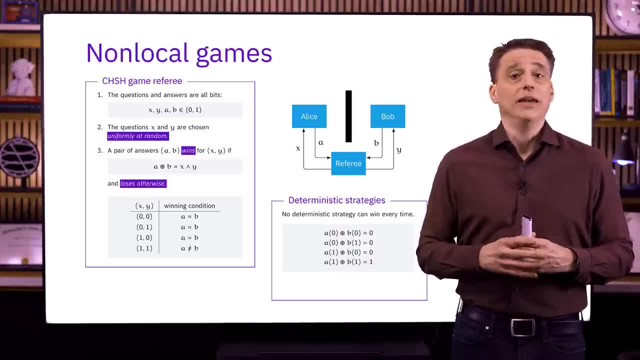 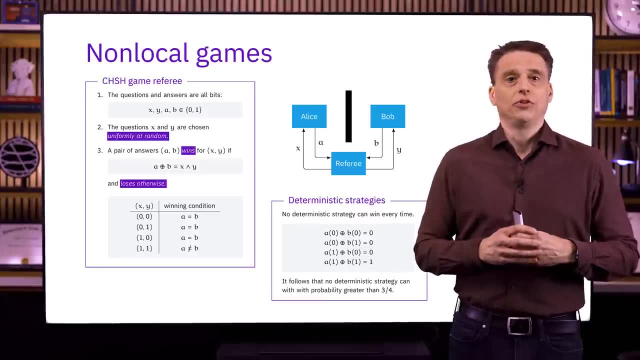 in at least one of the four cases. And so it follows- because the referee chooses the questions uniformly- that the probability of the four equations being true is equal to zero. And so it follows that the four equations are true, only that the probability for Alice and Bob 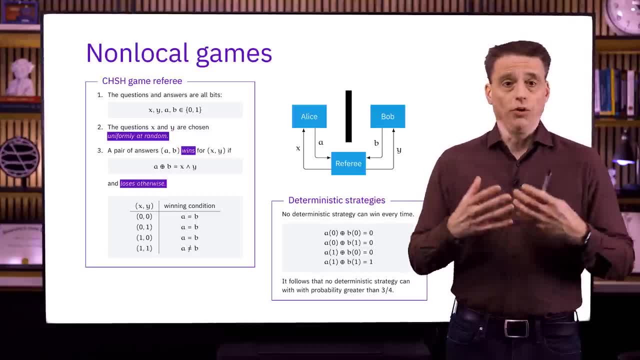 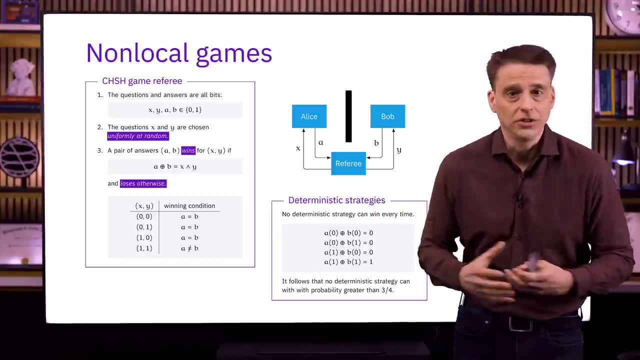 to win using a deterministic strategy is, at most, three-quarters or 75%. The fact that Alice and Bob can win with probability three-quarters is quite easy to see. actually, If Alice and Bob both answer zero all the time, for instance, they'll be correct three out of the four times. 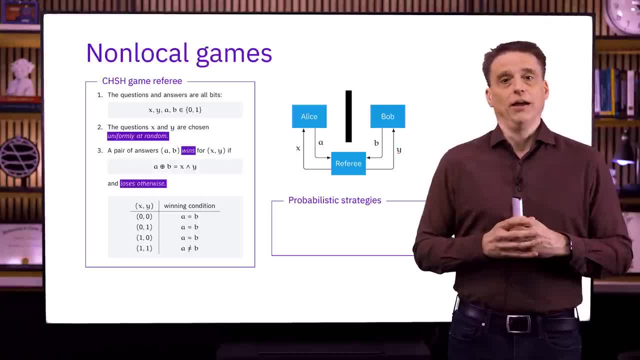 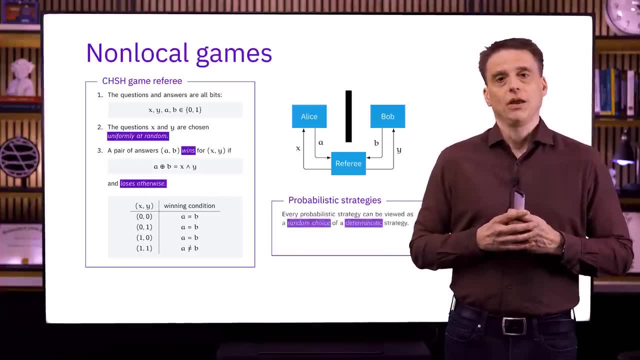 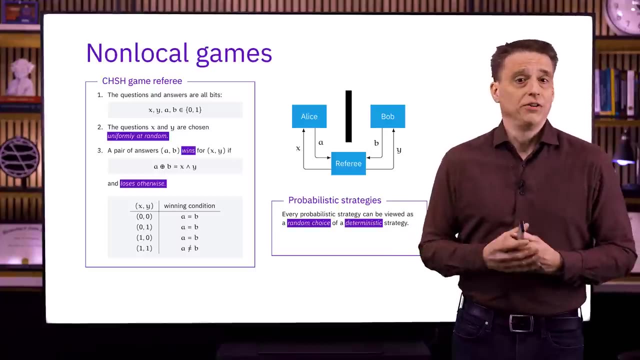 So Alice and Bob can't do any better than winning 75% of the time using a deterministic strategy. What about a probabilistic strategy? Well, it turns out that using a probabilistic strategy can't help them at all. That's because every probabilistic strategy can alternatively be viewed as: 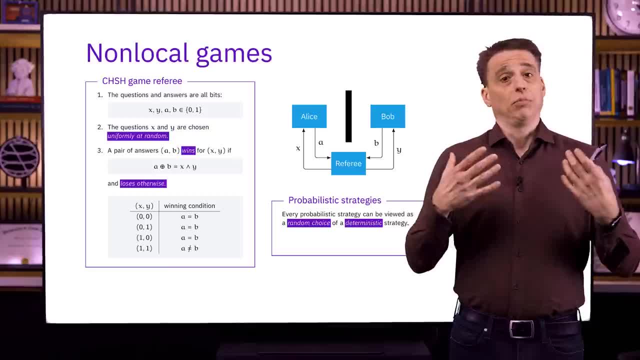 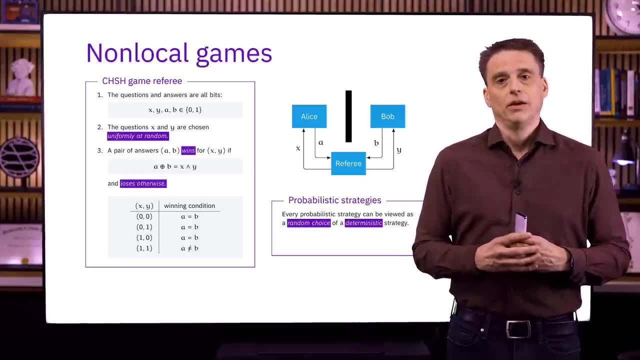 a random selection of a deterministic strategy, Just like probabilistic operations can be viewed as random selections of deterministic operations. as we saw in the first lesson, The average is never larger than the maximum, So it follows that a probabilistic strategy doesn't offer any advantage in 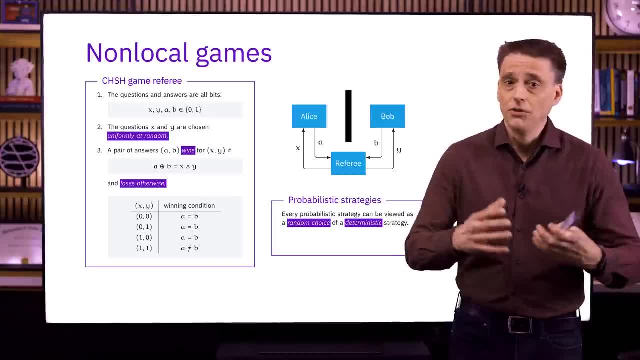 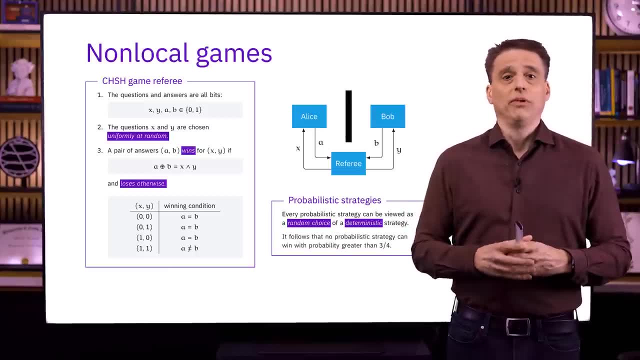 terms of winning over a deterministic strategy, And this even includes the possibility that Alice and Bob's random choices are correlated. So the bottom line is that winning with probability 3 quarters is the best that Alice and Bob can possibly do using any classical strategy. 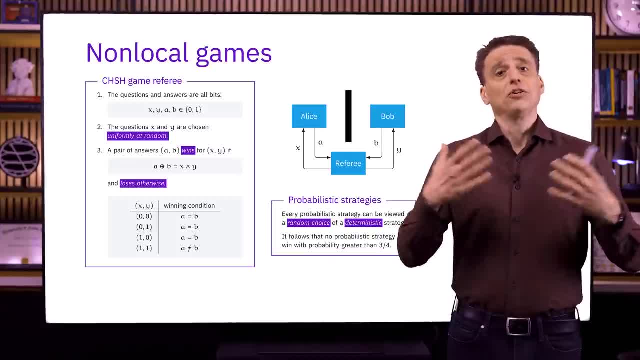 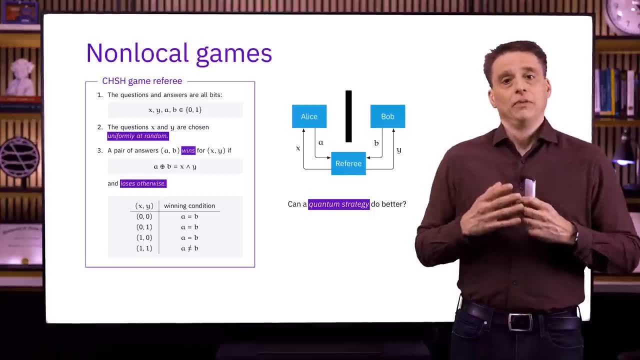 whether it's deterministic or probabilistic. The natural question to ask at this point is whether Alice and Bob can do any better using a quantum strategy And, in particular, if they share an entangled quantum state which they could have prepared prior to. 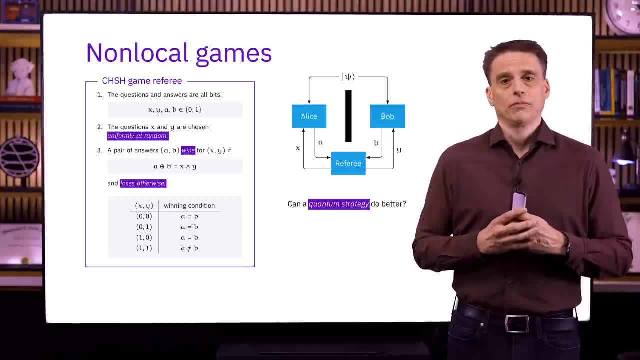 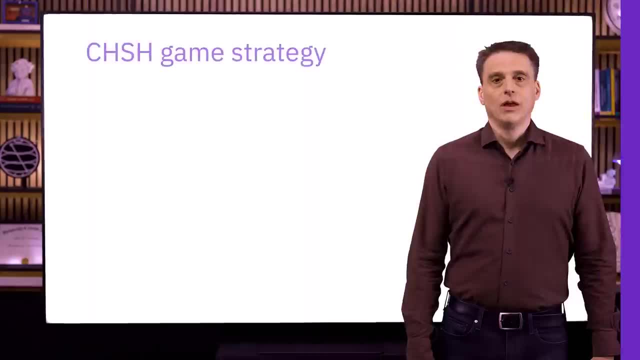 after playing the game. can that help them? The answer is yes, it can, And that is the point of the example and that's why it's so interesting. So let's see exactly how Alice and Bob can do better in this game using entanglement. 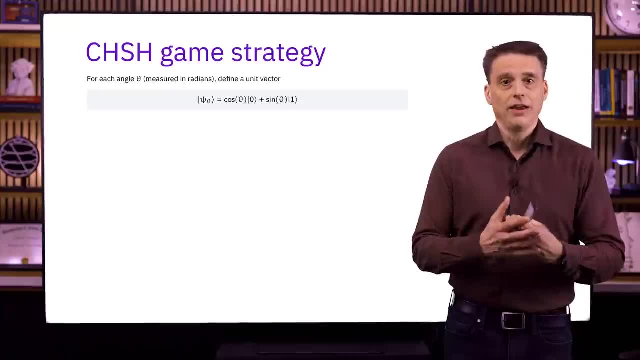 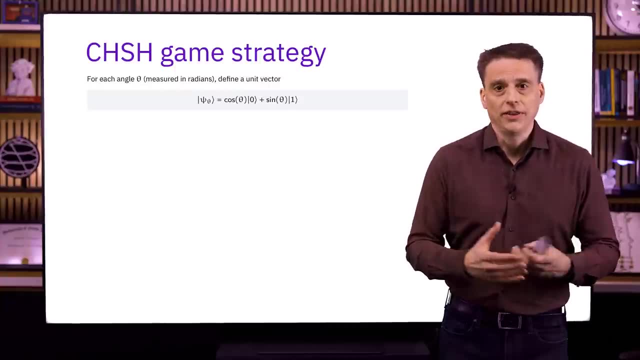 The first thing we need to do is to define a quantum state vector, psi theta, for each angle theta, as you can see here on the screen. So psi theta is equal to cosine theta times cat zero, plus sine theta times cat one. 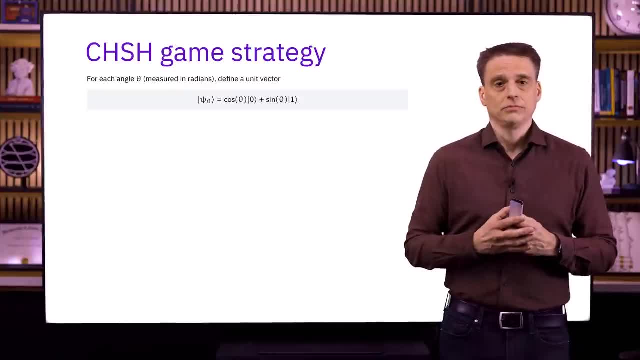 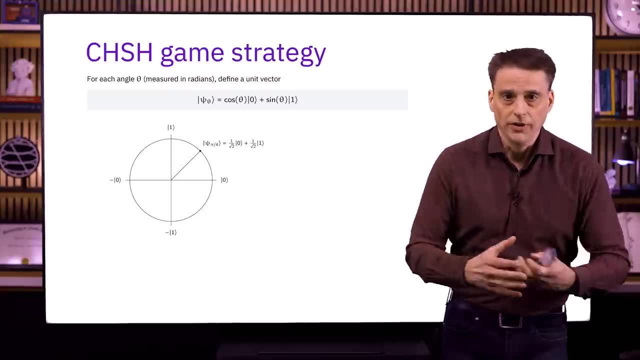 And here, by the way, we're thinking about angles in terms of radians. So, for example, here's the vector we get when theta is equal to pi over four, which is 45 degrees. Cosine of pi over four and sine of pi over four are both equal to 1 over. 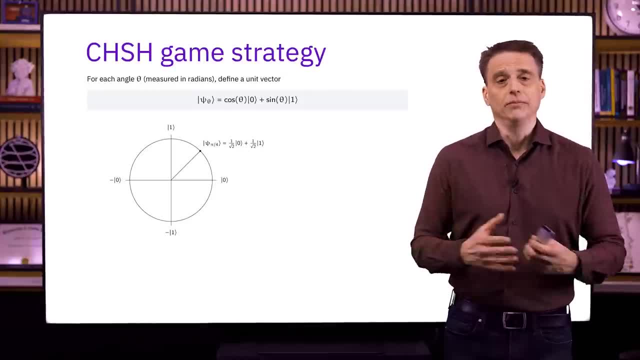 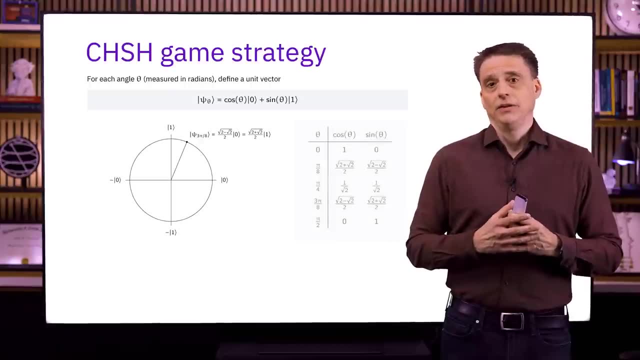 the square root of 2, so this is just another name for the plus state. Here's another example when theta is equal to three times pi over eight. And in case you don't have that, then you can use the plus state. don't happen to know the sine and cosine of 3 times pi over 8 off the top of your head? 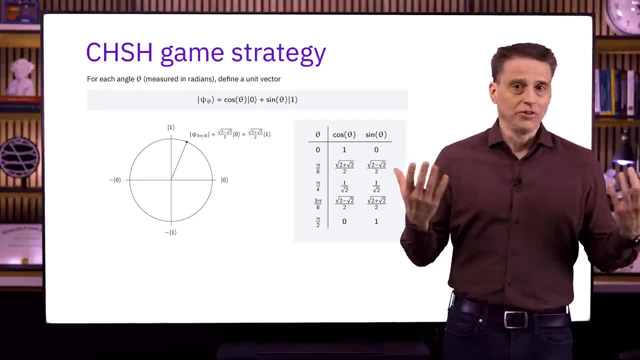 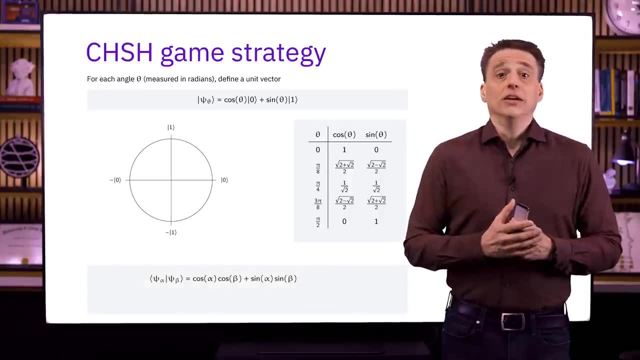 here's a table of the sines and the cosines that we're actually going to need throughout this example, and includes the ones that we need for this particular vector. Now, if we want to take the inner product between any two of these vectors for angles alpha, 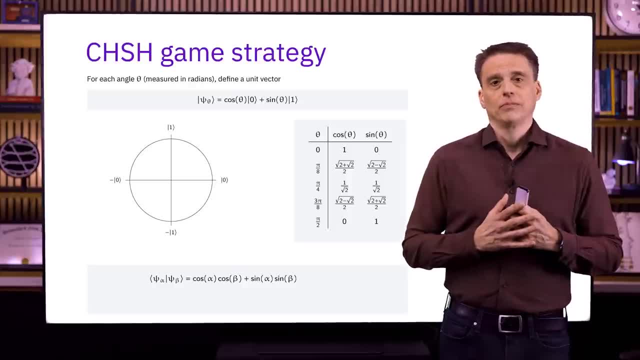 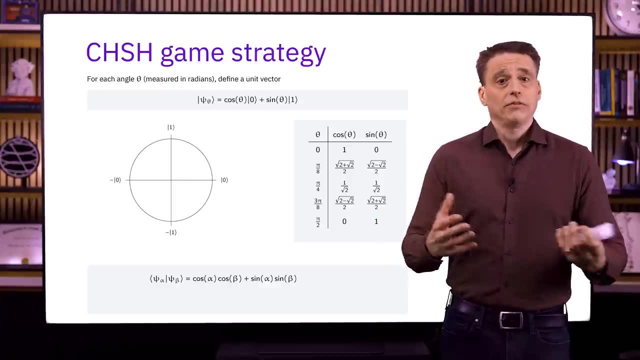 and beta. let's say it's straightforward to do that. We only have real number entries in these vectors, so there are no complex conjugates to worry about and we obtain the product of the cosines plus the product of the sines. 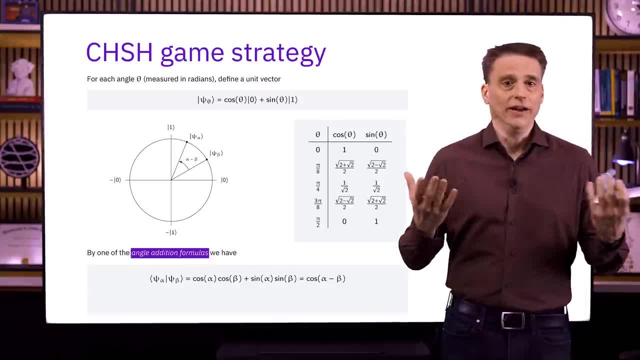 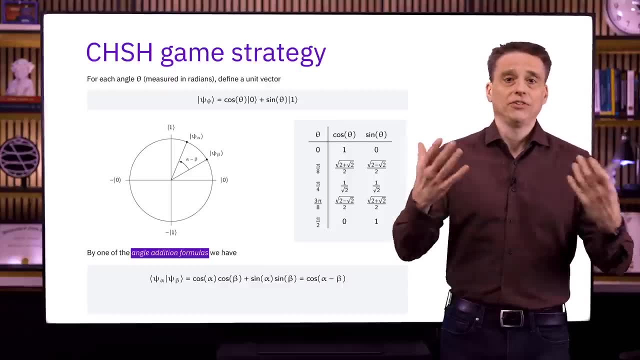 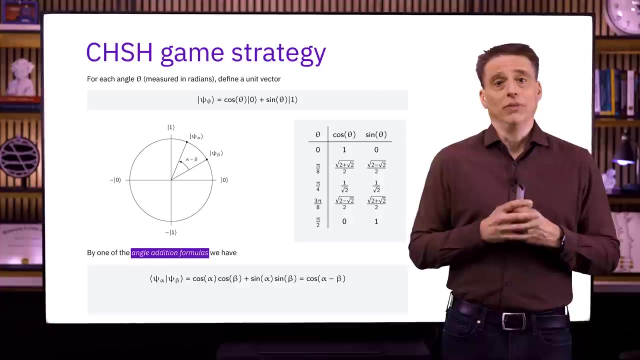 And we can use one of the so-called angle addition formulas to simplify that. It's the cosine of the difference between the angles And because the cosine function is symmetric around zero, it doesn't actually matter which order we take them in If you don't have these sorts of trigonometric identities committed to memory. by the way, 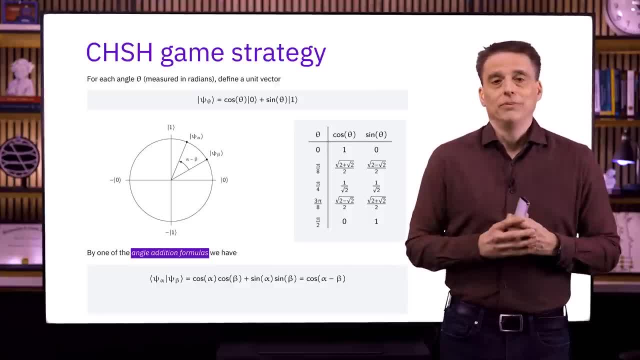 you're not alone, But you don't have to remember them, you can just look them up. This one does make sense, though, when you think about the G-shape. This is the geometric interpretation of the inner product between real unit vectors as: 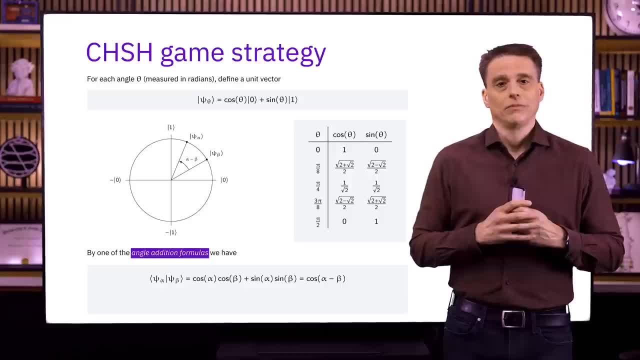 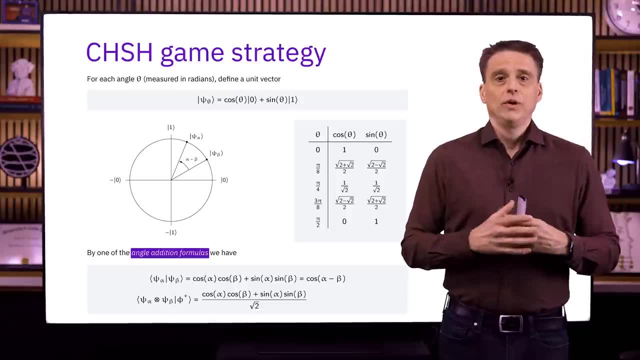 the cosine of the angle between them. If we compute the inner product of the tensor product of any two of these vectors with the phi-plus state, we get a similar looking expression, except that there is a square root of 2 in the denominator. 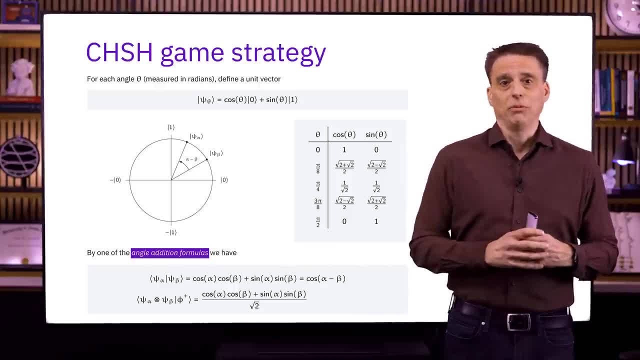 This is the first time that the phi-plus state has appeared in the context of this example, by the way, and we'll see exactly why we're interested in this particular inner product shortly, But for the moment, let's just imagine that this is the first time that the phi-plus state. 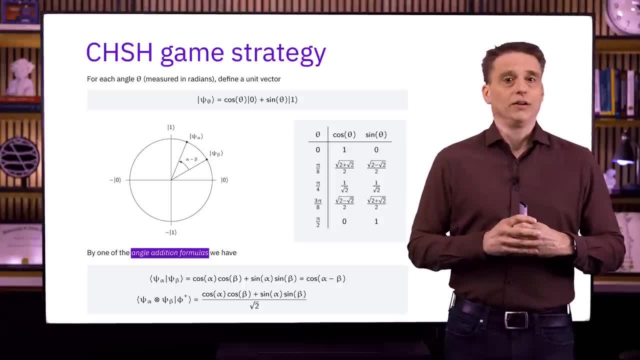 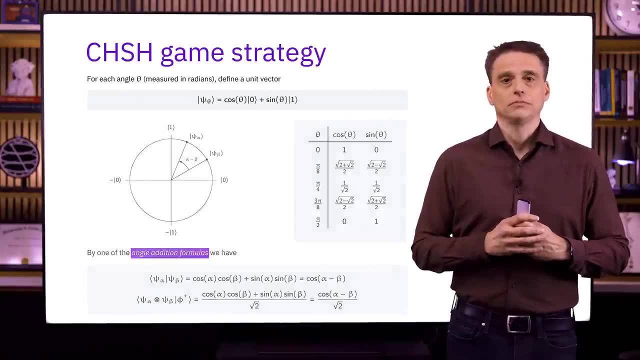 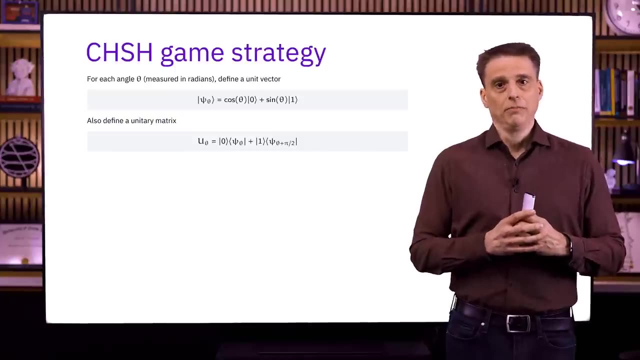 has appeared in the context of this example. We just observe that we obtain the same expression that we had for the inner product divided by the square root of 2. And so we can simplify as before. Next, we'll define a unitary matrix- u-theta- for each angle theta, like you see right here. 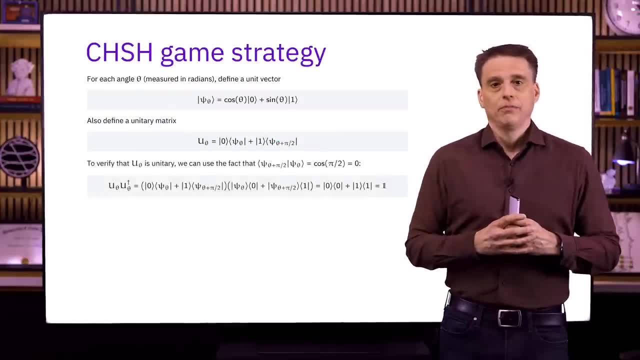 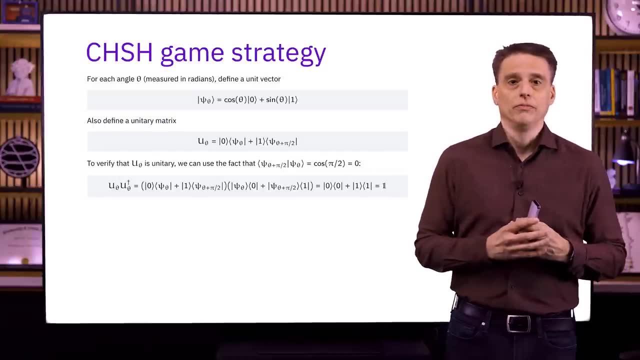 It's not difficult to check that this is indeed a unitary matrix. The key thing we need to recognize is that the vector psi-theta is orthogonal to the vector psi-theta-plus-pi-over-2. And that makes sense because if we rotate by pi-over-2, which is 90 degrees, we get an 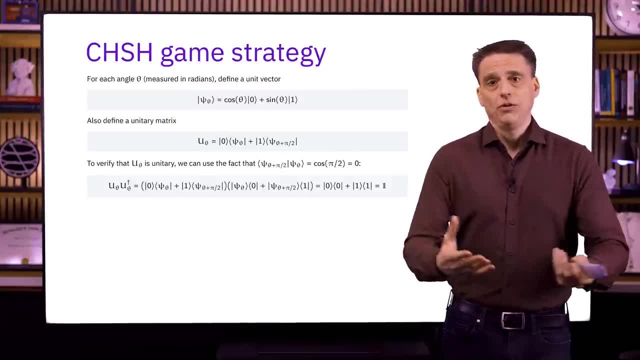 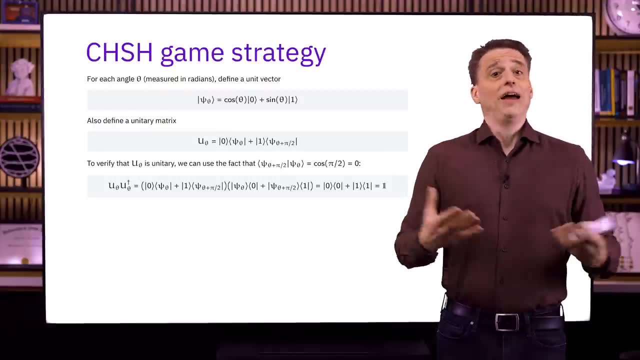 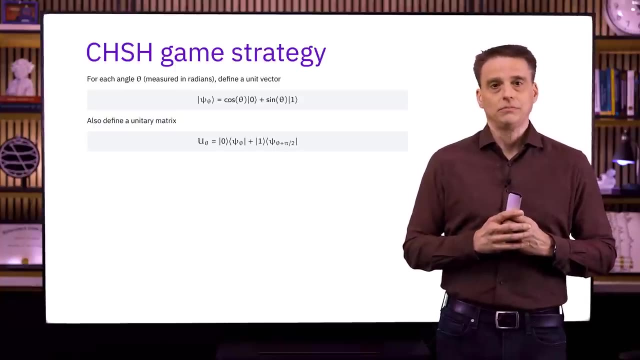 orthogonal vector. If we then multiply u-theta to u-theta-dagger, we get the identity matrix. Intuitively speaking, what this matrix does as an operation is to map psi-theta to ket-zero and psi-theta-plus-pi-over-2 to ket-one. 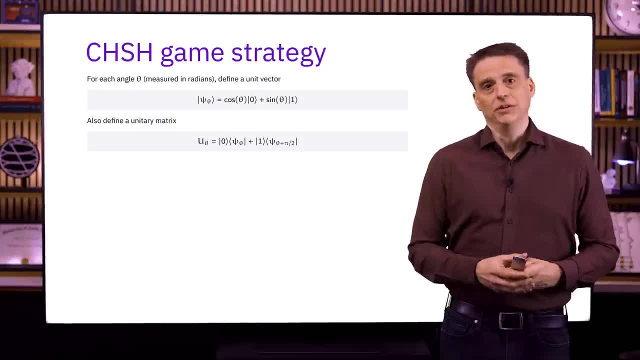 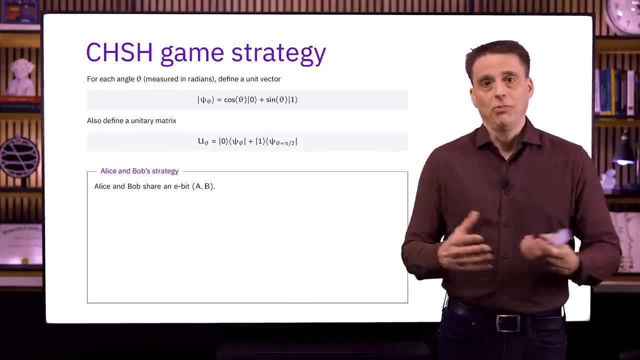 At this point, we have everything that we need to describe Alice and Bob's strategy, So let's start with the first one. First, just like we had for teleportation and superdense coding, Alice and Bob will start out by sharing an e-bit. 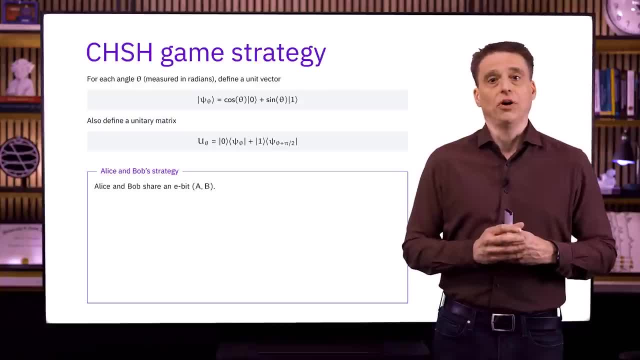 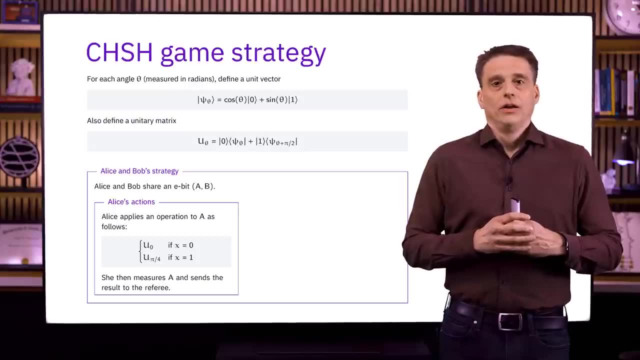 Alice holds a qubit a, Bob holds a qubit b and together the two qubits are in the phi-plus state. Alice's actions are as follows: She looks at the bit x that she receives from the referee and if x is equal to zero, she. 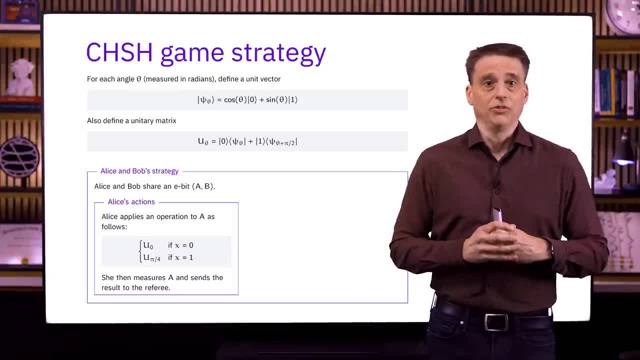 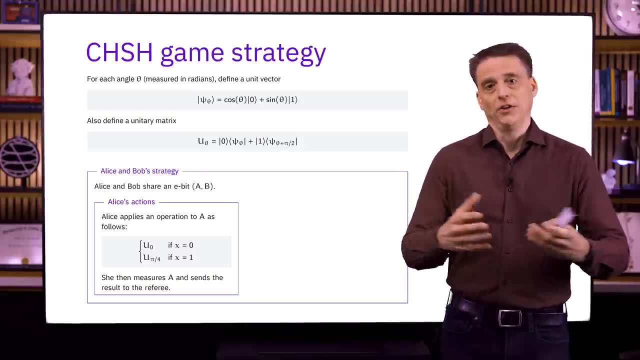 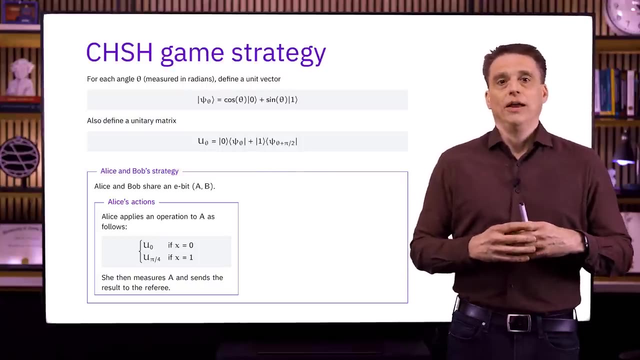 performs u-zero on a, which happens to be the same thing as doing nothing, because u-zero is the identity matrix If x is equal to one. on the other hand, she applies u-pi-over-4 to a. After she applies one of the two operations, she measures a using a standard basis measurement. 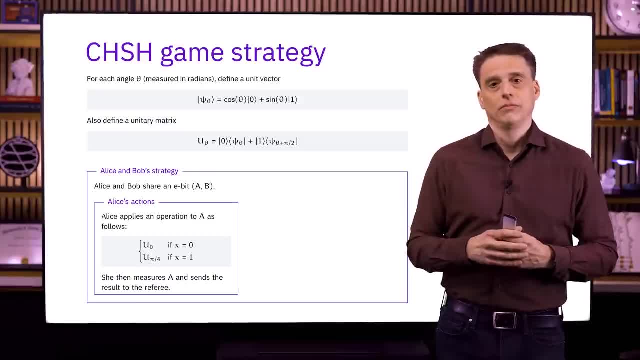 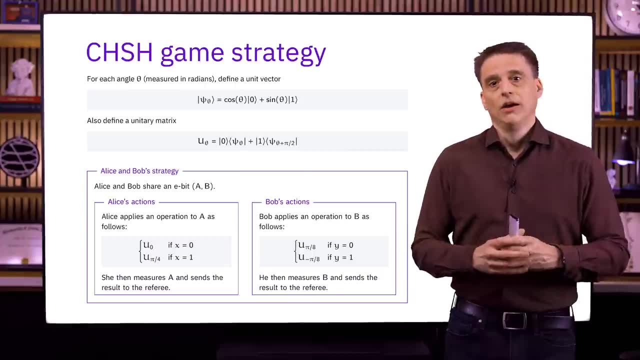 and sends whatever result she gets to the referee. Bob does something very similar. His qubit is called b, of course, and he receives y from the referee as opposed to x, but the key difference is that he uses different angles for his unitary operations. 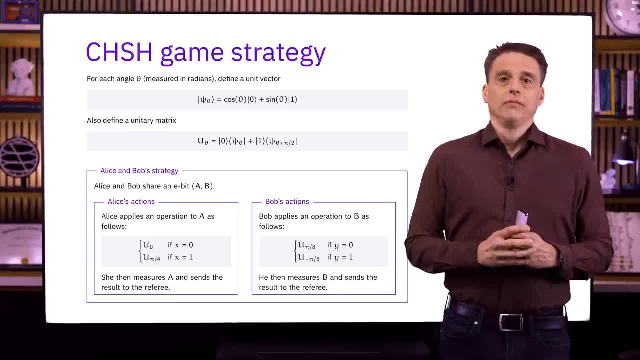 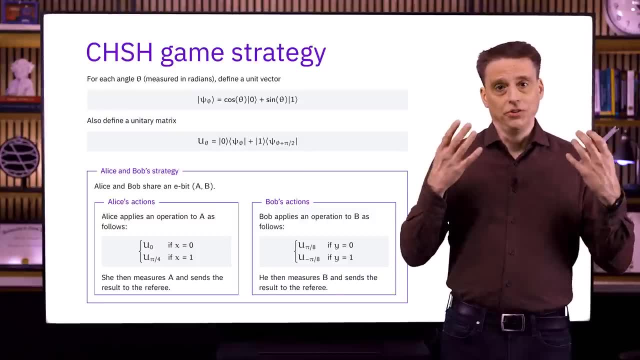 If y is equal to zero, he applies u-pi-over-8,, and if y is equal to one, he applies u-negative-pi-over-8.. And we'll see why these choices of angles are good choices shortly. It's not at all obvious. 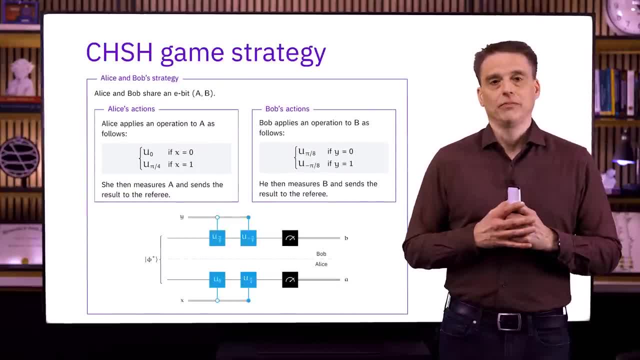 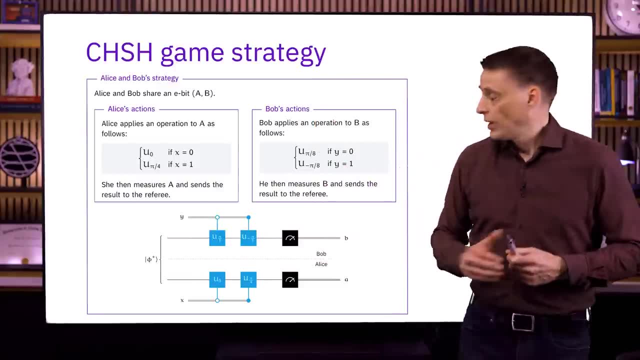 And here is a circuit diagram that expresses this strategy. Bob is on the top and Alice is on the bottom. this time, Here is the e-bit that is coming in, and these are the unitary gates that Alice and Bob might or might not apply. 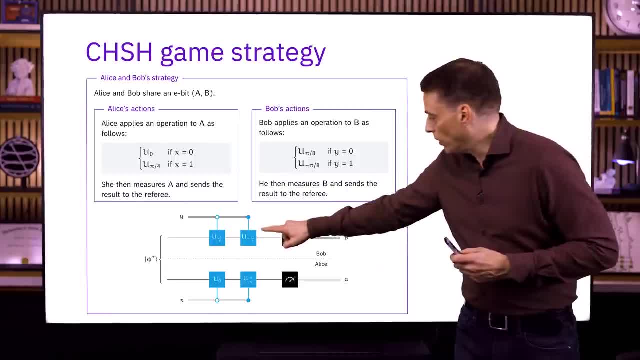 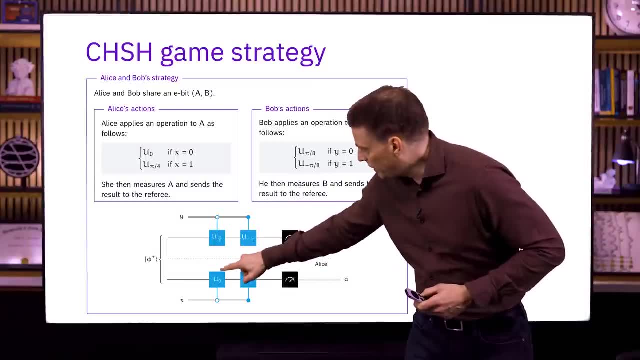 For this one and this one we have gates that are being controlled either by the bit x or by the bit y, And for these two right here we have what kind of look like control gates, except that the circle isn't filled in. 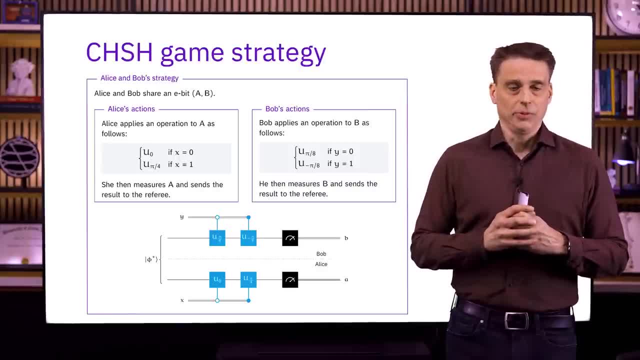 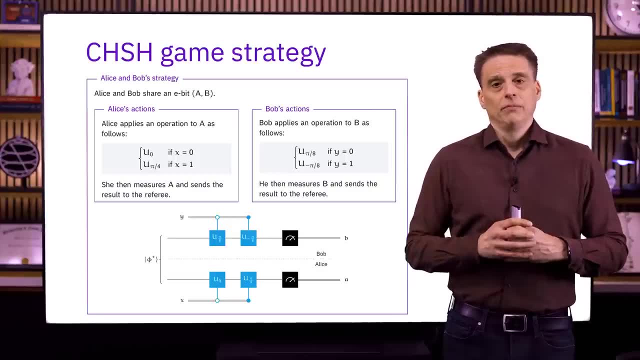 And what this means is that if the control bit is set to zero, then the gate is performed, and if the control is set to one, then nothing happens. So it's just like an ordinary control gate, except that the roles of zero and one for 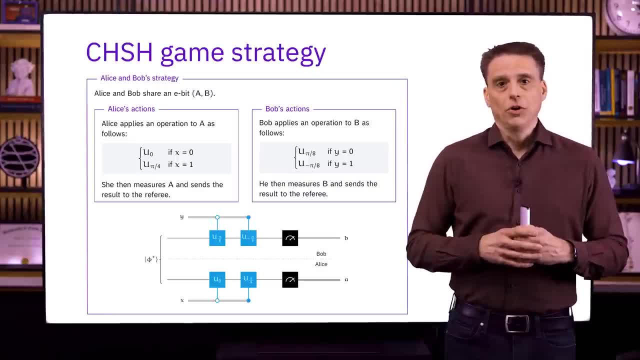 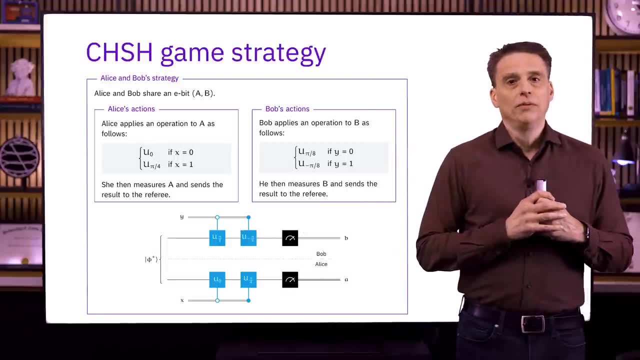 the control are swapped So effectively. Bob performs this gate right here if y is equal to zero, and he performs this gate right here if y is equal to one. And similarly, Alice performs this gate right here if x is equal to zero, and this gate. 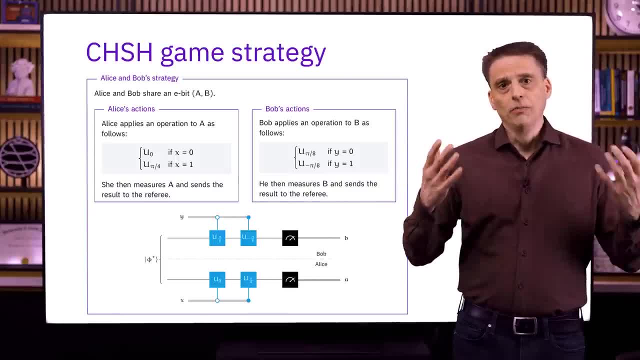 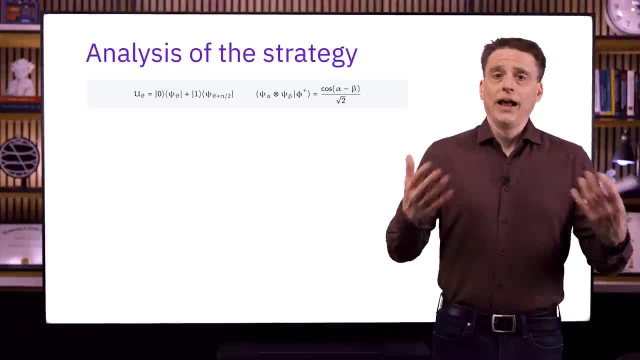 right here if x is equal to one. So that is Alice and Bob's strategy, And now we just need to figure out how well it works. For the analysis of the quantum strategy that I just described, we really only need two things at this point. 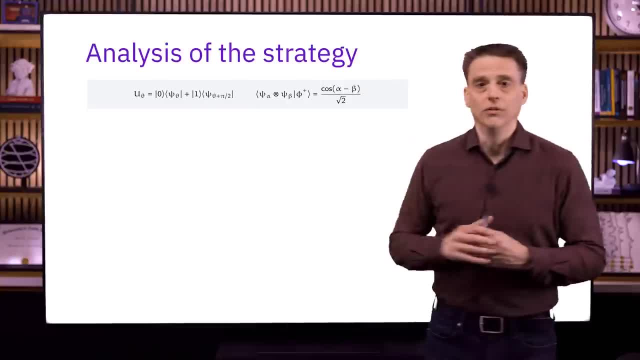 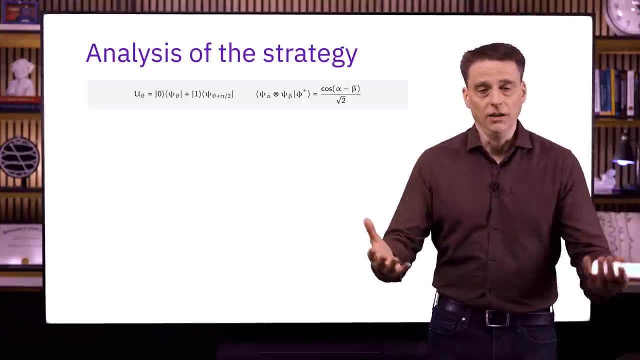 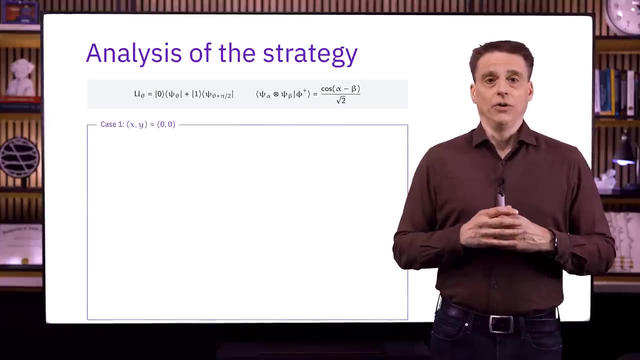 First, the unitary matrix u theta is, as you see, right here, and second, we had this formula. We don't actually even need the definition of the vector psi theta anymore. These two equations are all we need. There are four cases to consider, starting with case one, which is that x equals zero. 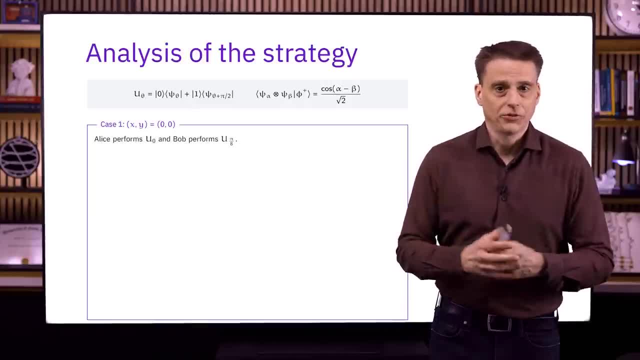 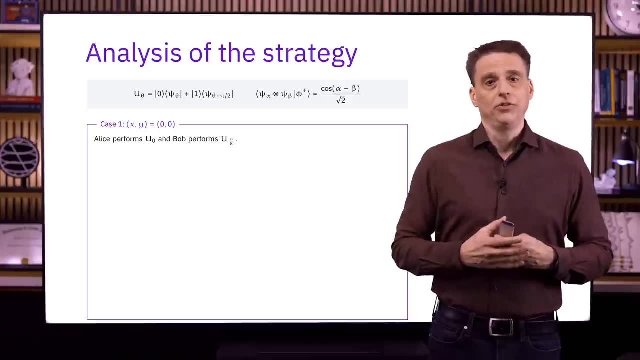 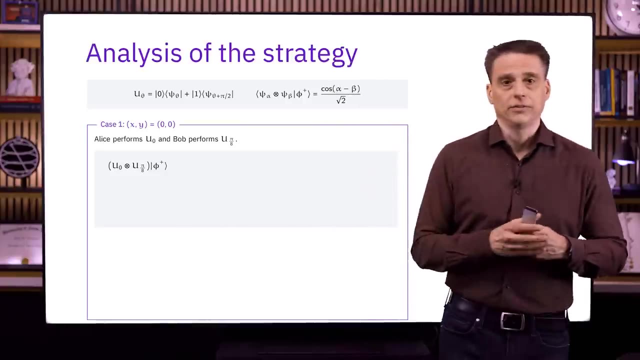 and y equals zero. And if we look back at the strategy, we'll find that in this case, Alice performs u zero on her qubit and Bob performs u pi over eight on her qubit. Remember, Alice is on the bottom and Bob is on the top, so their state looks like this. 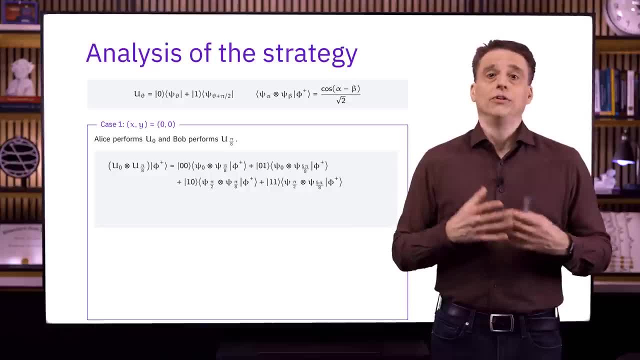 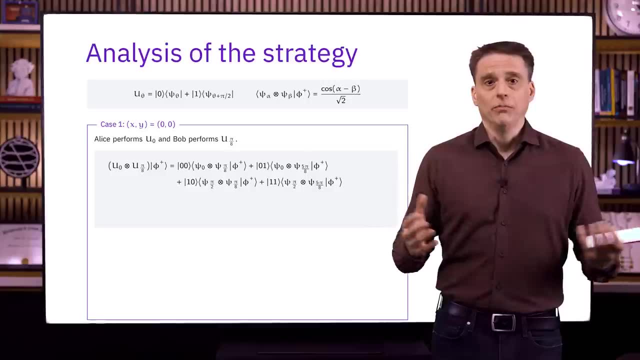 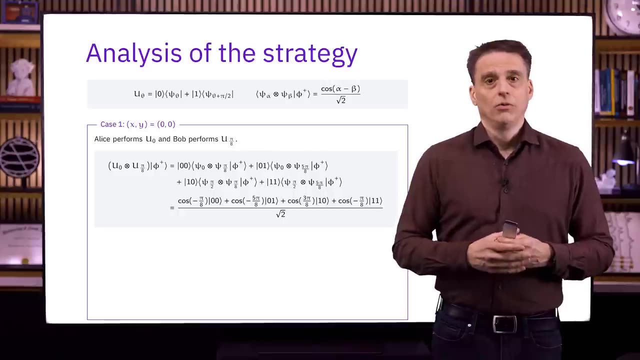 And by expanding that out according to the definition of u theta, we get this expression right here. We don't need to expand that out any further because we have the other formula to help us out, And if we apply that formula for each of these four terms, what we get is this: 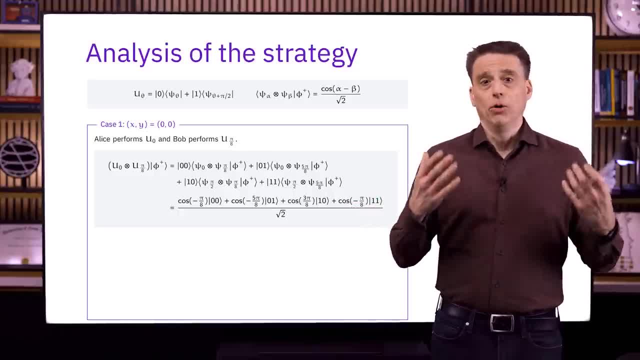 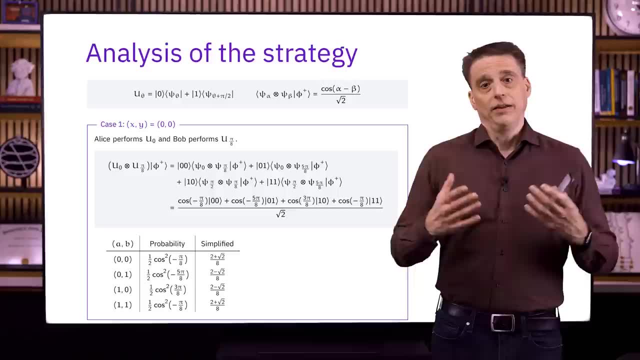 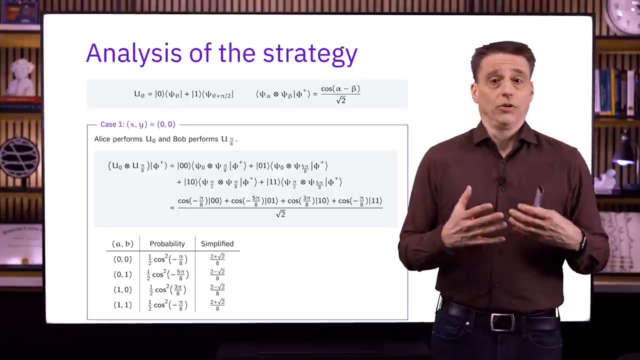 Science. All right, This is it. At this point, Alice and Bob both measure and here's a table that explains the distribution of the outcomes. We take the absolute value squared of the coefficients to get the probabilities, which happens to be the squares of the coefficients, because the coefficients 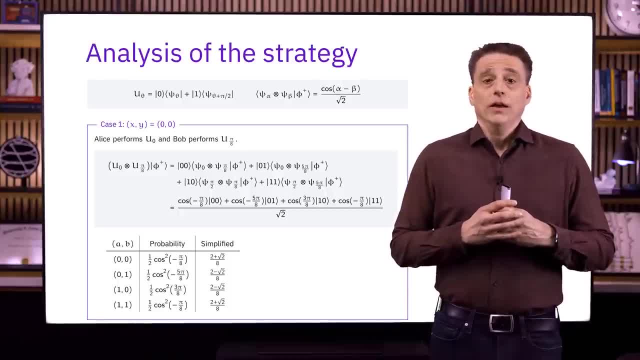 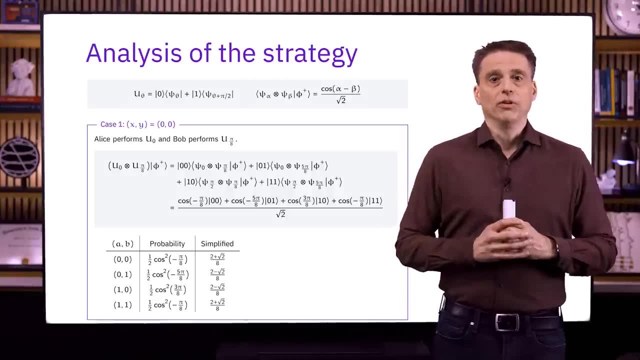 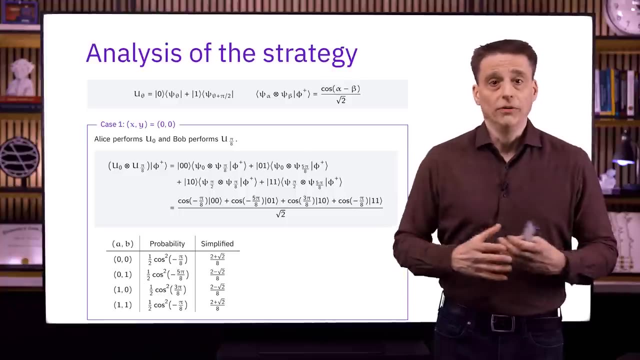 are all real numbers. in this case, If we make use of the sine and cosine values from earlier in the lesson, along with some symmetries, we can express these probabilities as we have right here in the last column. Now, what we really care about is the probability that they win. 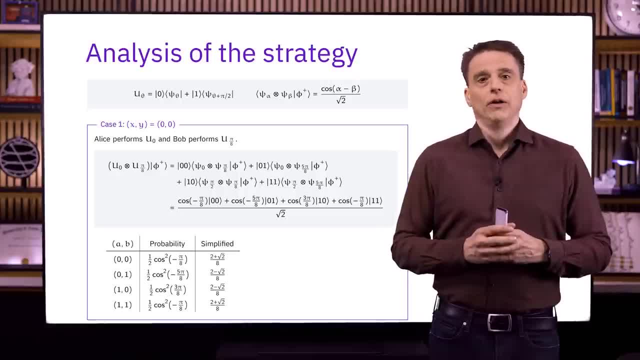 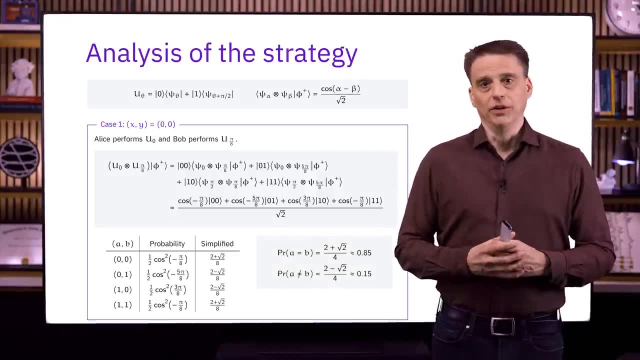 and remember that in the case that x and y are both zero, they win if a and b are equal and they lose if a and b are not equal. If we calculate those probabilities, we find that the probability that a and b are equal is the sum of this number and this number. 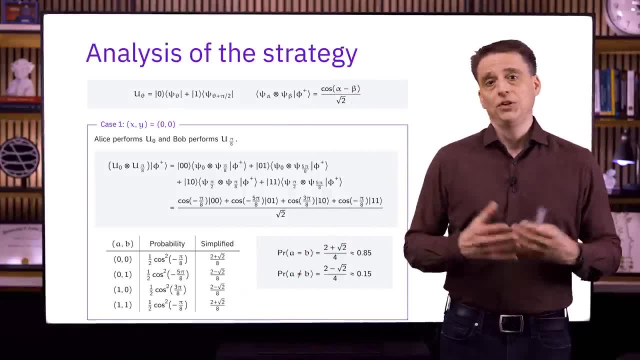 which is equal to 2 plus root 2 all over 4, which is about 80.. So we have 85 percent. The probability that a and b are not equal is 2 minus root 2 all over 4, which is naturally 1 minus the quantity that we just calculated. 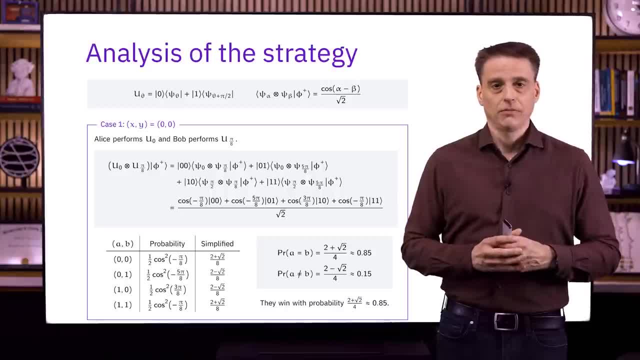 So they win with probability about 85 percent in this case. There are three more cases to consider, but they're all very similar to this one. In the case that x equals 0 and y equals 1, Bob applies u negative pi over 8,. 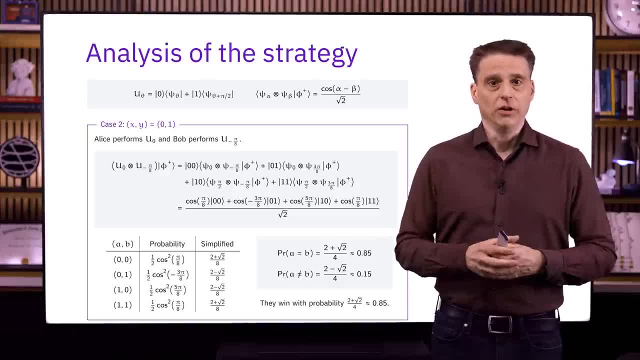 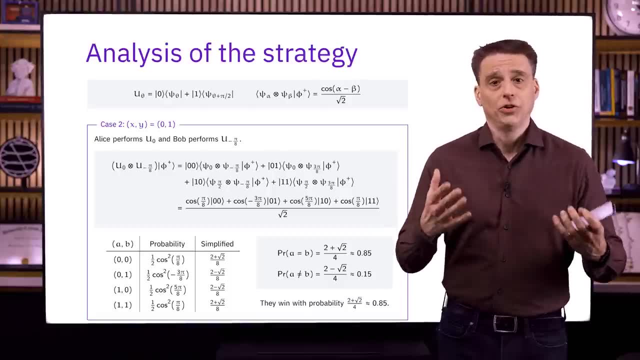 rather than u pi over 8.. The values in the formulas change somewhat, but we end up with exactly the same probabilities that we had in the previous case. When x equals 0 and y equals 1, Alice and Bob still win when a and b are equal. 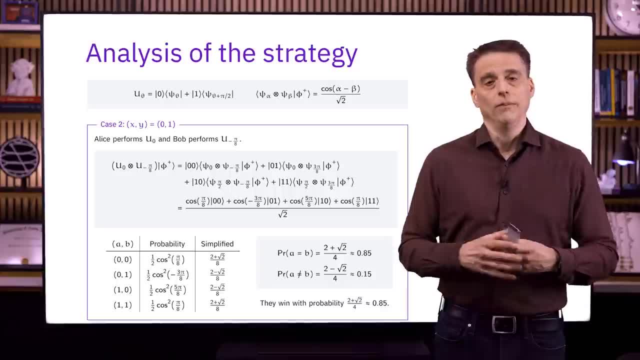 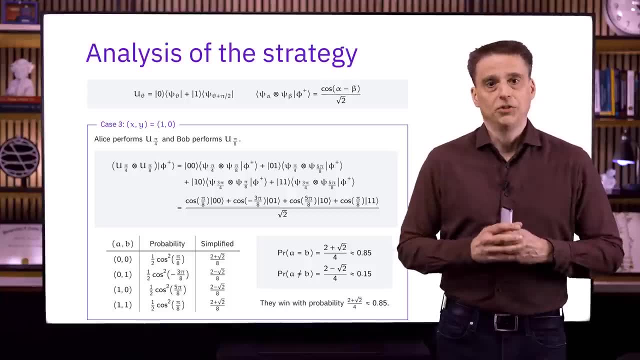 and so we have exactly the same winning probability as before. In the third case, when x is equal to 1 and y is equal to 0, we have a similar situation. The angles are different, but they have exactly the same relationship to one another. 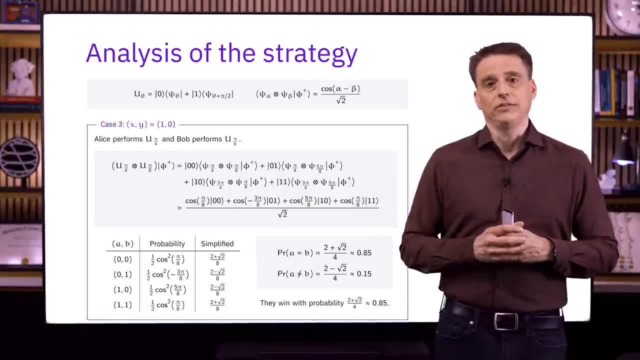 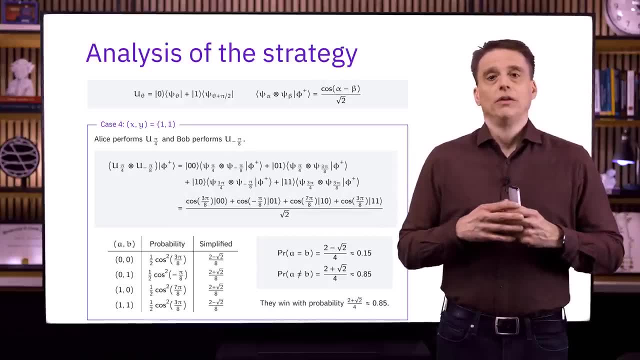 and in fact we do get exactly the same vector that we got in the previous case. So the probabilities are the same and so is the winning probability. The last case is a little bit different, as we might expect, because the winning condition is different in this case. 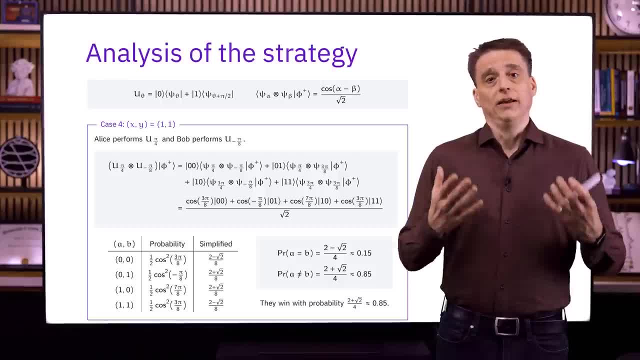 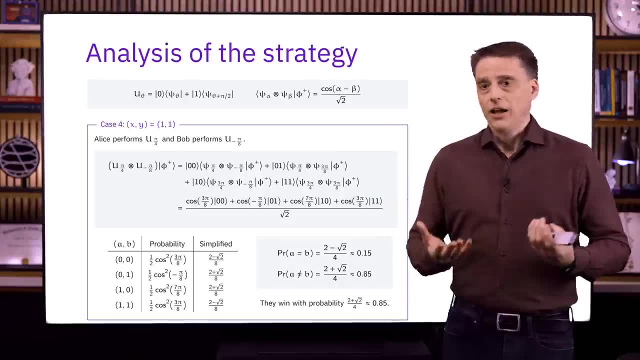 When x and y are both equal to 1, Alice and Bob win when a and b are different. The basic method is the same, although the angles are different. This time we get this vector right here And you can check that by going through the required subtractions. 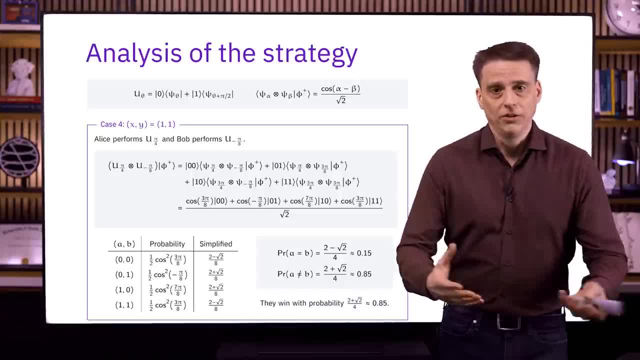 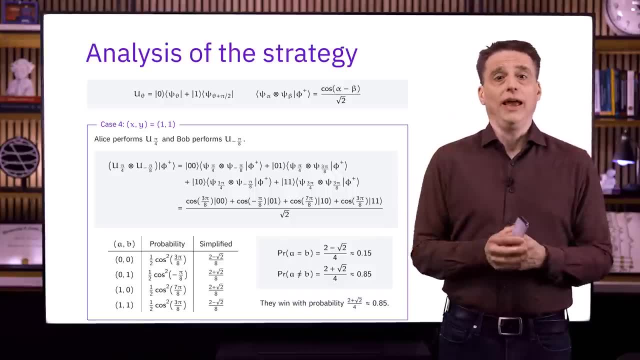 The probabilities do change. finally, and if we look up the values that we need, we see that the probabilities have effectively swapped positions from before. So this time it's the probability that a is not equal to b that is the larger of the two. 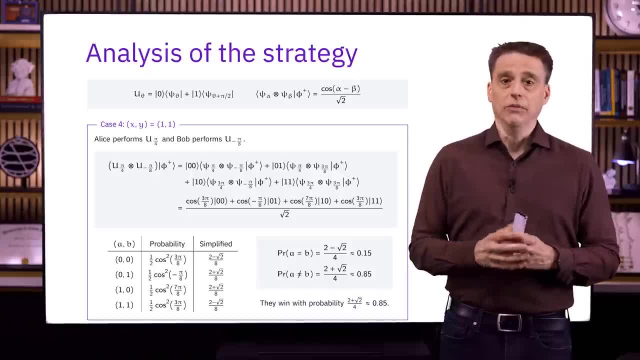 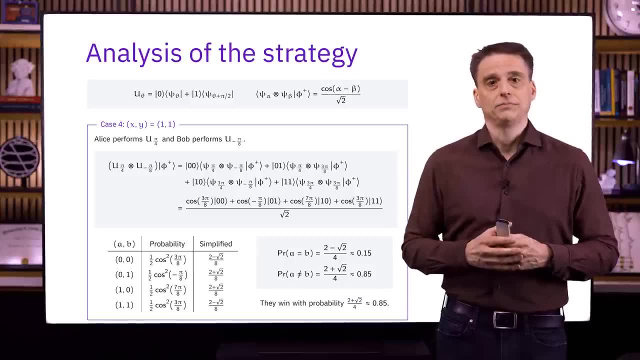 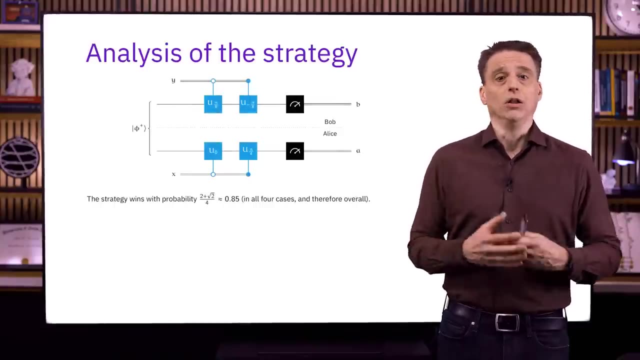 But that's good, because in this case Alice and Bob win when a and b are not equal. So once again they win, with probability approximately 85%. Given that they win in every case with the same probability, which is 2 plus root 2, all over 4,. 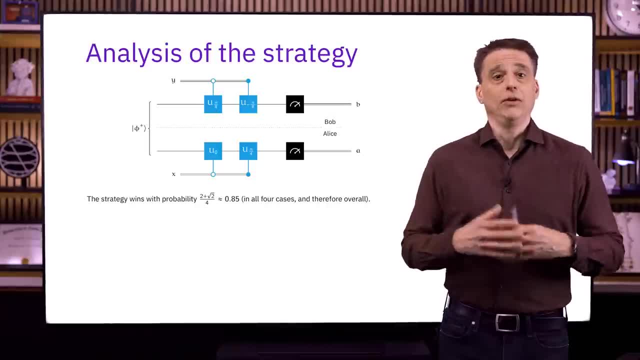 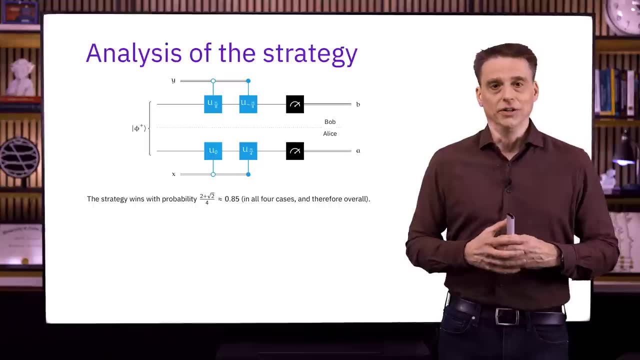 or about 85%. that's the probability that they win. overall. That's better than any classical strategy can do for this game, and that's what makes it interesting. This happens to be the optimal winning probability for any quantum strategy. You can't do any better than this using any entangled state. 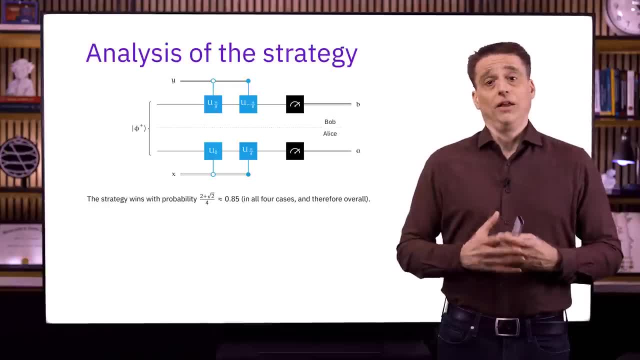 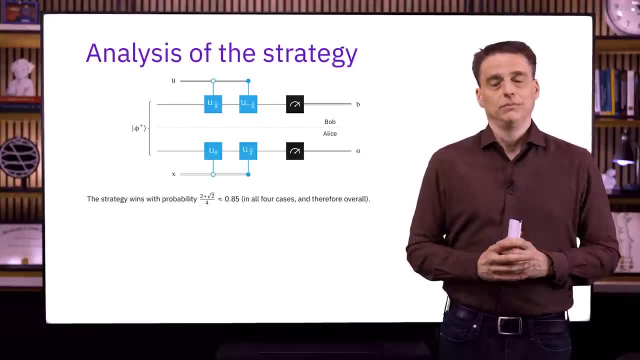 That fact is known as Searleson's inequality. It's named for Boris Searleson, who first proved it and, to my knowledge, was one of the first people to describe this example as a game In case. the analysis that we just went through seems a little bit mysterious. 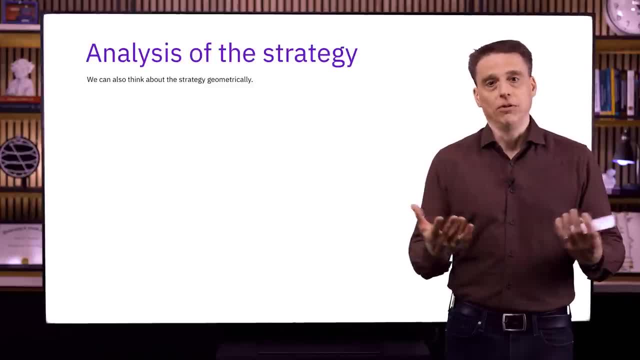 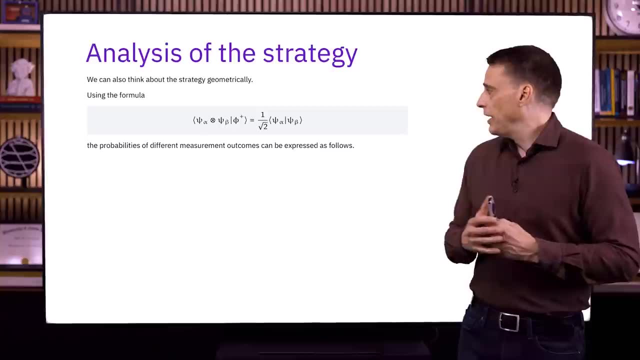 it's possible to think about it geometrically, which might be helpful to give you a better sense for the choice of the angles, Specifically, if we use the formula that you see right here, which we can easily deduce from the expressions we already found for the inner products involved. 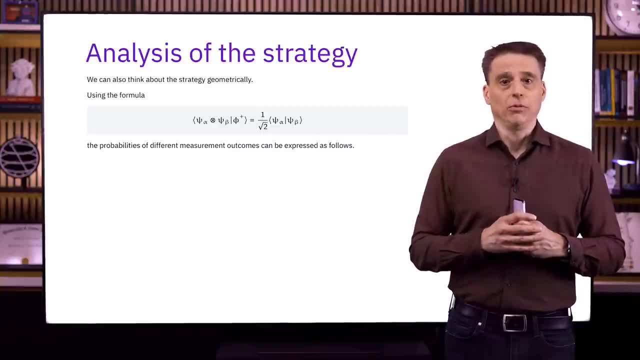 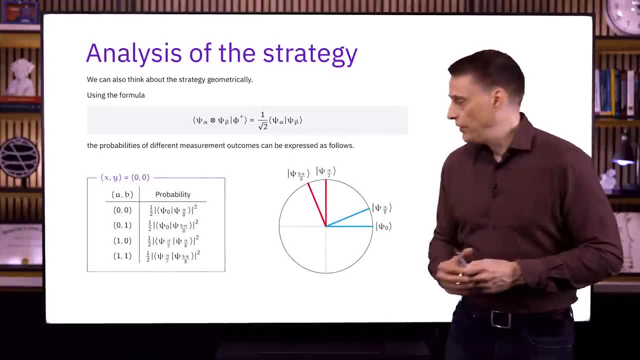 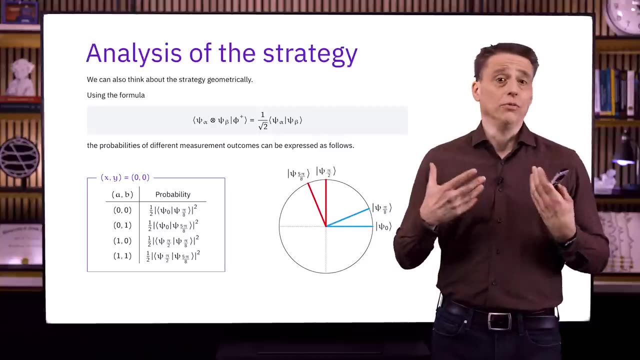 then we can alternatively express the probabilities of the different possible measurement outcomes in the four cases as follows. First, if xy equals 00, then these are the probabilities of the various measurement outcomes, and you have to either think back or look back at the analysis that we just went through to conclude that, using our formula, 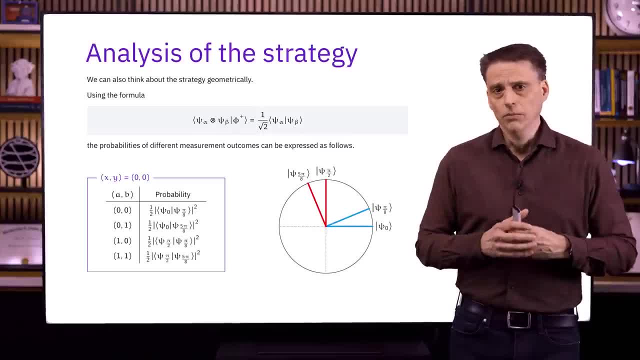 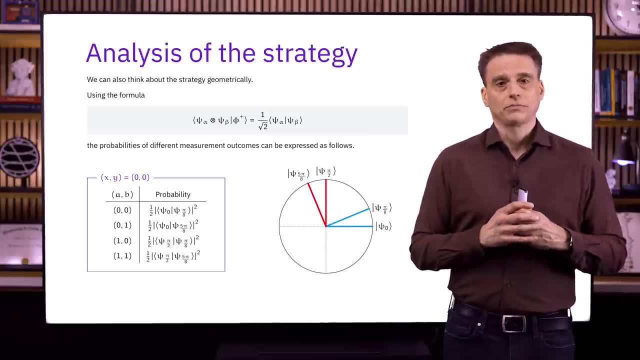 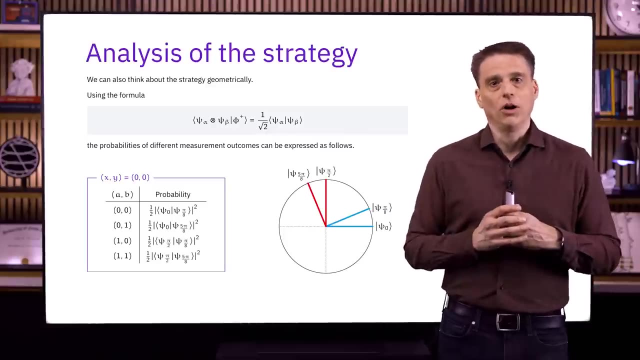 Over here we can see the different state vectors drawn as they were before, and the color-coding here is that blue corresponds to the outcome 0, and red corresponds to the outcome one. You can see that the angle between the blue vectors and the angle between the red vectors is relatively small. 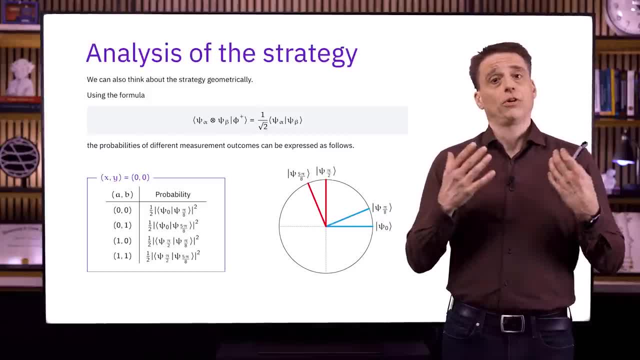 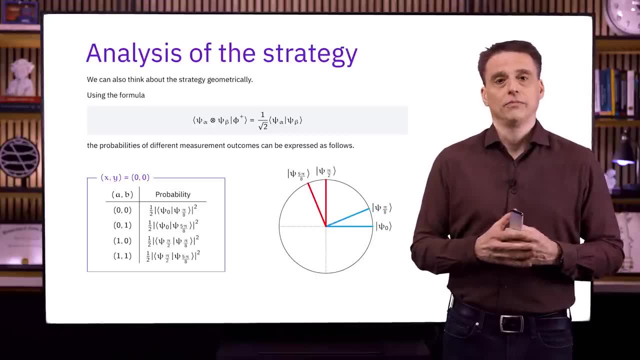 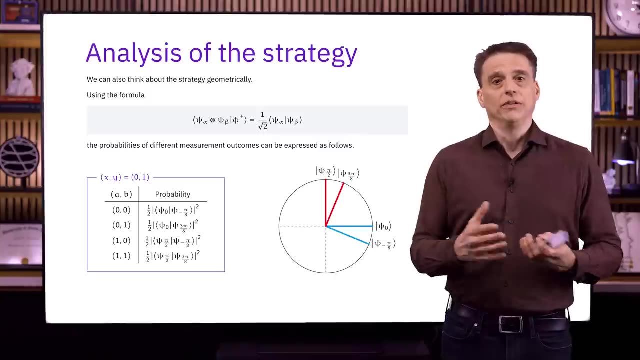 It's pi over eight in both cases. So the cosine is relatively large And that means that the probability that the two outcomes are equal is relatively large. In the case that x- y equals zero one, it's a similar situation The angles between the vectors having the same color. 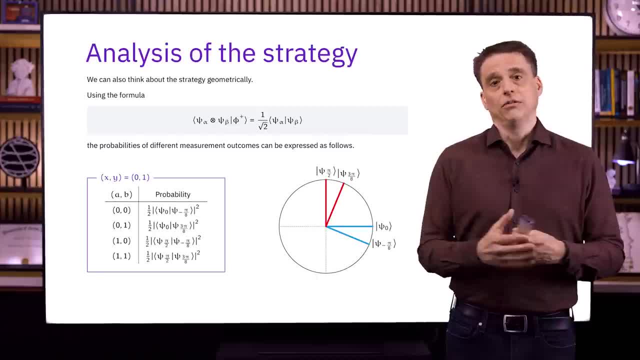 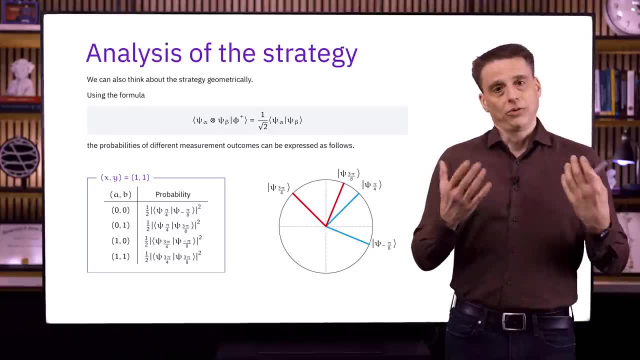 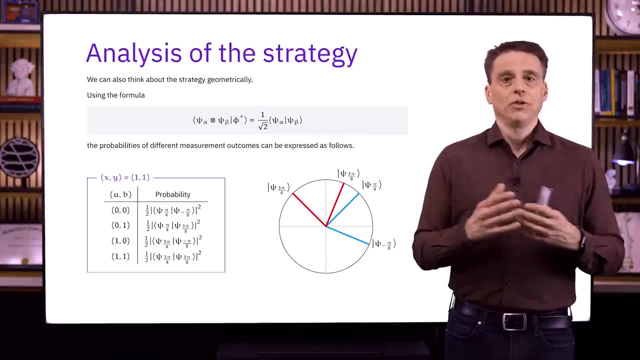 is small, so the probability of equal outcomes is again relatively large. The third case is similar, And in the fourth case, when x- y equals one one, something interesting happens. This time just by the way these vectors have been chosen. 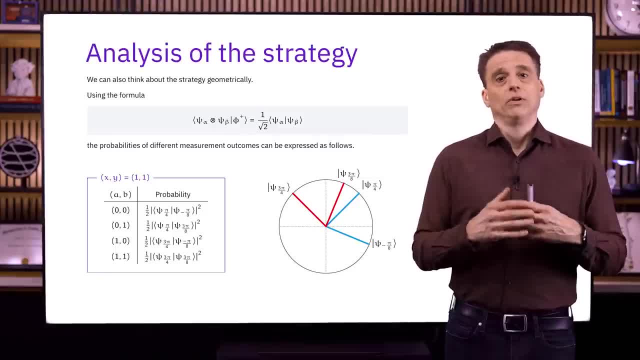 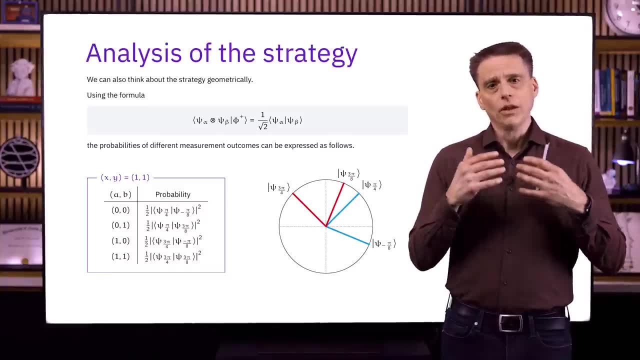 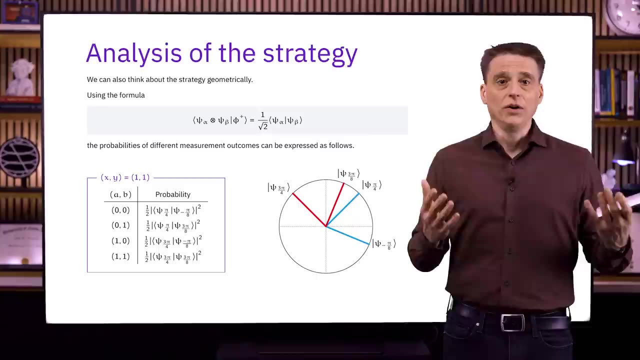 we see that the angles between vectors having the same color are relatively large And specifically, the angles are three times pi over eight in both cases. This means that the probability that the measurement outcomes is equal is relatively small, But this is the one case in which Alice and Bob win. 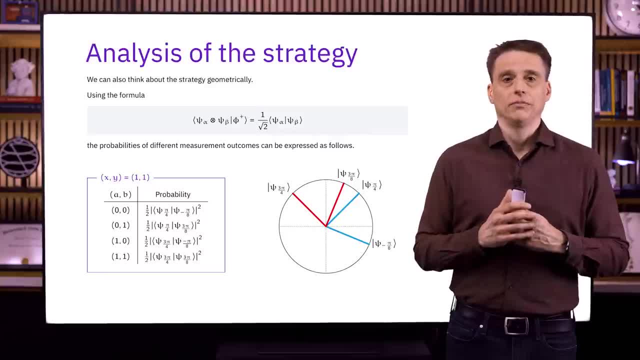 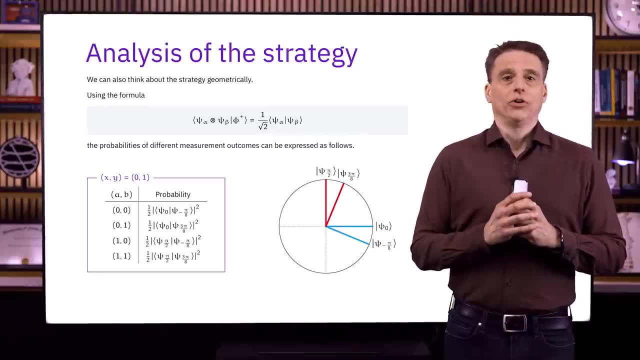 when their answers disagree. So it's what we want Once again. here are the vectors: When x- y equals zero zero. when x- y equals zero one. when x- y equals one zero and when x- y equals one one. 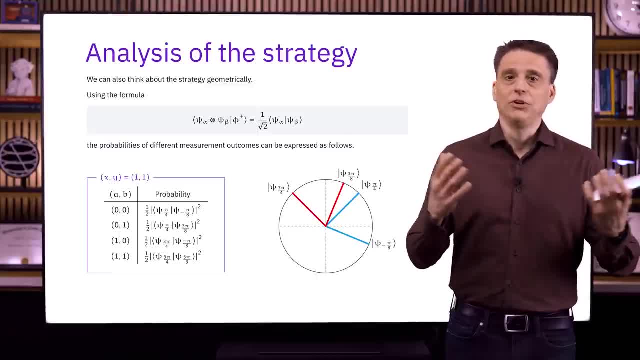 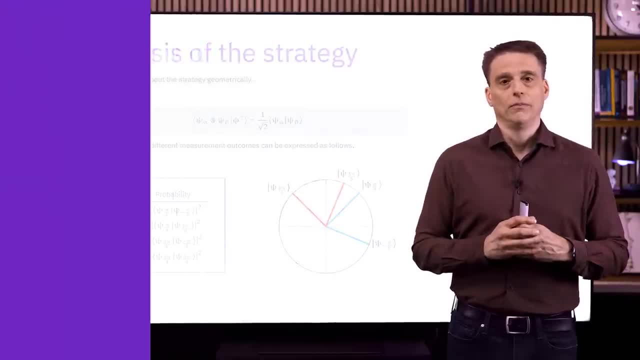 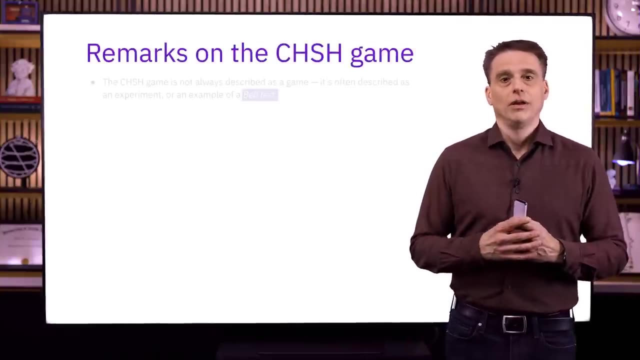 And perhaps this geometric picture is helpful in building some intuition for how this strategy works And why these various angles were chosen in the way that they were. To finish off the lesson, I'll make a few brief remarks about the CHSH game. First, as I've already mentioned, 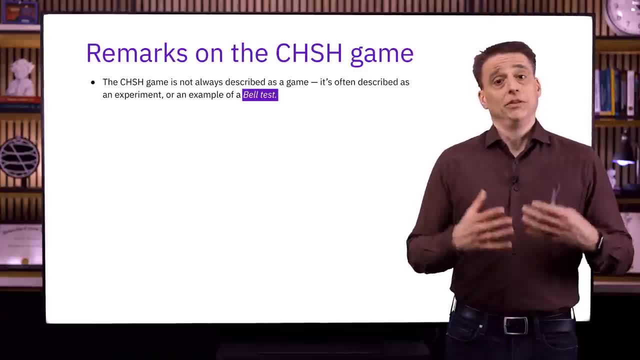 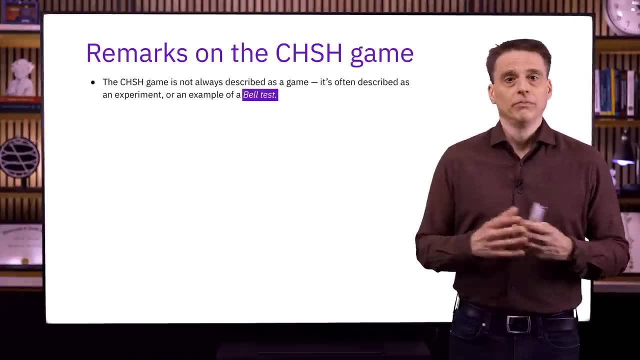 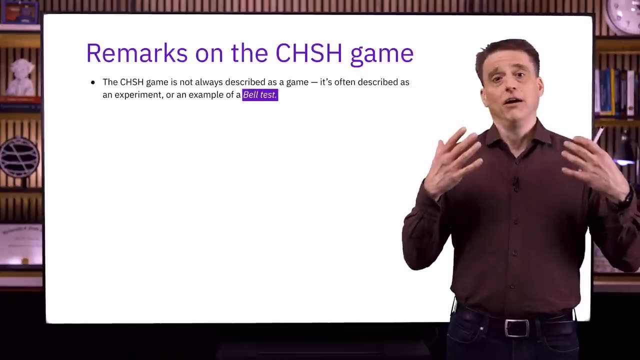 this example isn't always described as a game. In the physics community, for instance, it's more common that the example is described simply as an experiment rather than a game, And Alice and Bob are viewed as being detectors rather than players. The basic idea of an experiment like this. 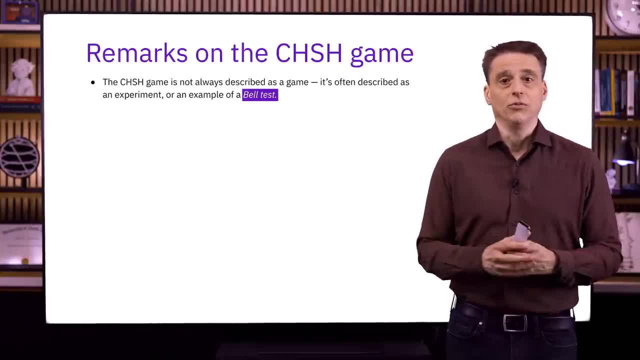 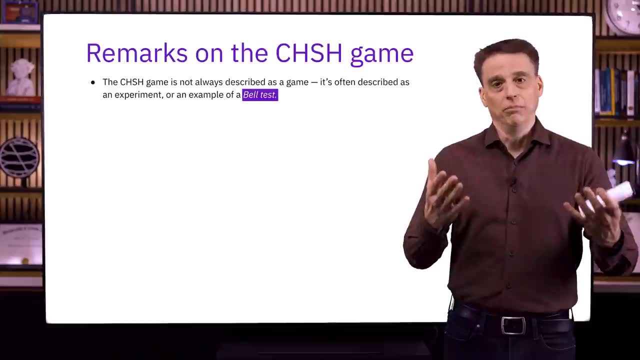 where entanglement leads to statistical results that are inconsistent with any classical description or, more generally, any theory based on so-called local hidden variables is due to John Bell, the namesake of the Bell states, And so people often refer to experiments of this sort. 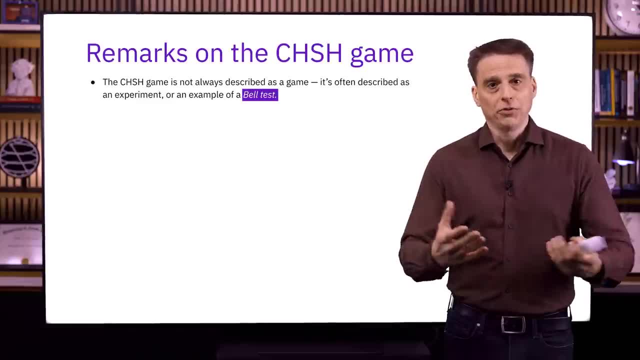 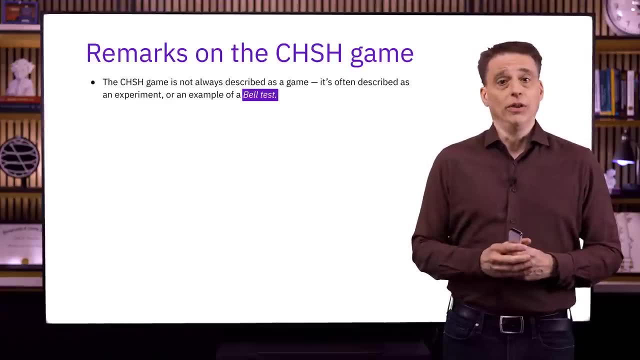 as Bell tests. Sometimes people also refer to Bell's theorem, which can be formulated in different ways, But it basically says that quantum mechanics is not going to work. But it basically says that quantum mechanics is not going to work. It is not compatible with so-called local, hidden variable theories. 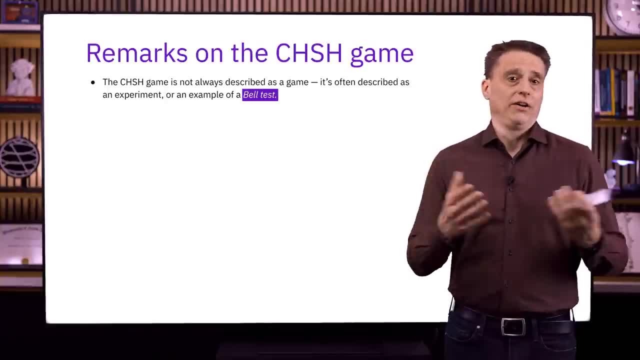 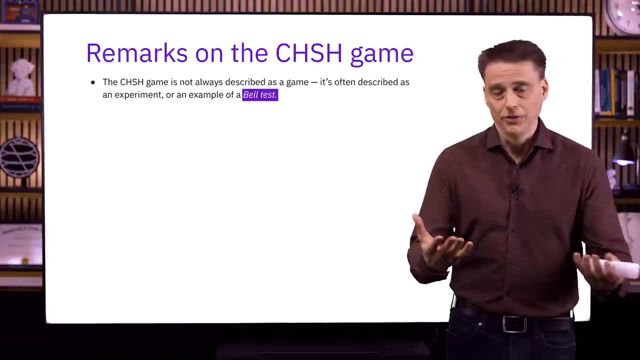 The CHSH game, or inequality, is essentially a very nice and clean example of a Bell test, And you can think about this example as a proof or a demonstration of Bell's theorem. The second remark is that the CHSH game offers us one way. 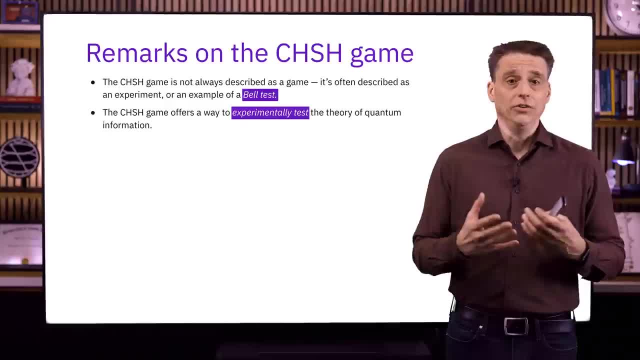 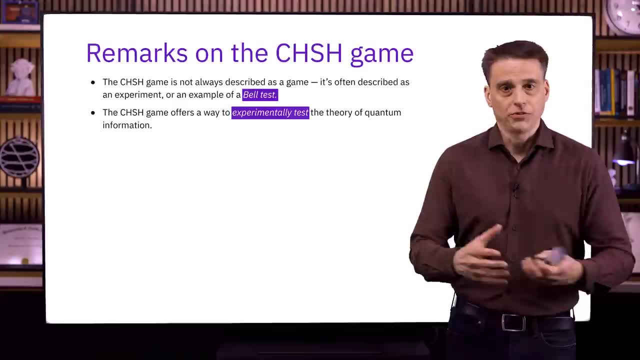 to experimentally test that the theory of quantum information is an accurate theory. We can actually set up experiments that implement the CHSH game, including the sort of strategy based on entanglement that I just described, and see if it works, And it does. 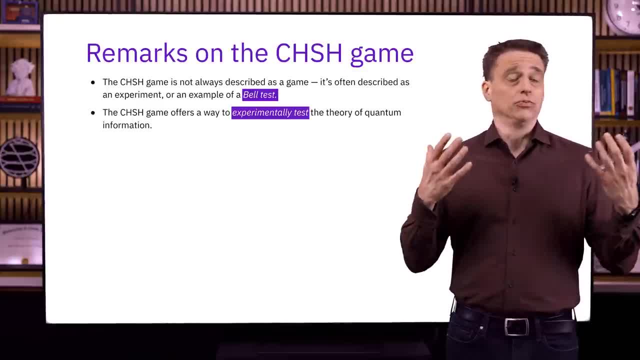 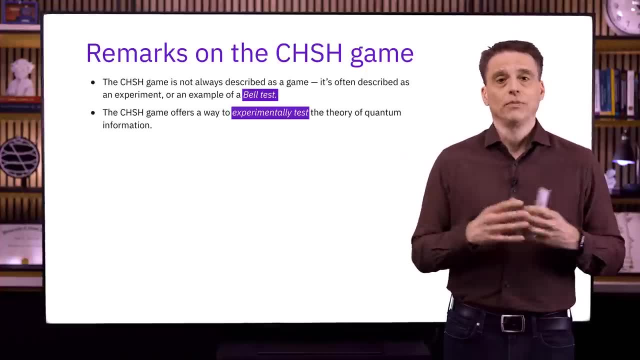 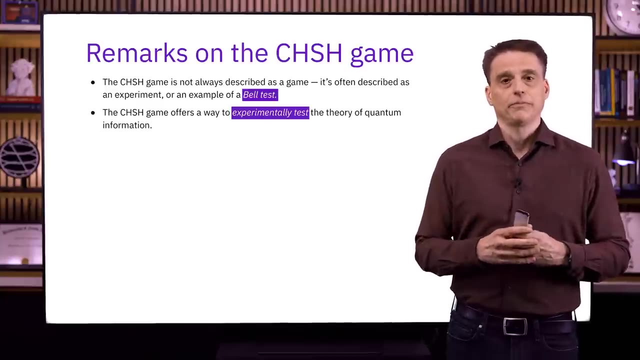 This provides us with a high degree of confidence that entanglement is real And, unlike the perhaps vague or poetic ways that we try to come up with to explain entanglement, the CHSH game or experiment gives us a concrete and testable way to observe entanglement.